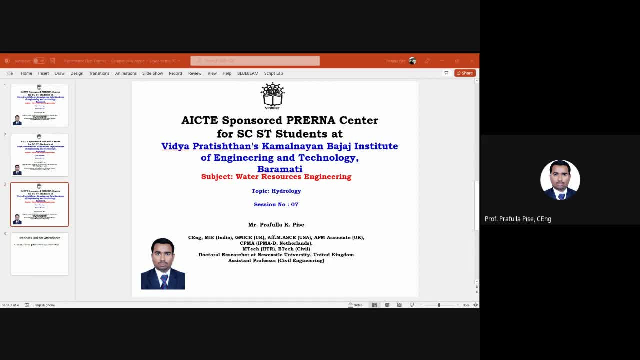 by Professor, Prof Pise. So today we will discuss about the hydrology which is a topic under water resource engineering. There will be like three topics we will see, you will see, under the water resource engineering. First is hydrology. second is irrigation engineering. 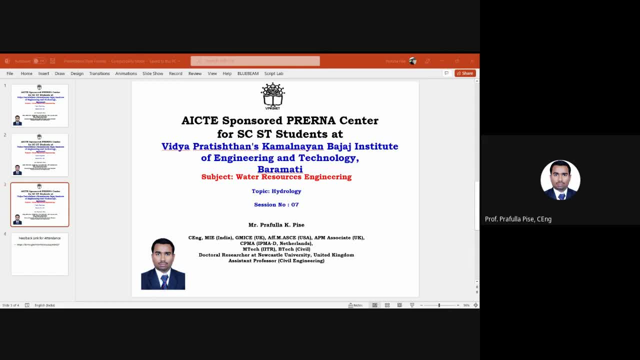 and third is the dams: okay, which was called as a water resource engineering tool- Okay. third, we have already covered some of the theory part about hydrology. We also covered the syllabus for water resource engineering for GET 2022.. Now today we will try to study. 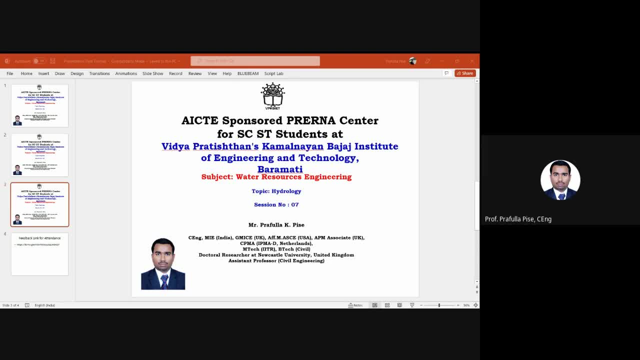 the hydrology. So we will start with hydrology. So we will start with hydrology. So we will start with hydrology. Okay, And then also we will try to know some advanced topics in hydrology And also, if time formats. 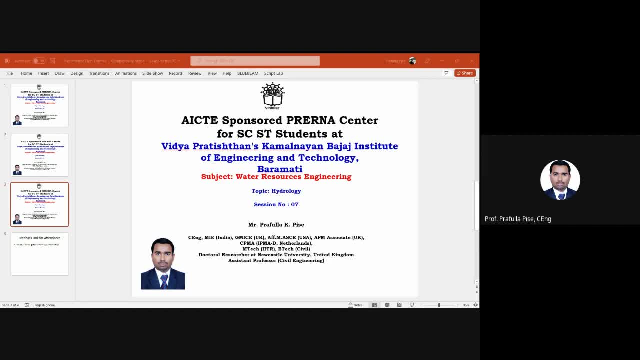 we will try to do some exercises. okay, some problems. So I will give you some questions and I will ask you to solve those. But if you can't, then don't worry about it. I also of those uh problems. okay, now you will see there are a lot of uh questions in hydrology. they are totally uh. 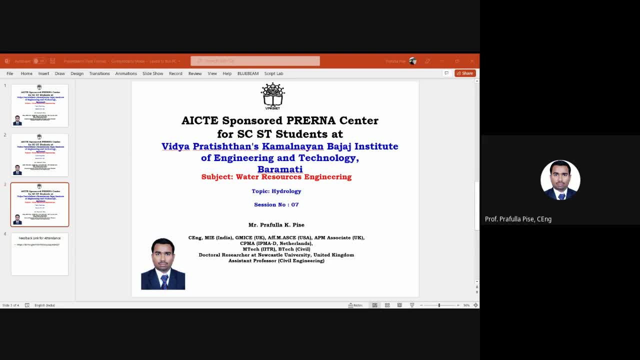 theoretical based. okay, so it's going to be a little bit difficult to remember each and everything. okay, so that's only uh possible if, if you can uh practice it now. to practice, you have to understand. please don't go over last three or five years uh get paper, because usually in uh gate the last five years questions the last five yearsrok. 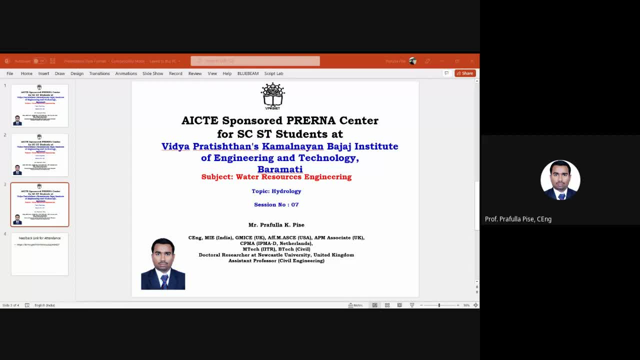 don't uh reappear, okay. there is always chance of one or two questions, you know, appearing repeating themselves, but it's highly unlikely, is even equation. take paper, question paper and and now new questions. okay, theoretical question, definitely theoretical. they don't have any new theoretical question, okay, and they don't have a new uh. 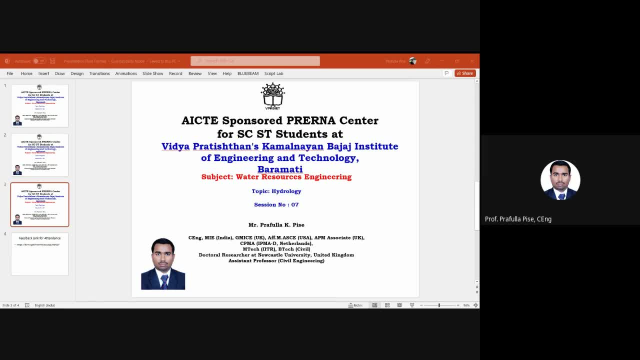 theoretical question: uh number is a repeat. uh, uh, uh, uh, uh, um, what do you mean? what? yes, yes, yes, any sigma one, V and seven, eight, because they're going to call it j. You have to solely focus on practicing exam paper. Give mock test For mock test. I have shared some links in my whatsapp group. 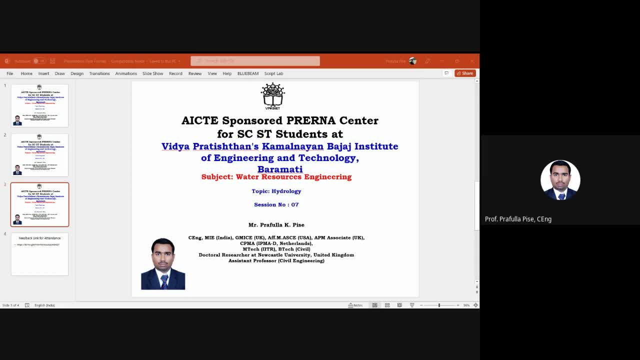 There is a test book. It costs around 15-20 rupees per month. It is not that expensive. What is the subscription? If the subscription is free, why can't you get it? If you want to upgrade, like in Udemy, you can upgrade. 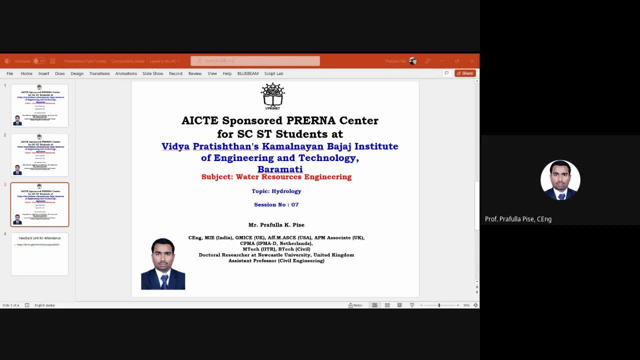 Why can't you get a subscription? It costs around 1 month. They have a lot of mock test available, Not only the entire syllabus, but they have mock exam with respect to topic wise, Because topic wise there is an exam. 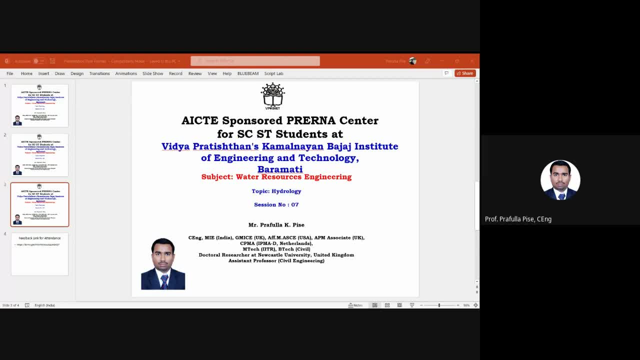 You can give an exam based on the topic, For example, general aptitude, mathematics mock test. You can give that. Or you can give an exam based on the topics in CVG And it is not that expensive. It costs around 100-1500 rupees per month. 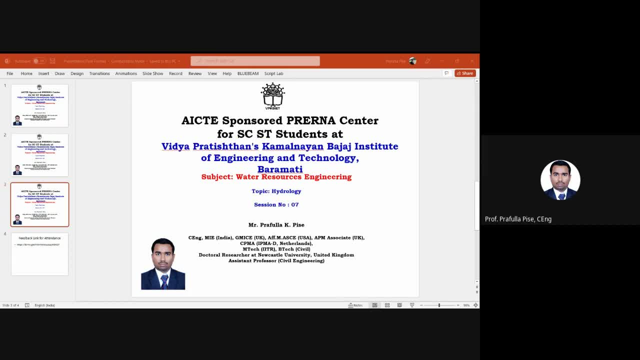 You can give that. What else can you do Online web: They have a website. You can give through their website. They have an app. You can give through the app, But for 1 month, if you focus, you can only give mock test. 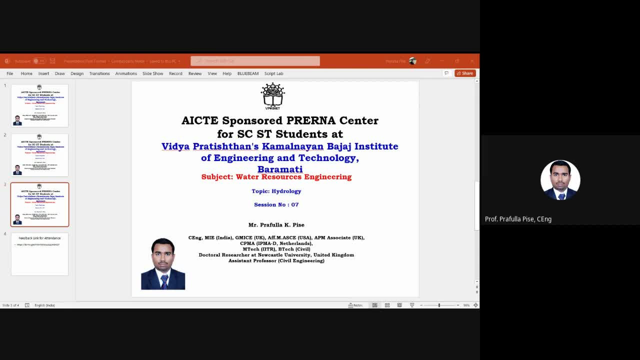 Now is the time to study or learn anything new. You can't learn anything new, Just give a test paper. The second thing is you give mock test. But what do most people do? They give a test And say, sir, give me 20 marks in mock test. 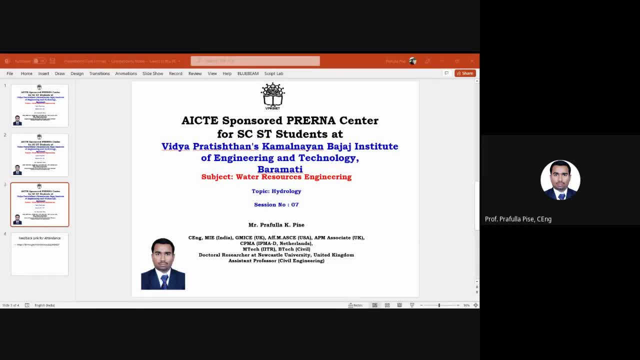 I am talking about topic wise. You get it: General aptitude and mathematics. They have mock test For that topic. you give 20 questions, Give 20 mark test paper And they give 1 hour. It is 60 minutes. 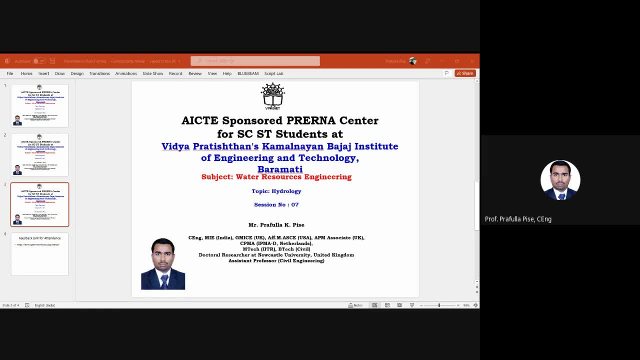 Or 20 questions. So 20 questions you can give 30-32 marks. for 20 questions they will have 30 to 32 marks and they will give you 60 minute time. why? what is the reason? yes, sir, okay, okay, right answer. 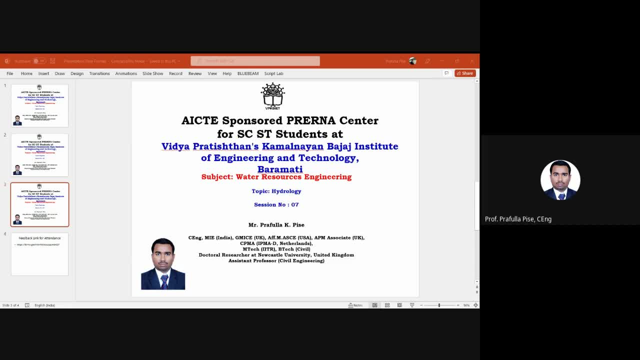 upon wrong color. why? uh, our logic was not worked out. okay, you have to find that out. media logic question answer: um, okay, and then you have to learn. and when i say learn okay, okay is not right now, it is not about your knowledge. okay, you already have knowledge, you already have studied everything. 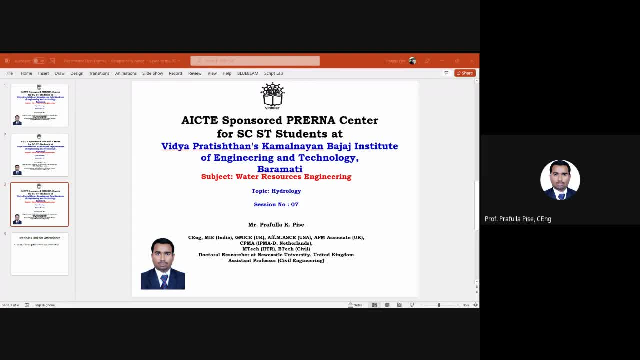 and right now you have to focus on how to crack the gate exam. the cracker example. how do you mean you have to know how to crack the gate exam. the main concern is this: In the paper there are questions and tricks. questions are simple and normal, but most 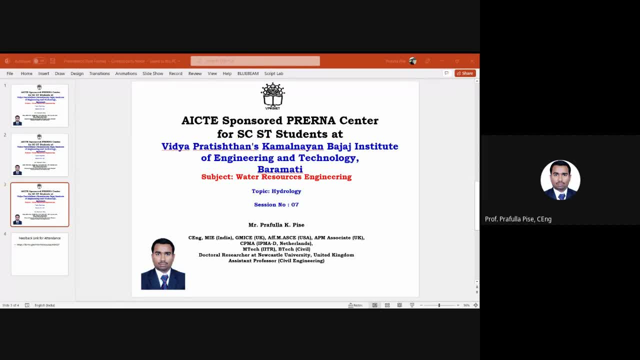 of the times they are not. there is always a trick in the exam paper. there is always a trick. So in the mock test paper you have to learn all the tricks and you have to learn all the tricks. Okay. 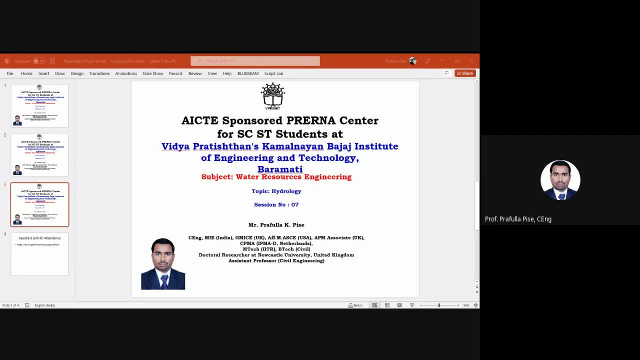 Now, if you have been here for a long time, there is a normal trick: we use it all. we use it at the maximum method of elimination. okay, now we have four options in the gate. the question is: you know that there are two options in the gate? they are totally wrong. 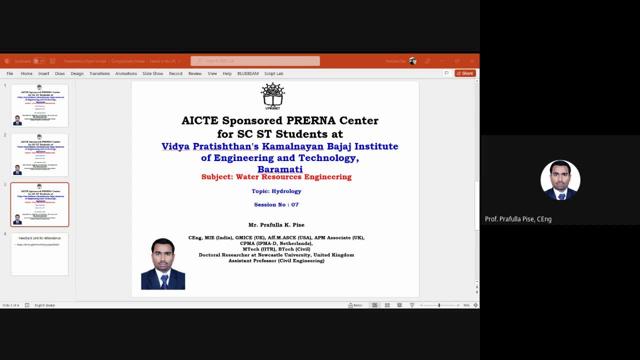 we do this. So I start with these two options and I complete them. Both the options fly away. both the options fly away. okay, they are so close to the right answer. Okay, Now we have to do something out of logic and choose the correct answer. 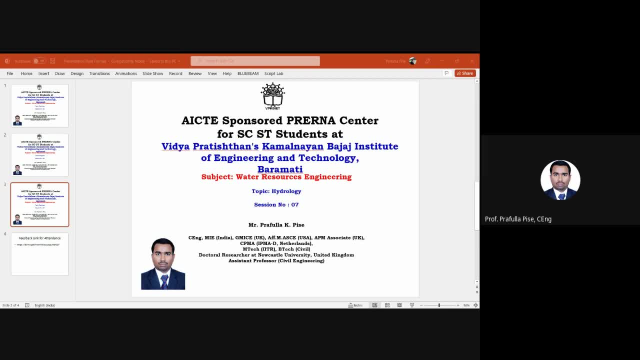 So this is only one trick, or this is only one logical trick, The only thing we do to get our right or correct answer. But there are a lot of things. okay, there are a lot of tricks in gate examination, which. 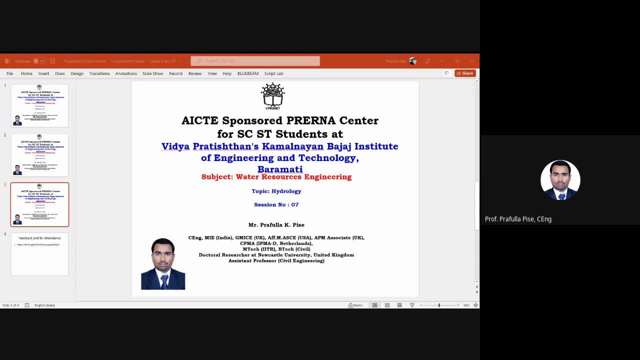 are called test papers. by solving as many as mock tests, okay. or the previous year's test papers, get test. You know, sometimes we have these types of wording. what can be the answer? What can be? there are our options: all of the above, none of the above, both A and B. 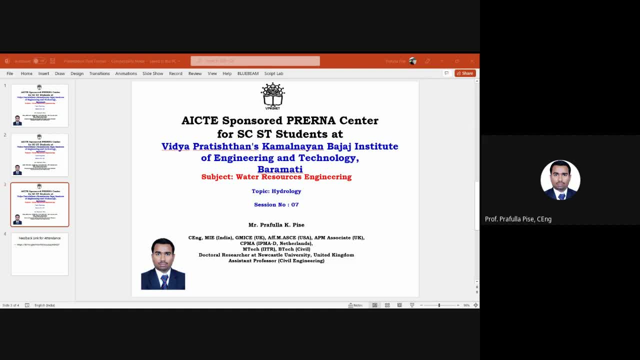 that's our question. Am I speaking correct? What am I saying? Okay, So you know, we have to do one thing, we have to do a test, We have to know the answer. Yes, Harshvardhan Mayuri, do you understand what I am saying? 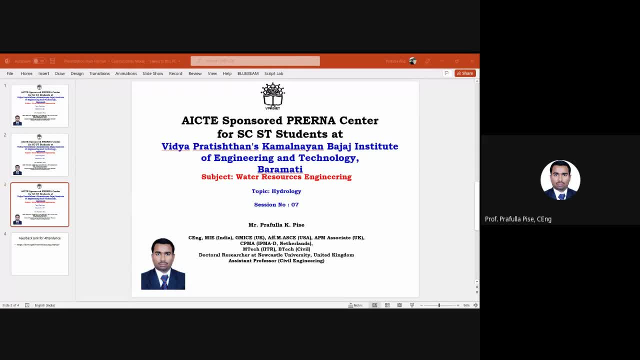 Yes, I can understand what you are saying. What was the trick? None of the above. all of the above, both A and B. What is the trick? What trick was it? What is the trick? What was the trick? What is the trick? 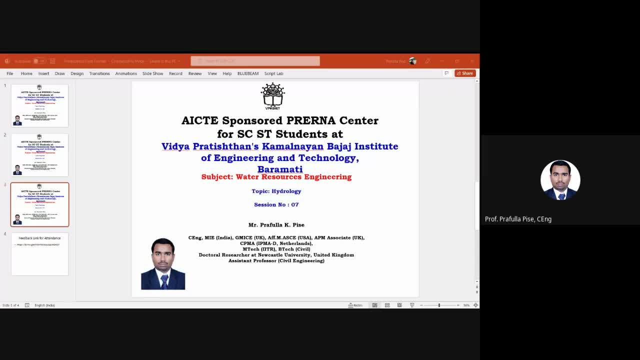 When you look at the question, you will know that if there is an option above, then the answer will not be given at all. But what do the maximum students do? They correct the answer above. So you can see that if there is an option above, then the answer will not be given at all. 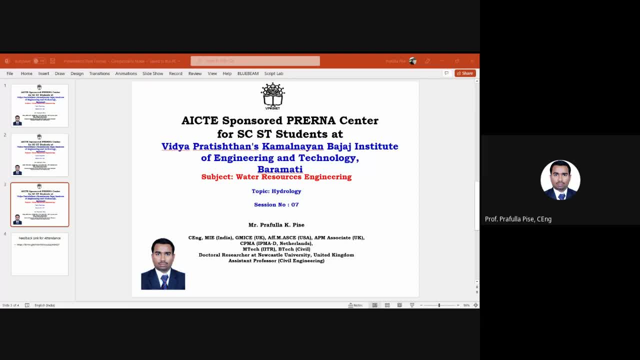 But if there is an option above, then the answer will be given at all. Or if there is an option above, then the answer will be given at both A and B. These are called hat tricks. Let me explain. These are called hat tricks. 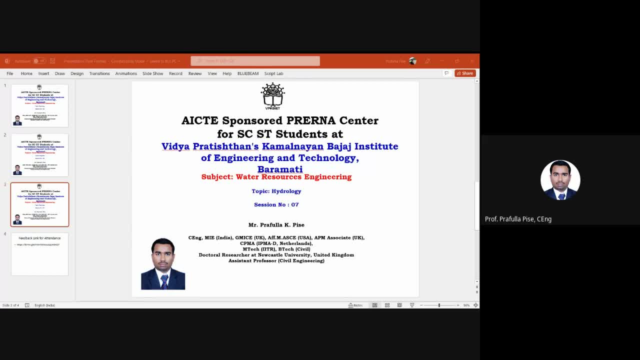 These are called hat tricks And you won't find these tricks. How do you find these tricks Where you solve the maximum question And you don't have to solve it After solving it? you have to check what is the answer in this question. 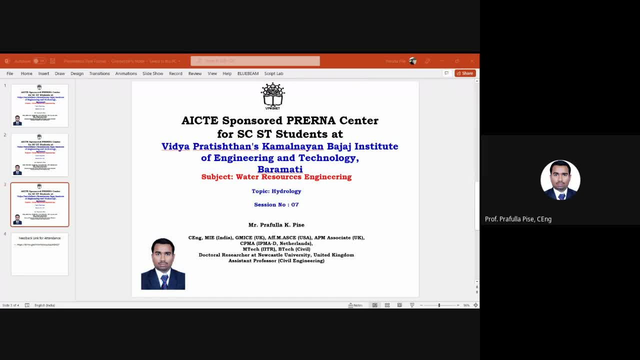 And what is the answer? And how did it come? You already know the answer. You already know the answer. I have done little revision, I have read it, So I know what is the answer. You can see what is the answer. 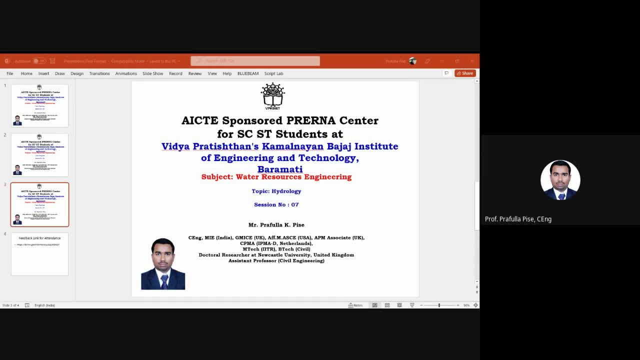 You will get the logic out of the box. Civil engineering is not a point of view. You have to use a little logic and commons to find the answers, And that is the skill of gates. How do the students and students focus? I mean, we are going to solve each and every question. it is not possible at all. 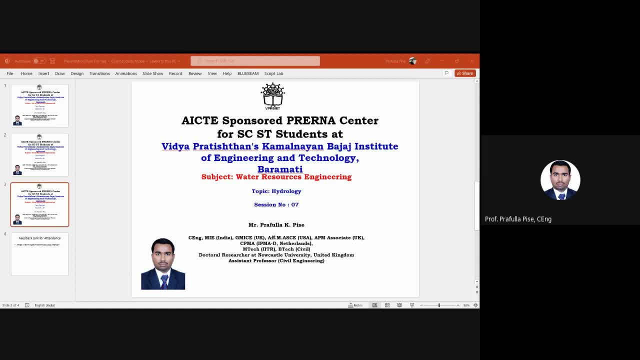 yes, sir, they have scored 100 percent. they are not expecting you to get hundred percent marks, why? because they are not expecting you to solve each and every question. okay, what is the full form of gate? the full form of gate is graduate aptitude test for engineering. 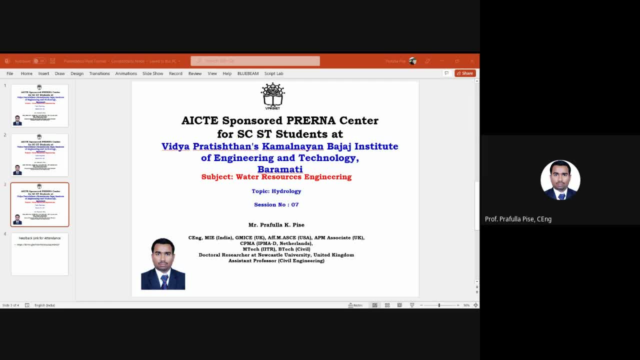 aptitude test as an engineer from the thinking of say him, but most of the questions will be there which you have to understand. use your common sense or logic and find out the answer. okay, when you are doing subject to type question, yes, that means you are really checking your knowledge. 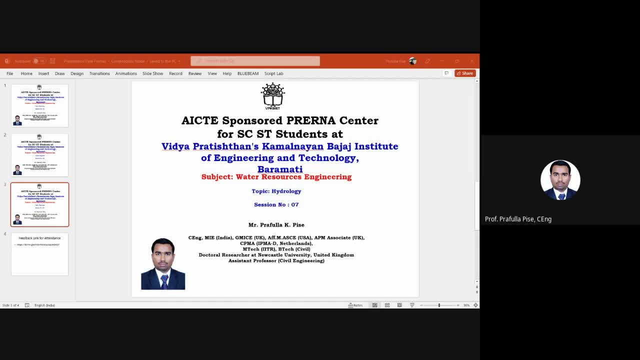 but when you are doing object to type question, it is all about your aptitude. okay, as an engineer, you have to develop your logic, you have to develop your skill, okay, so don't try to solve every question or your answer will not be like that by solving every question. 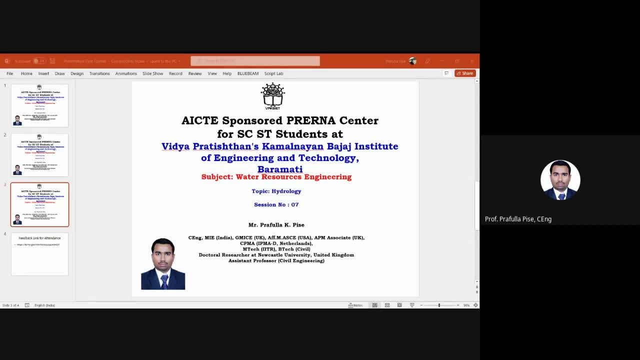 you have to use your logic, and that logic can only be developed okay when you start thinking out of the box. when i say out of the box, which means what other people do, how many students are there in the gate? how many students are there in the gate? 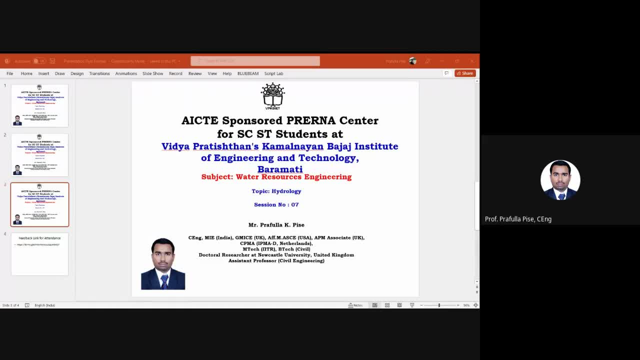 how many students are there in the gate? do you have any idea how many students are there in the gate? まん mycket meni Owari. I don't know, sir, how many students are there in the gate in each sector. do you have any idea how many students are there in the gate in each sector? 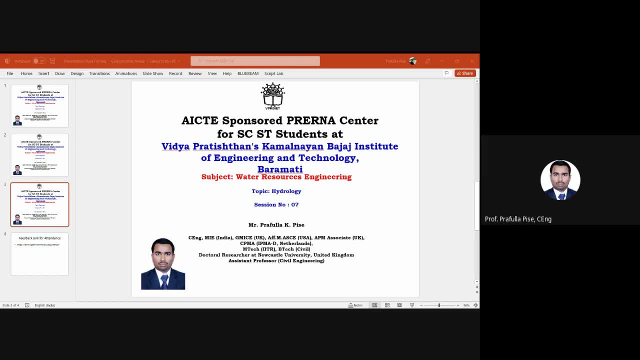 two teams in the gate In Maharashtra In this India, On Maharashtra, On Maharashtra. Now, as we have seen, in Maharashtra alone around 2 lakh children are born in the gate, And in the whole of India 9-10 lakh children are born. 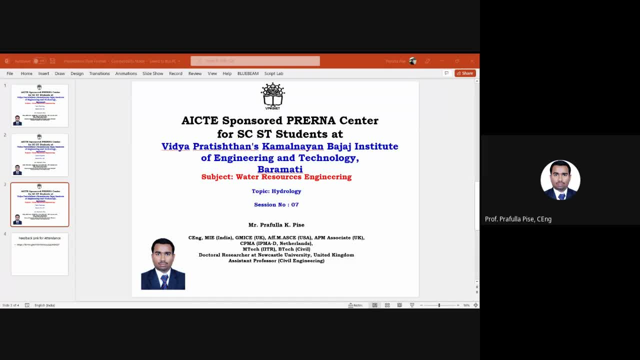 Before it was less, but now it is going higher and higher. And how many percent of children pass, How many percent of children are qualified So in the gate? if 10 lakh children sit in the gate, that means 1.5 lakh children, 15% children. they are qualified as a gate qualifier. 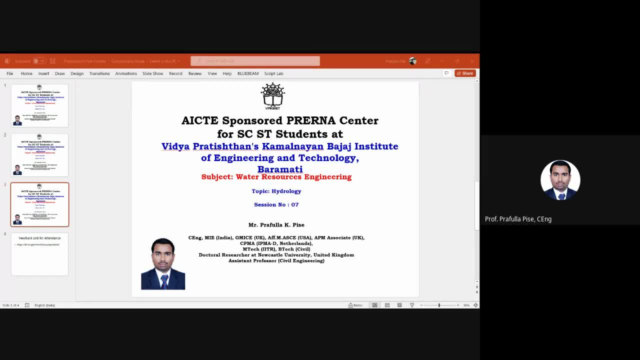 And that 15% children- only 1.5-2% children- pass IIT. So if there are 10 lakh children out of them, 10-15000 children pass IIT. Now IIT has increased a lot. That's why Earlier the number was less. In IIT the number of seats was less. Now IIT has increased. In IIT the number of master seats has increased. So 10 lakh children pass IIT every year. 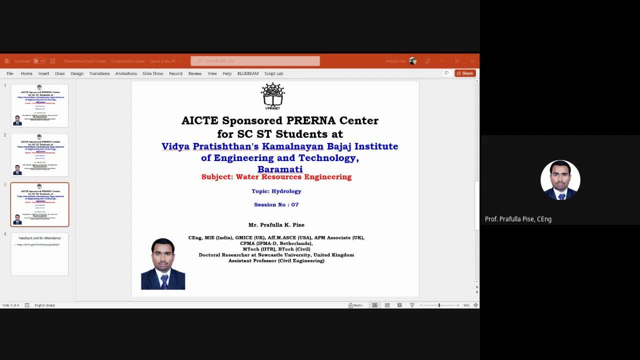 Approximately 1% And plus the rest have PSU. So they accept the score of the gate And it is not only for MTech or PG, They also use the gate score for PSD. There are many people who are masters who do PSD. 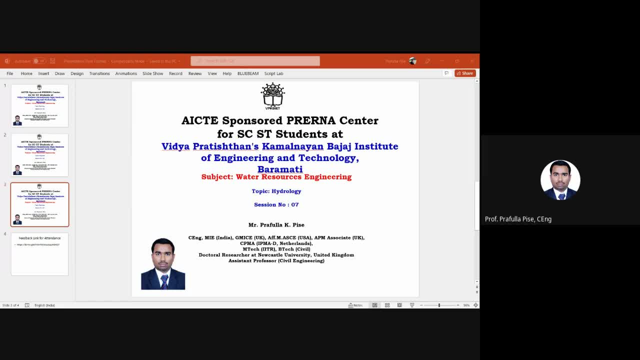 They also appear for the gate exam. So if there are 10 lakh children, we have to be unique, We have to be different than those. You will see the picture of 10 lakh children. How do we do 10 lakh people? 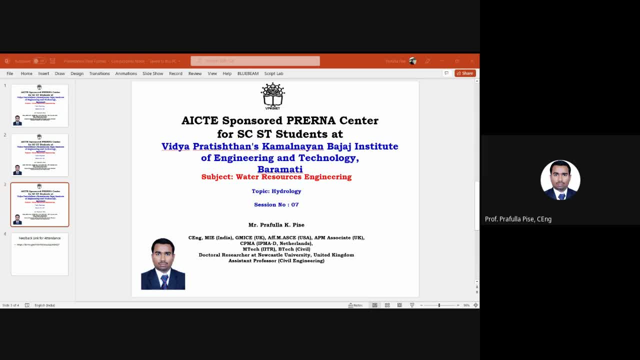 As you think, Each and every question we have to solve. OK, We solve every question. We have to get right answer for each and every question. We have to use the calculator and get done all the calculation. We have to remember all the formulas. 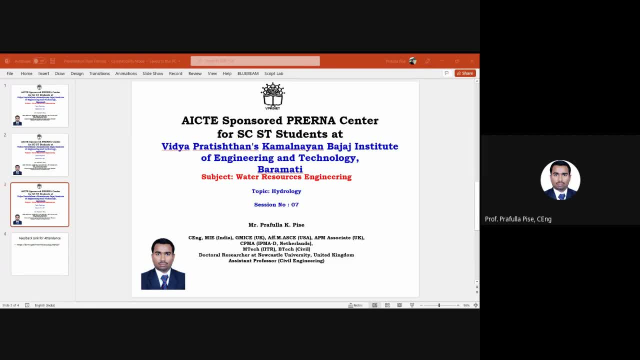 OK, But we have to remember all the theory. Everyone is thinking like this, And the exam paper set or the exam candidate, they also know this. So they are not looking for everyone. They are looking for some people who are different than everyone. 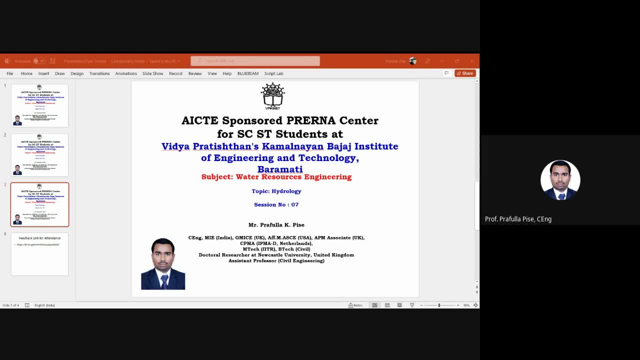 Keep this in mind. You have to be different. You have to think differently about what other people are thinking. Now this is done. Now I will tell you the second part about the gate. I had told you in the previous video. Now I will repeat it again. 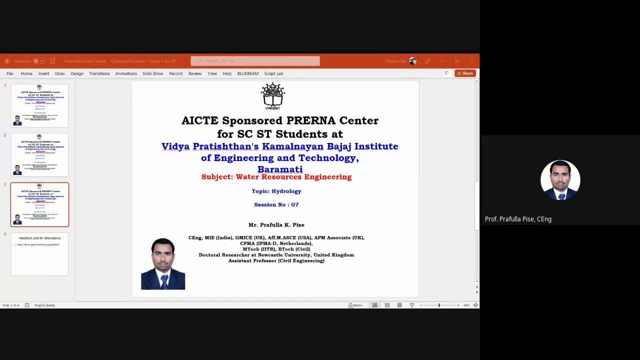 You should not have all the subjects in the gate. Your strong suit, You should focus on it. If your mathematics is strong, then focus on mathematics. If your structure is good, then focus on structure. If your water source is good, then focus on water source. 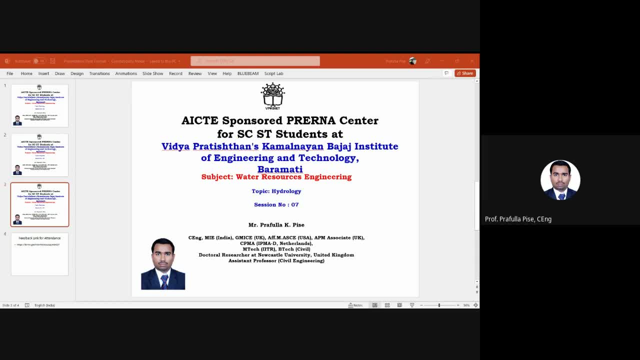 If your environment is good, then focus on environment. If your subject is good, then focus more on it. If your subject is weak, then don't talk much about it, Don't focus on it, Even Don't talk much about it. 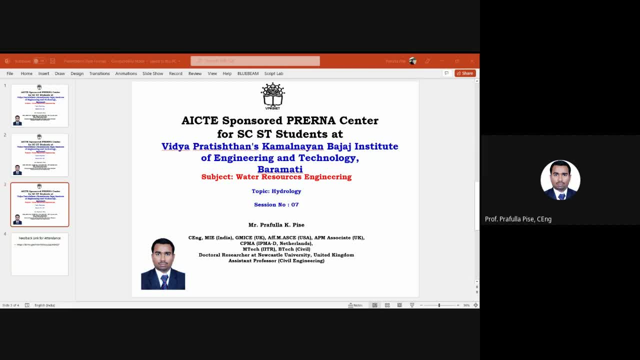 When we are going to take an exam. Remember There are going to be questions on each and every topic. Okay, If you miss some questions, it doesn't matter, Because if you miss a question it is better than getting a wrong answer. 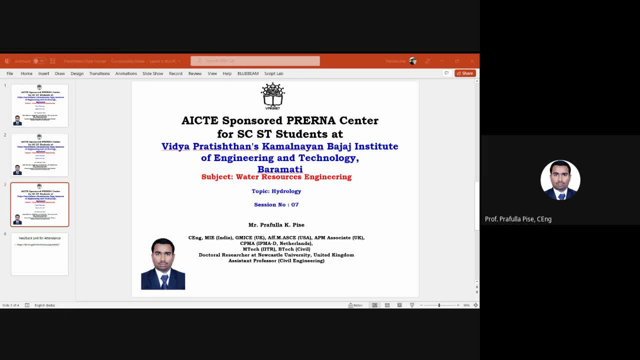 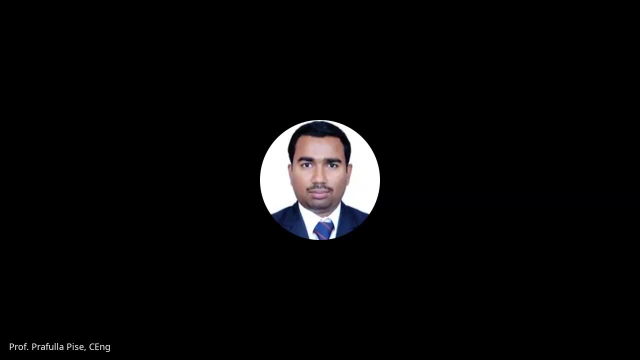 There is negative marking if you get a wrong answer, If you miss a question. there is no negative marking. Okay, Only solve the questions which you are comfortable with. Now, this is about gate. This is not a general idea. Now let's see hydrology. 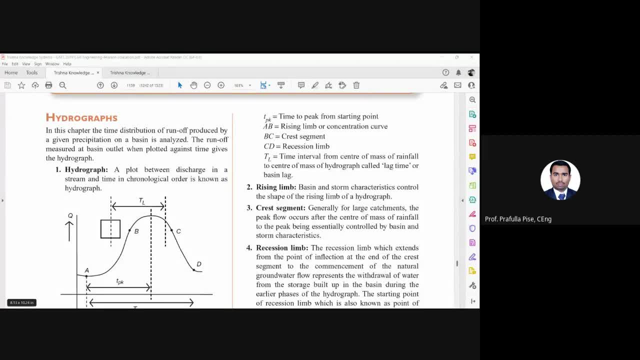 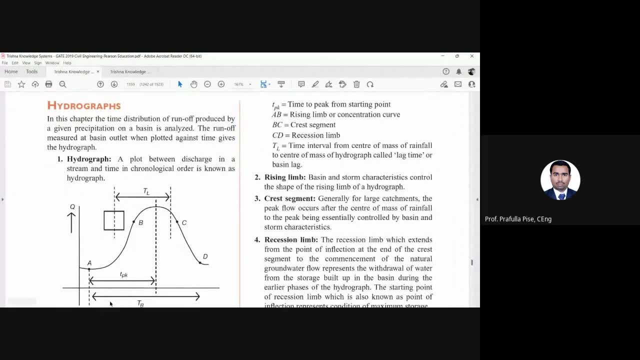 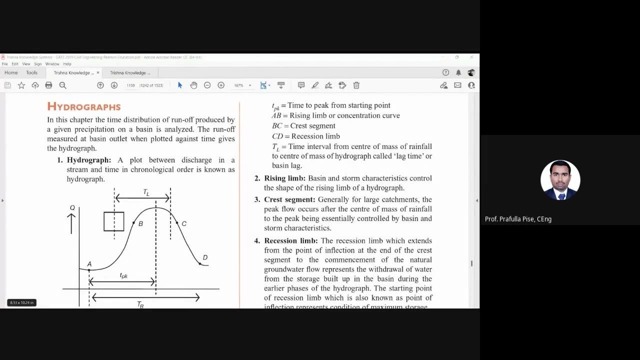 Okay, Any other question or something you want to ask? Any doubt about what I said? Any question about what I said? Any doubt about what I said? No, sir, No. Then let's start from the beginning. What did I say? 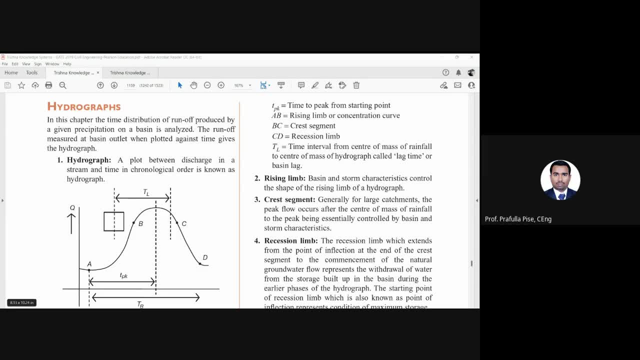 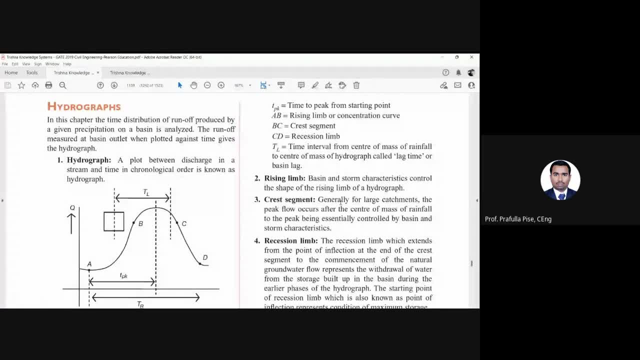 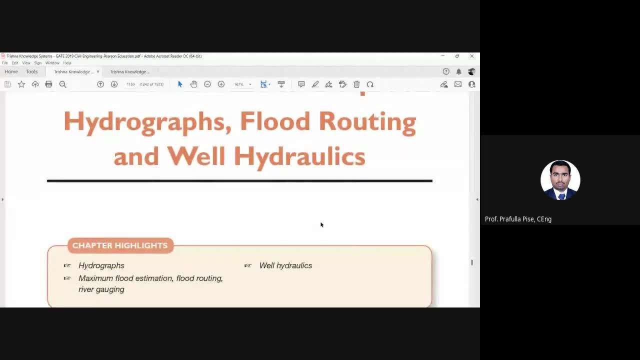 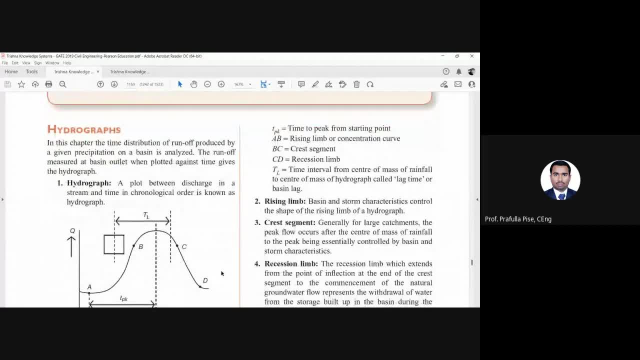 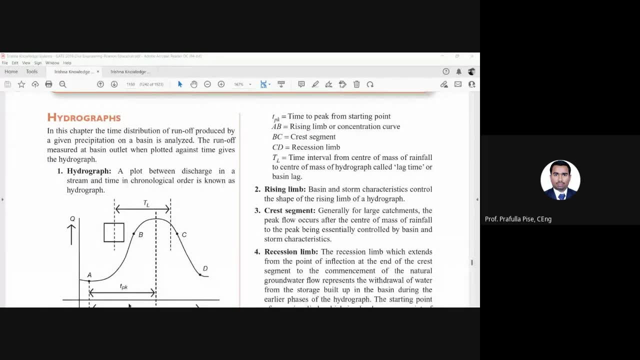 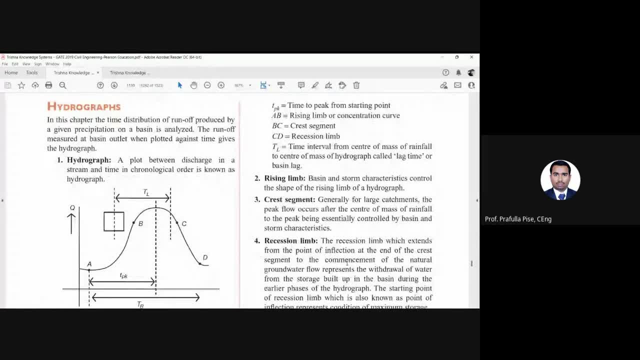 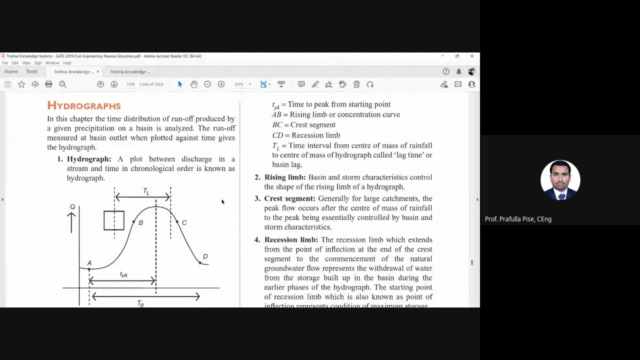 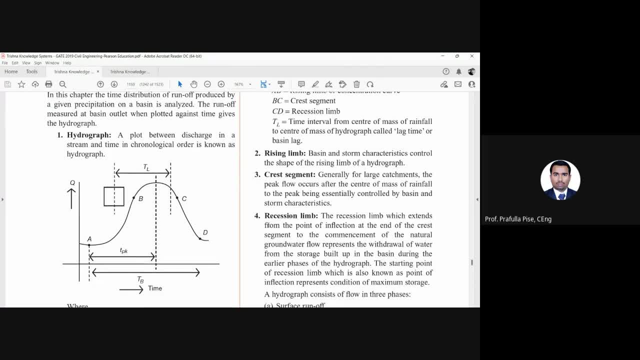 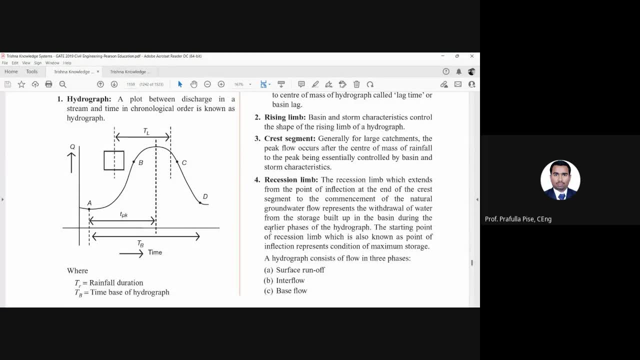 hydrographs. okay, so what is hydrograph? it is a plot between discharge in a stream and time in chronological order, which is known as a hydrograph. so discharge and time. okay, so we have time on x-axis and we have discharge on y-axis. okay, and the most important thing, 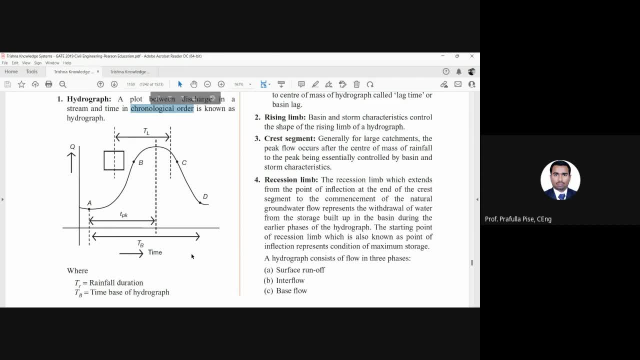 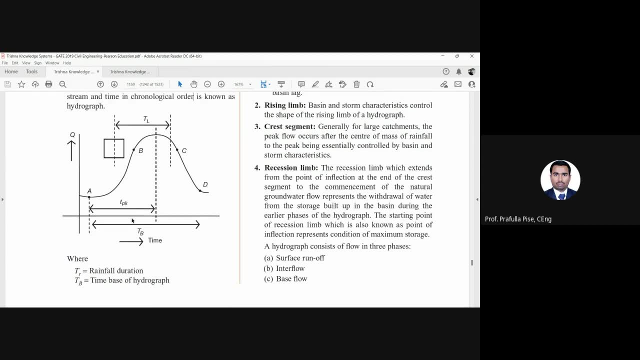 is. it is in chronological order. so these are the main important factors. we have to remember about the hydrograph. now, in the hydrograph this look like a bell curve, okay, or parabola, we can say it is like a bell shape, er, if you remember from your mathematics, it looks like: 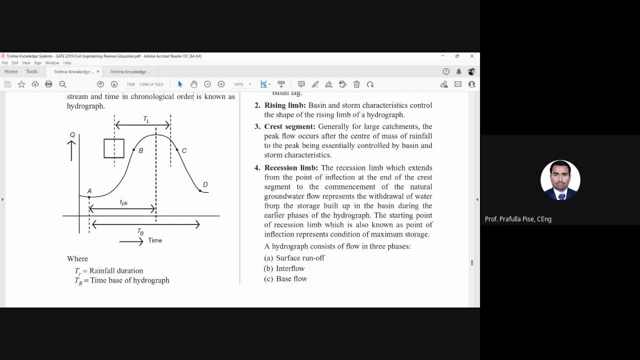 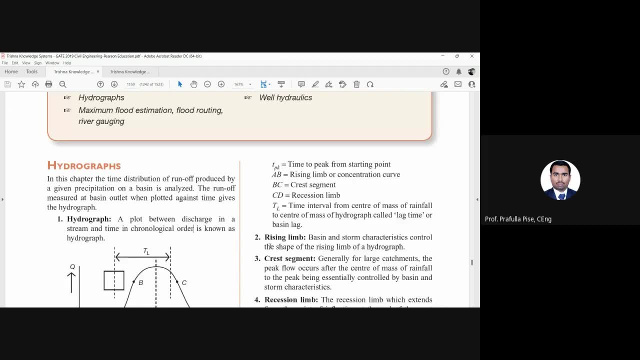 a bell shape. it is like a bell shape, okay, so be still and be witty to those little things. what is what is saying? strong point behind the confidence. we will move it back for more a normal distribution: okay. here we have point a, point b, point c, okay, and point d, okay. so what is? 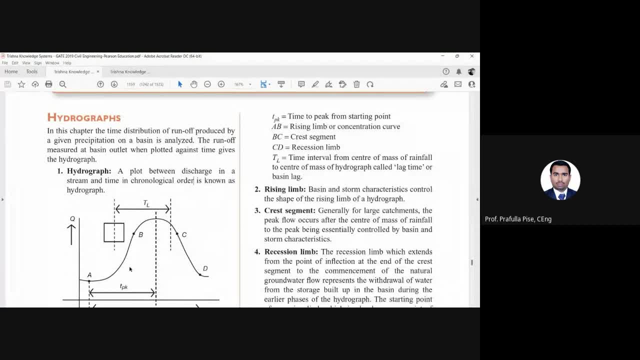 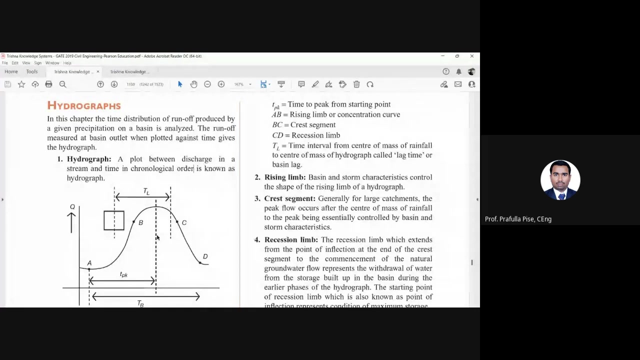 a to b. a to b is a rising limb, okay. or concentration curve. b to c is what we call as a crest segment and c to d is what we call as a recession limb, rising crest recession, okay. now we have t? l. what is t l? so time interval from center of mass of rainfall to center of mass of. 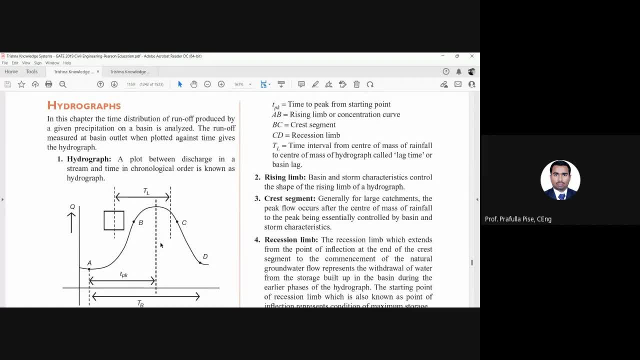 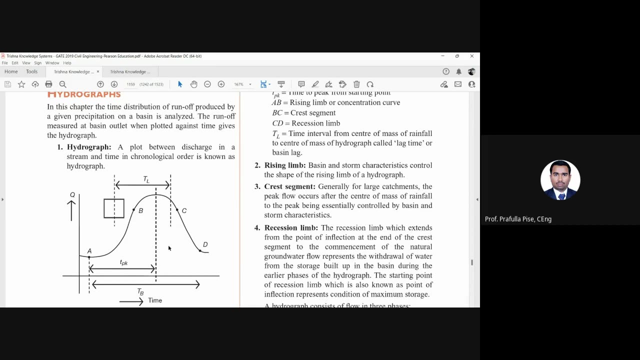 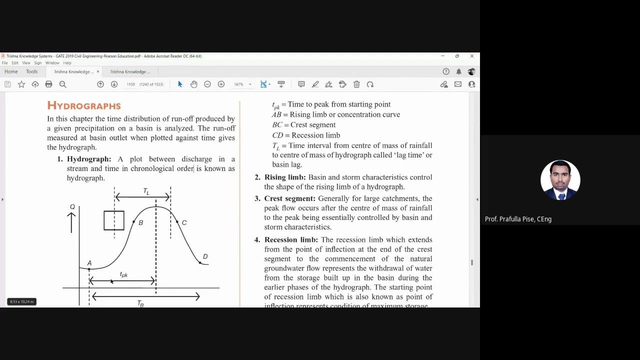 hydrograph. okay, it is called the lag time or basin lag. okay, so that's why t l lag time, t l lag time. okay, now there is another time which is we call as a t p k. p k means peak. okay, time to peak from starting point. so a was the starting point and here is the peak point. so time taken from: 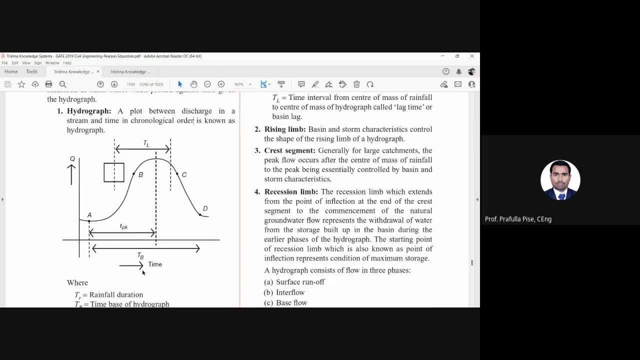 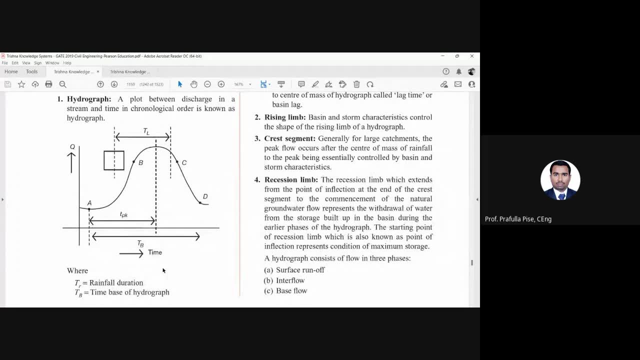 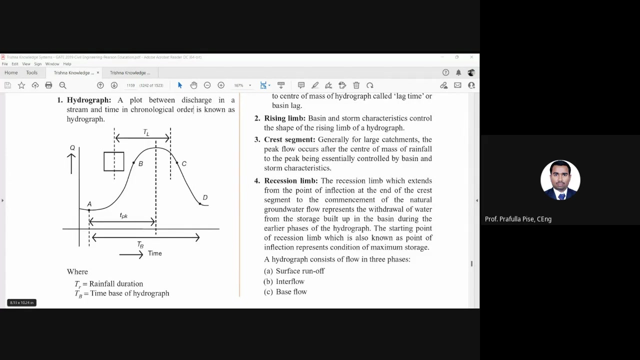 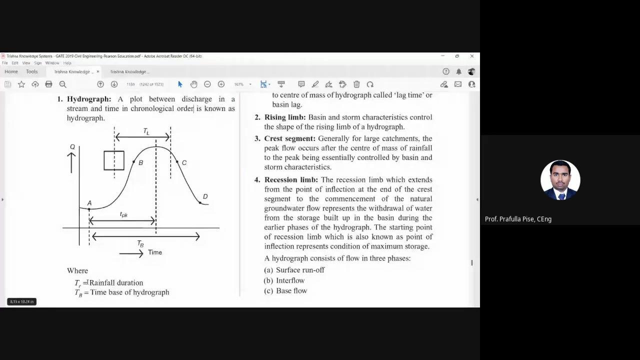 starting point to peak point is called as t p k. now we have t r, okay, which is also called as a rainfall duration, and t b is work as a time base of hydrograph. okay, now why it is necessary to understand this uh, hydrograph, because in the exam that is most important. okay, they might give you an hydrograph. 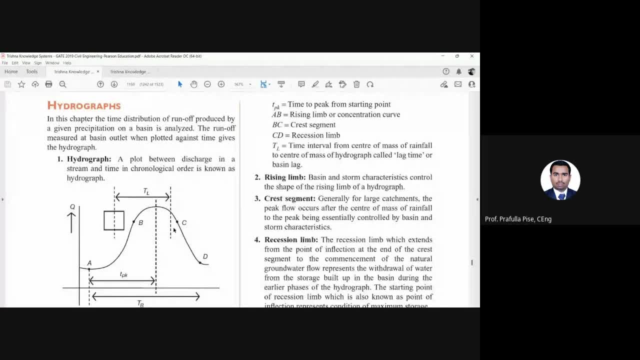 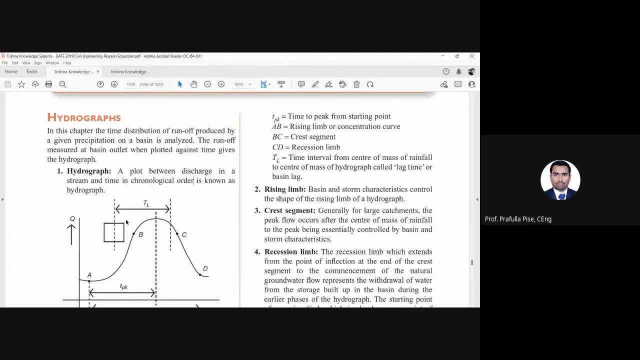 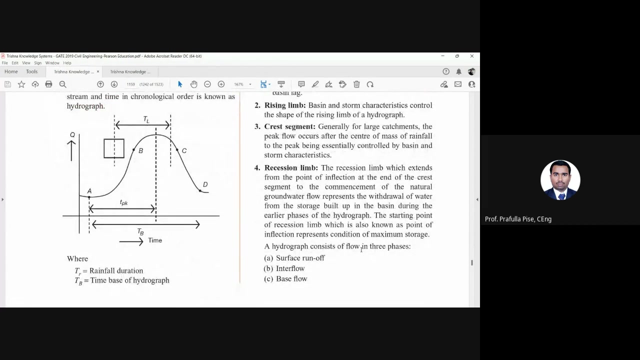 and they will ask you to find this, find that okay, or they will might give you the table, okay, with discharge and time okay, and they will ask you something okay about any of this term, okay. so you have to understand those terms. now, what is rising limb? so basin and storm characteristics control the shape of rising limb of hydrograph. 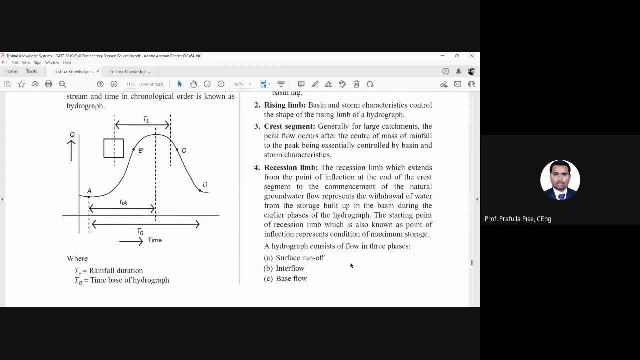 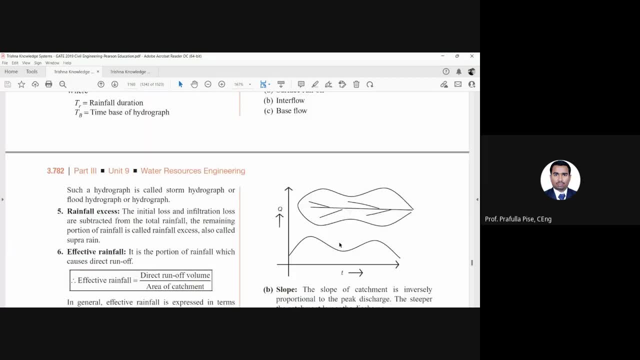 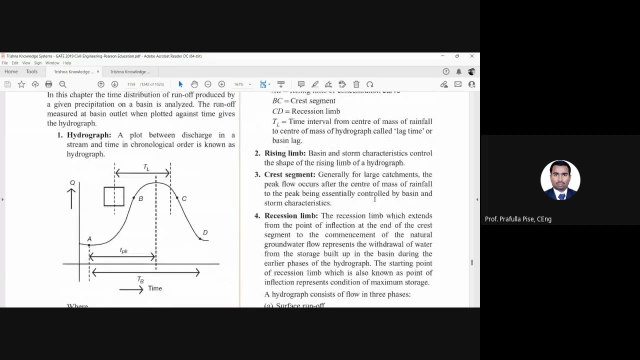 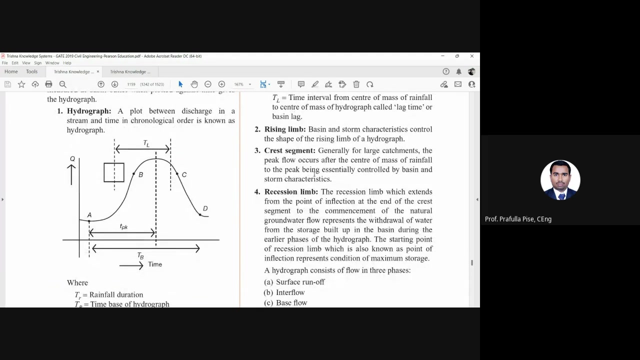 okay, so this is something you have to remember: basin and storm characteristics: basin means watershed, okay, so these are the watershed. okay, so those basically control the shape of rising limb crest segment is generally for large catchment. the peak flow occurs after the center of mass of rainfall to peak being essentially controlled by basin and storm characteristics. okay, so it is. 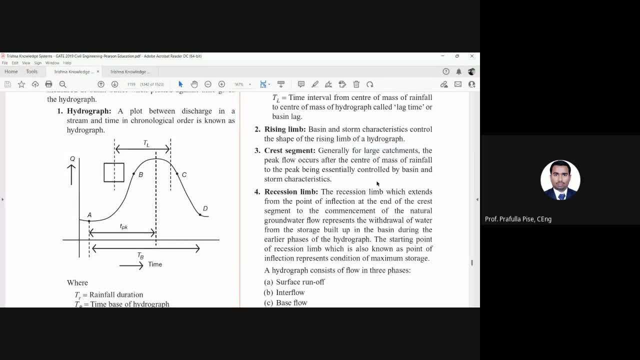 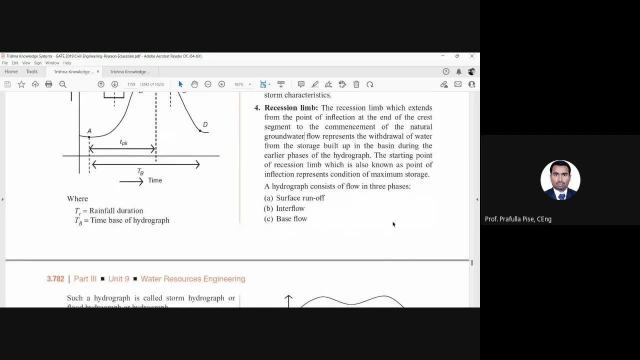 basically, for large catchment area it will be a larger crest. for small crash media the crest will be sharp. okay now recession limb. okay now recession limb system which extends from the point of inflection at the end of crash segment to the commencement of natural groundwater flow, representing the withdrawal of water from the storage. 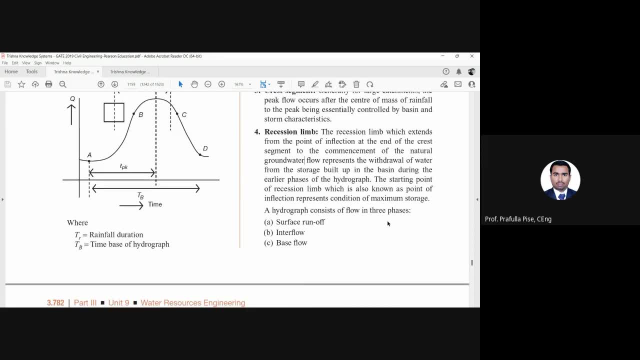 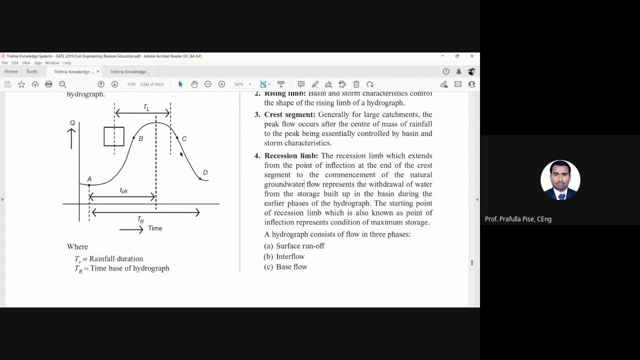 built up in basin during the early phase of hydrograph. so that's again you have to understand. for the recession limb, the groundwater or saturation or infiltration rate, these things plays much important role in the recession limb, the starting point of position limb, which is also known as the point of inflection. okay, so that's the point. 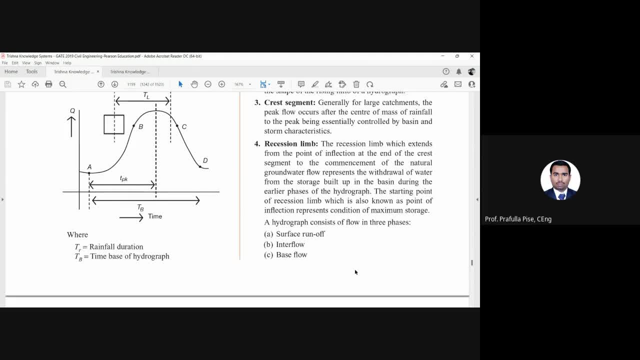 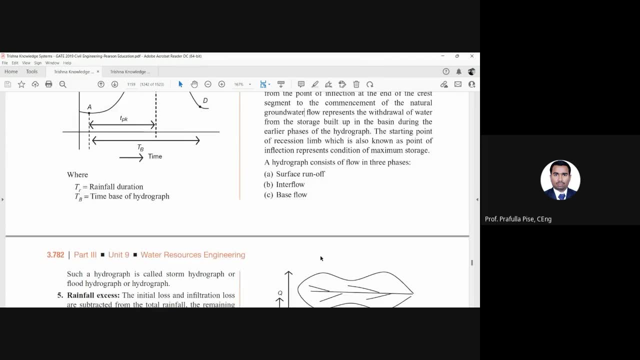 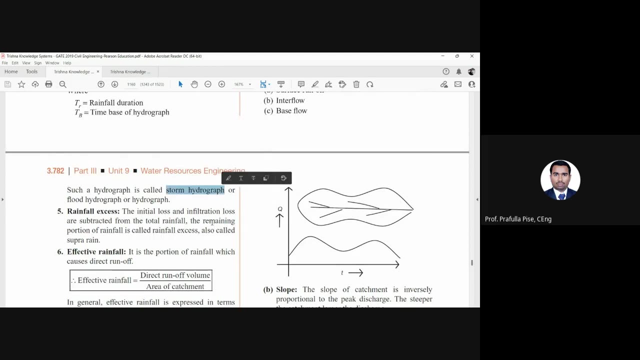 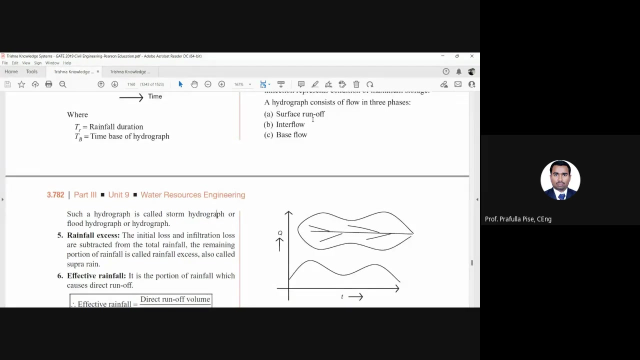 uh represents condition of maximum storage. a hydrograph consists of the following three phases: surface runoff, interflow and base flow, and this hydrographs called as a storm hydrograph, okay, or flood hydrograph. what is the storm hydrograph for photograph which has surface runoff, interflow and base flow? okay. 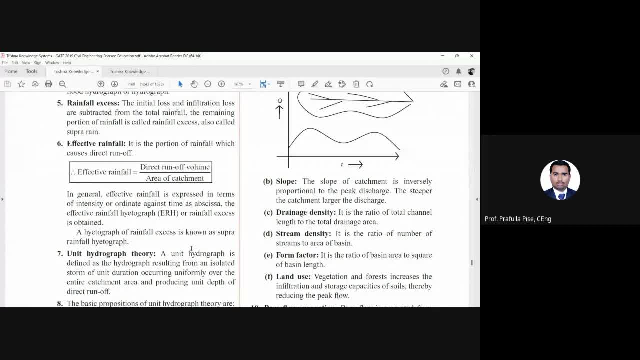 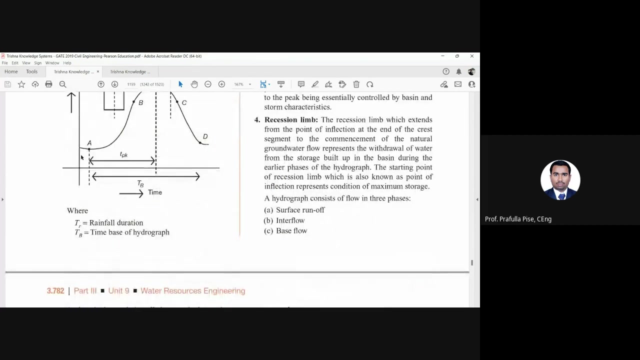 rainfall excess. the initial loss and infiltration loss are subtracted from the total rainfall. the remaining portion of rainfall is called rainfall excess, also called as a supra rain. okay, again, remember these terms: supra rain or then for excess. so you have to subtract the initial. okay, let's subtract the initial loss and inflation lot loss. 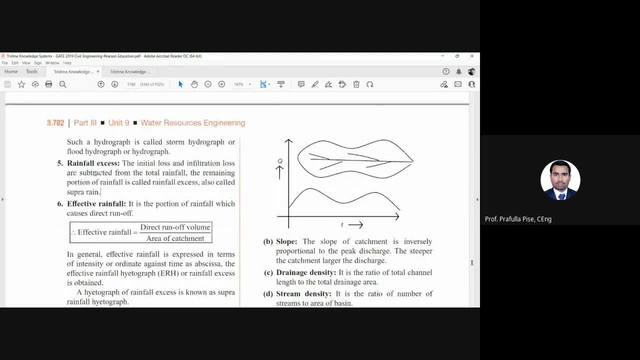 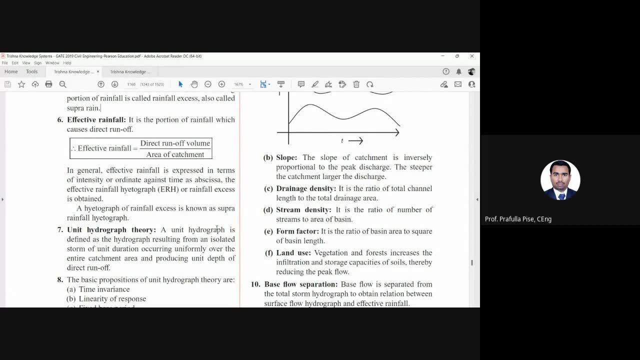 okay, from the total rainfall that is only going to give us the then for excess effective rainfall, it is the portion of rainfall which causes direct runoff. direct runoff means usually we have the surface runoff or ground runoff. effective rainfall equals to direct runoff volume over the area of catchment. okay, so basically volume. 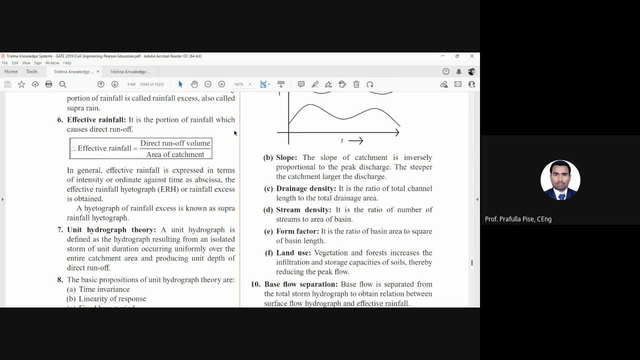 divided by area will give you a height. okay, that is basically in between inches or mm, centimeter. okay, it depends. nowadays we use mm, but uh, still now. uh, because of the british system, we use some, or sometimes we use inches, but uh, we are looking at the si system, so it is in mm. 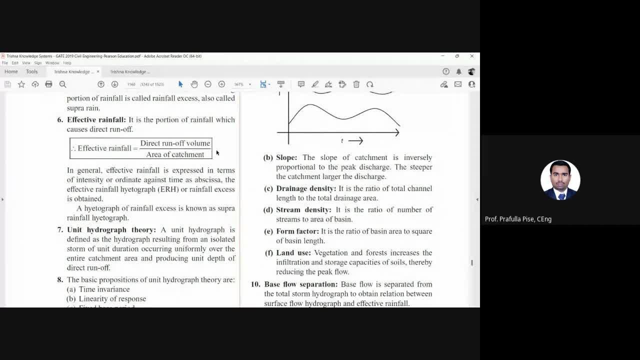 but in get exam they might ask you in inches or they might ask you in mm if they want to. you know, throw you out of your balance. so they might ask you in centimeter. so you have to focus mm, centimeter, inches. these are the things you have to remember. okay, these are the things you have to. 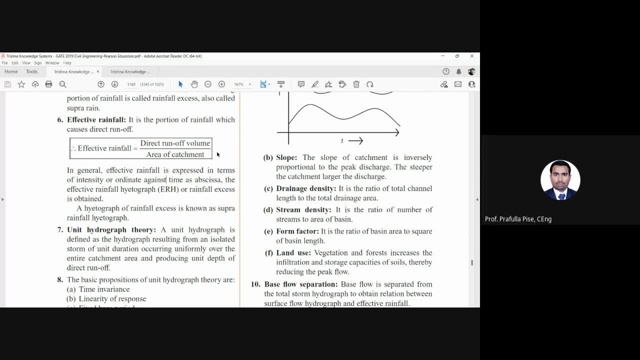 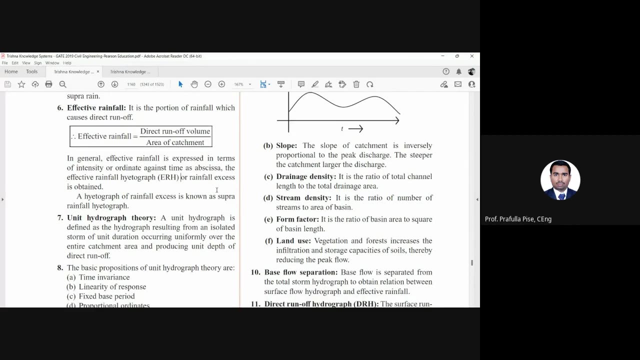 focus on. okay, these are the theoretical questions. okay, because a lot of problem in hydrology you will find is very time consuming. okay, there will be time consuming because it's mostly uh, consists of statistics and because of the statistics you have to go through a longer procedure on a time consuming procedure to find. 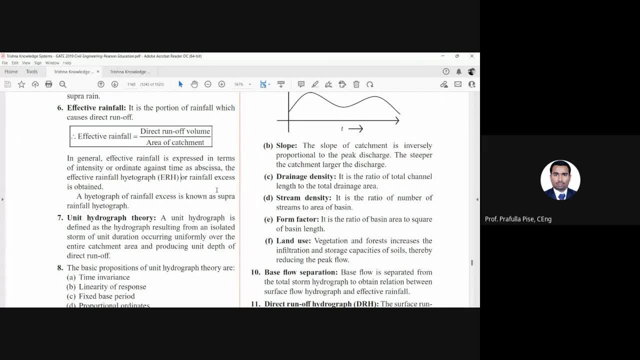 out the answer. so to avoid that, you have to understand, you have to remember these basic concepts. okay, so it's then for is nothing but volume over area? okay, so you can use that logic to get your answer. okay, so, direction of volume over area of catchment. 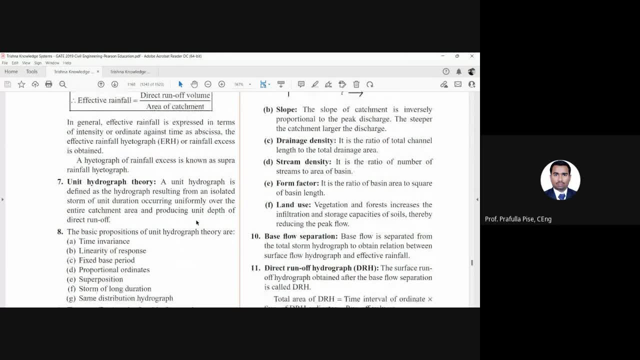 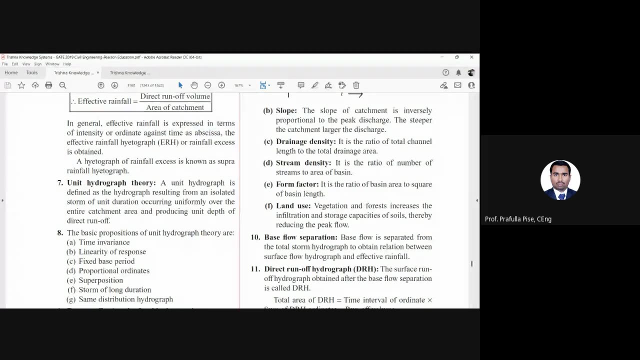 in general, effective rainfall is expressed in terms of intensity or ordered against time as abscissa. now you have to remember what is ordered and what is abscissa. can anyone know? can anyone tell me what is uh ordered and what is abscissa? can anyone tell me what is ordered and what is abscissa? 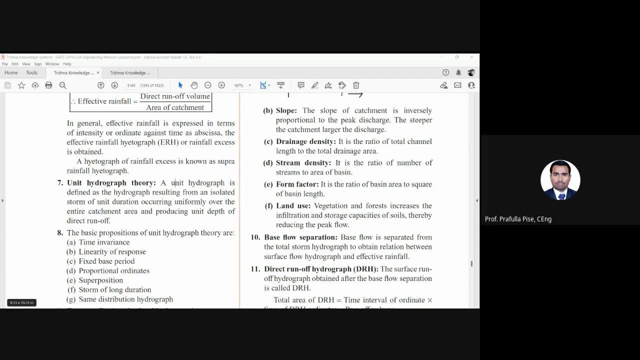 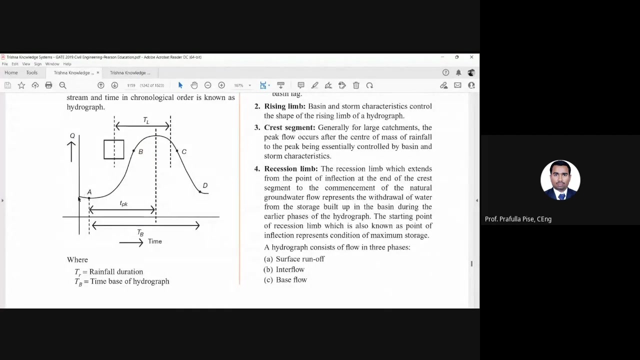 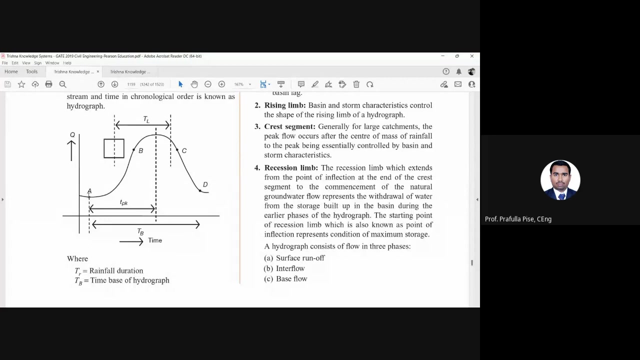 um, um, so when we plot a graph- okay, suppose this is a graph, okay, so this graph, it cuts y axis here. so this, from zero to this, that is what you call as the ordinate, okay, and from, if you try to get like this, so this: uh, cut x axis at this point. from zero to this point is what you call the. 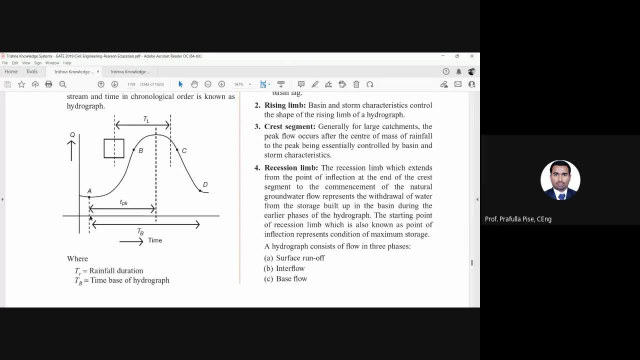 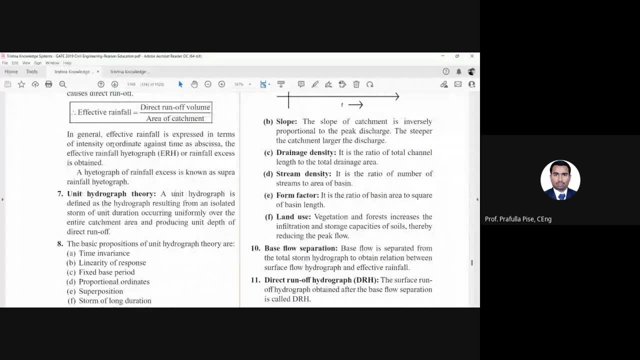 abscissa, so ordinate abscissa, okay. so see, it's quite easy, you know, if you try to understand the basic concept, it's quite easy to find out the answer. so, basically, whenever they find, when they ask you to find out effective rainfall, it's basically: ordinate against abscissa, the. 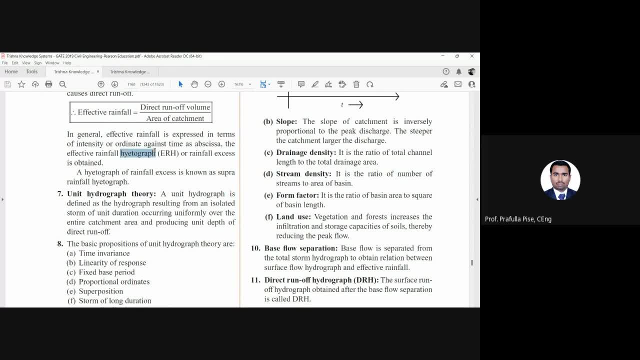 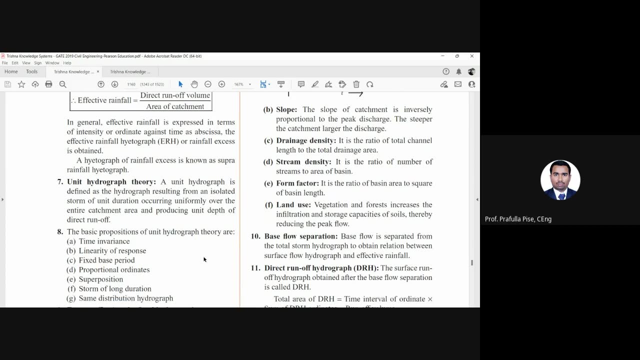 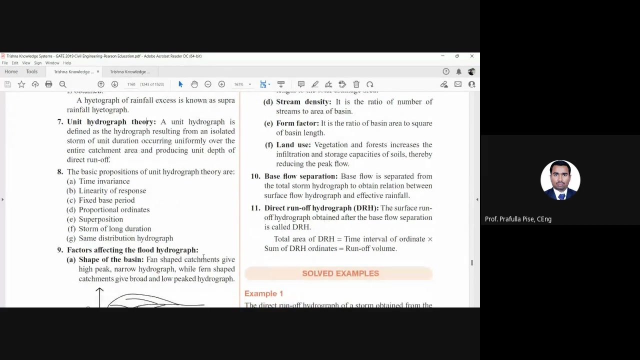 effective rainfall hydrograph. this is a hydrograph, not hydrograph. okay, a rainfall axis is obtained. okay, hydrograph of rainfall axis is known as the supra rainfall hydrograph. now anyone know what is the hydrograph hydrograph and what is hydrograph? difference between hydrograph and hydrograph. 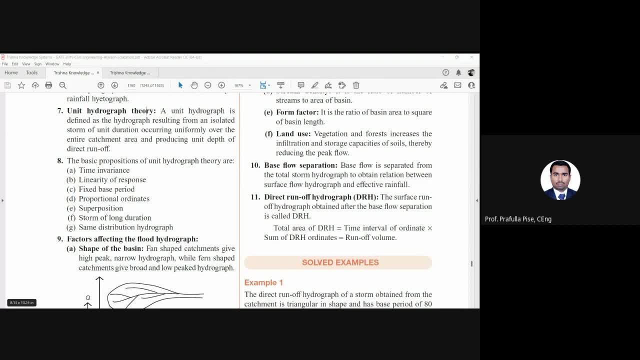 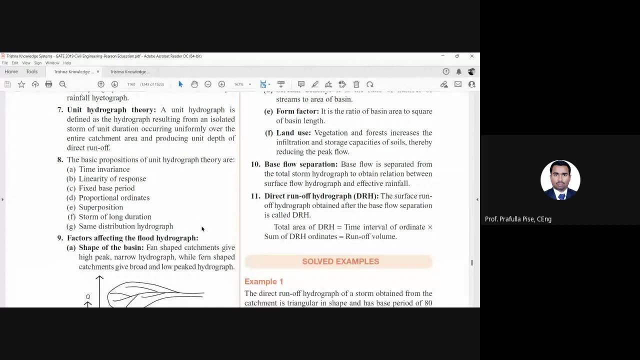 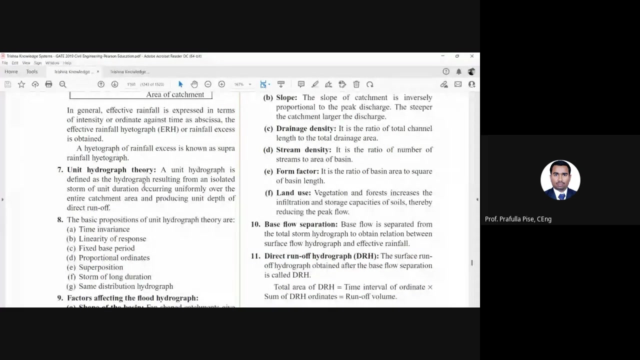 a third, take all the guy but taking a shelter around the kind of hydrograph unit hydrograph theory. a new hydrograph is defined as a hydrograph resulting from an isolated storm of unit duration occurring uniformly over the entire catchment area and producing unit depth of direct runoff. so hydrograph, hydrograph and unit. 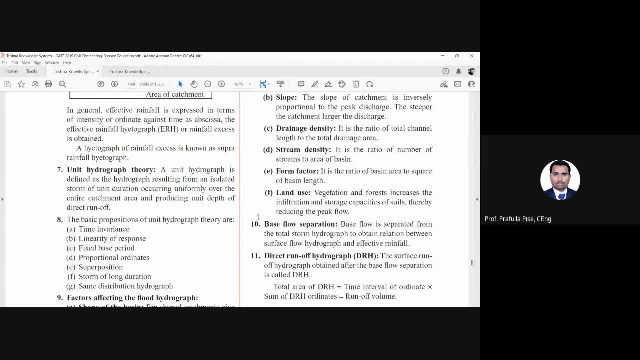 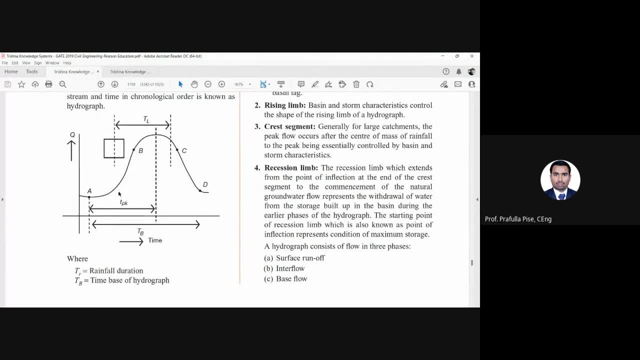 hydrograph. so hydrograph is basically what we have. okay, so this is what we call as a hydrograph. okay, but if you plot a bar, okay, bar diagram. bar diagram means for each hour or half hour, okay, or two hours block. that's what you call as a. 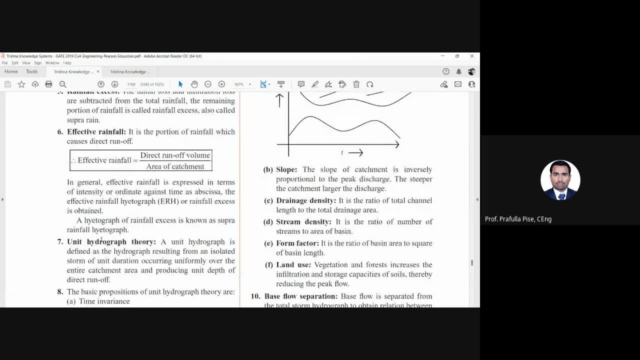 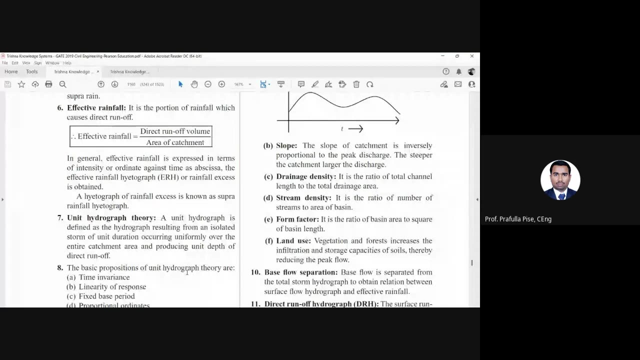 hydrograph. okay, so hydrograph may be for a half hour, maybe for one hour, may for two hours. that's what hydrograph and unit hydrograph is when we have a. a unit unit means one unit depth of direct runoff. unit depth of diagram means one meter or one mm per second. okay, that is sorry. one meter cube per. 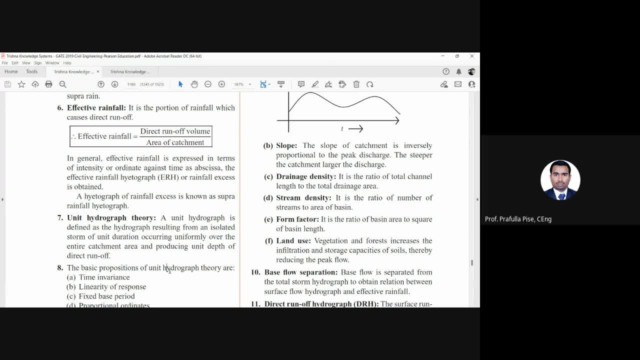 second: okay, so that is what you call as a unit depth of direct runoff. so discharge over time they sorry, that is a hydrograph, hydrographze. when time is the one time, okay. when unidepth is given as the time, okay then– one hour time or half hour time, or two hour time, okay. 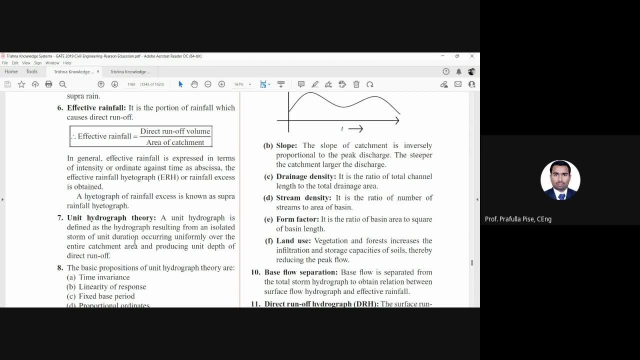 when we do unit in time, it becomes a hydrograph. when we do unit in discharge, it becomes an egg. when we do unit in direct runoff, it becomes an egg, then it becomes a unit hydrograph. okay, that's something you have to understand, you have to remember. 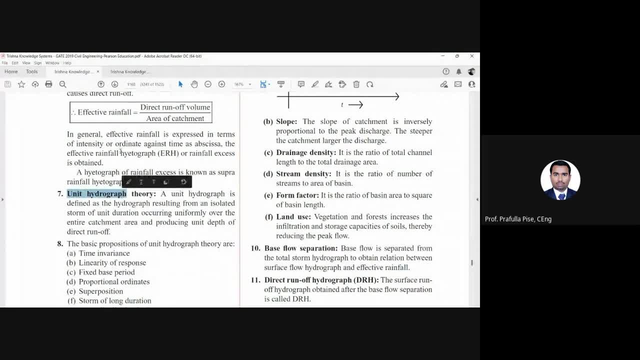 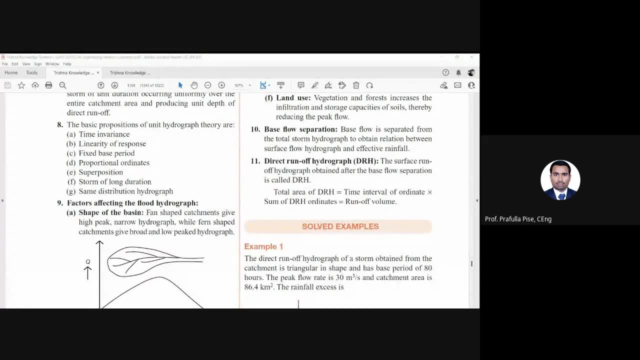 most of the people, they get confused with unit hydrograph and hydrograph. okay, remember what I am saying. is correct or wrong, Rohan? yes, sir, yes, did you understand the unit hydrograph and hydrograph? yes, sir, yes, what did you understand? what did you understand? 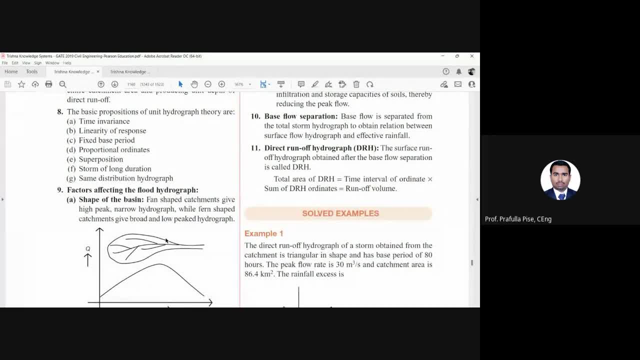 yes, sir. okay, the basic proposition of unit hydrograph theory are time invariance, linearity of response, fixed base period, proportional ordnance, superposition, storm of long duration, same description. so these are the what we call as a basic proposition, or basic assumptions, or basic characteristics of a unit hydrograph. 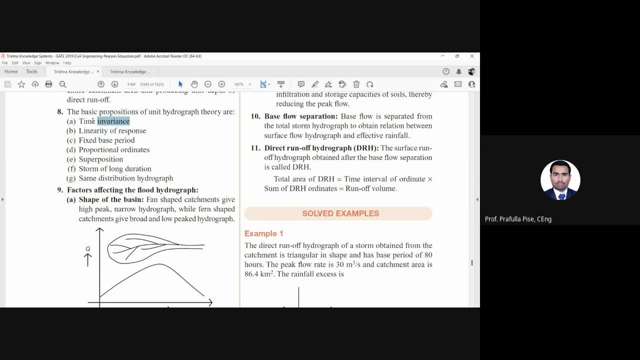 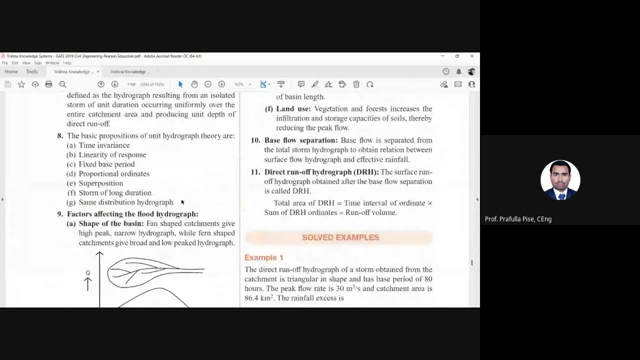 okay. time invariance: same time. also, we don't change the time. linearity of response: okay, so we get the linear response, not the non-linear fixed base period: okay, so if the base of the unit hydrograph is fixed, okay. proportional ordnance: okay, means. 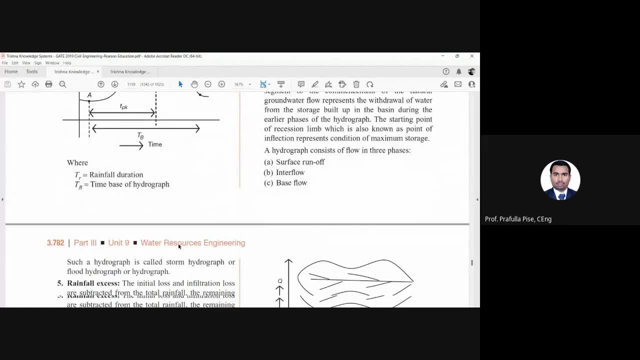 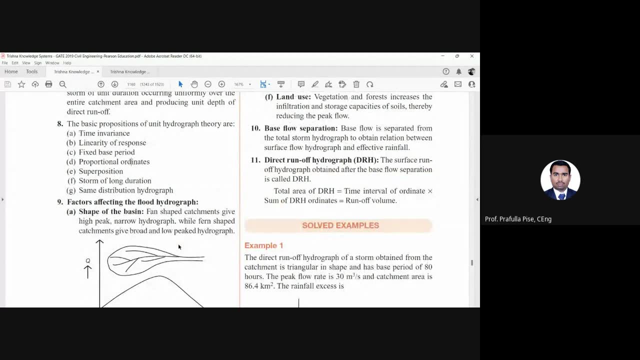 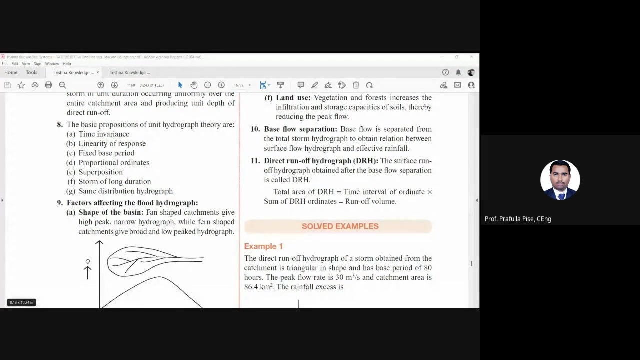 these are the ordnance. okay, they are in proportionate. proportional. there is a correlation in it. correlation means it increases in two steps, or increases in one and a half steps, or increases in three steps. okay, that's what we call proportional ordnance. so yes, 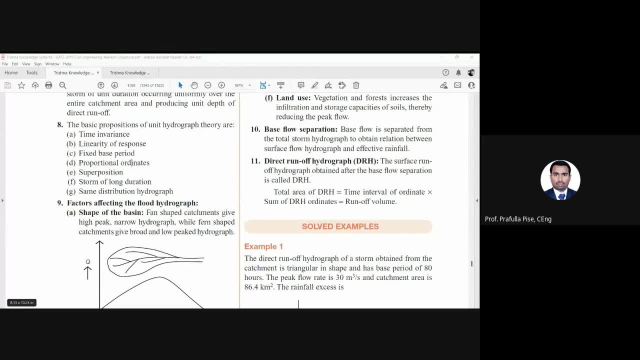 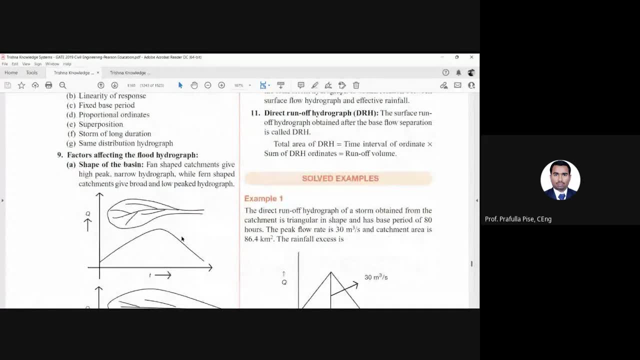 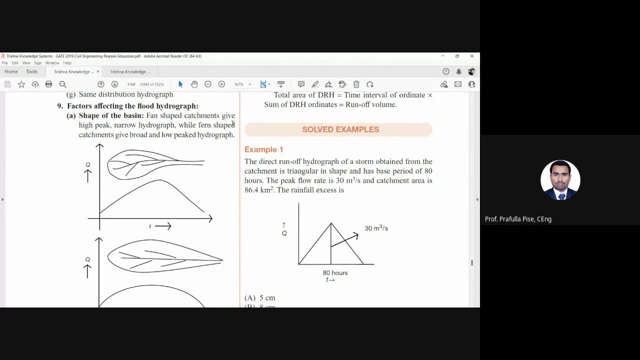 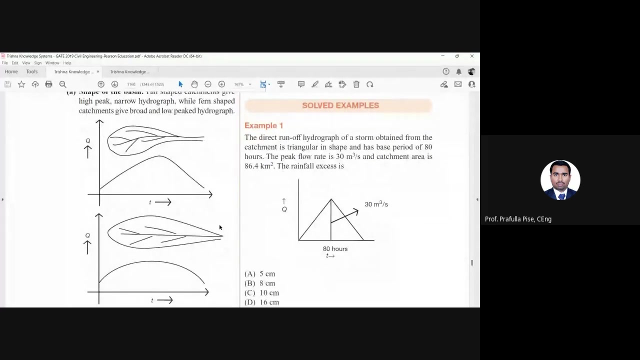 someone ask, want to ask something okay, factors affecting the floor: hydrograph, shape of the basin. fan shaped catchment gives high peak, okay, so that's the fan based. so let's see we have a high peak, okay, and narrow hydrograph, while fun shaped, fun, okay. shaped attachment gives broad and low peak hydrograph. so 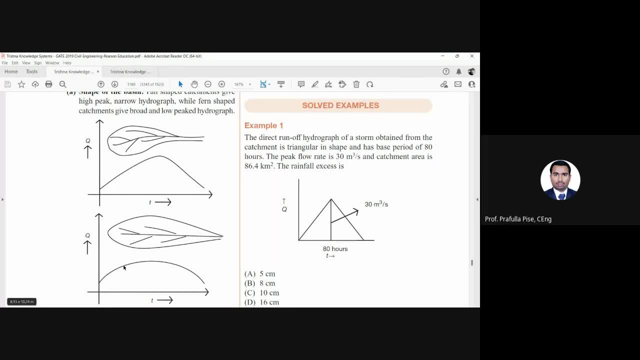 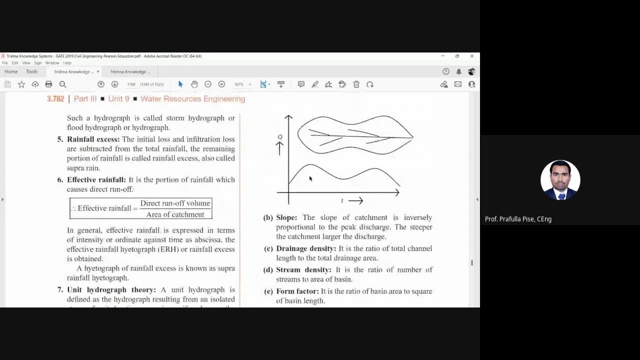 this is: it is low, but it has the largest or larger crest, okay, or you can see, the catchment is something like this. so at this portion- okay, you will see there is a peak. this portion, you will see there is a recession. and this portion again, you will see the second peak. 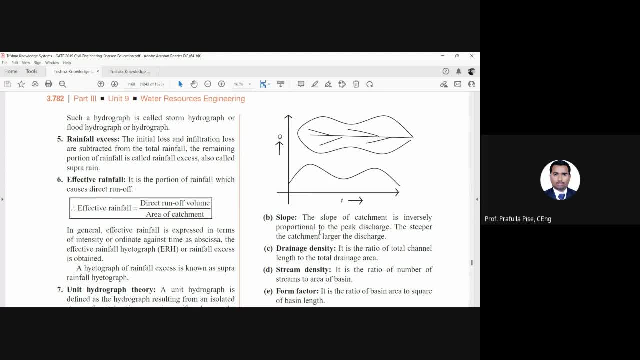 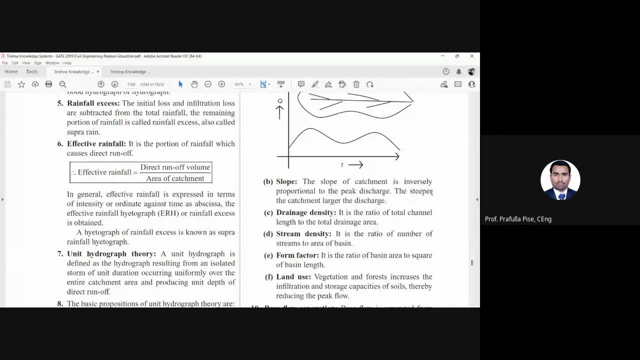 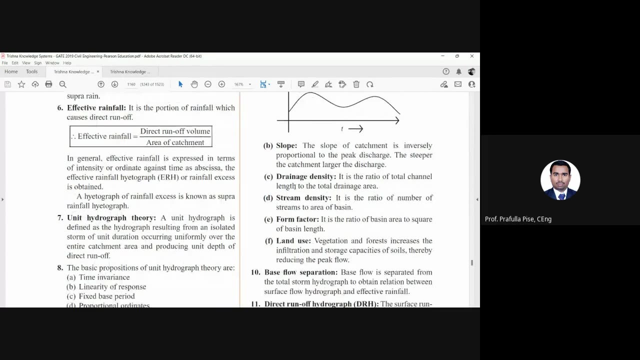 okay, the slope of catchment is inversely proportional to the peak discharge. okay, slope of catchment is inversely proportional to the peak of discharge. peak discharge: the steeper the catchment, larger the discharge. okay. drainage density: it is the ratio of total channel length to the total drainage area. 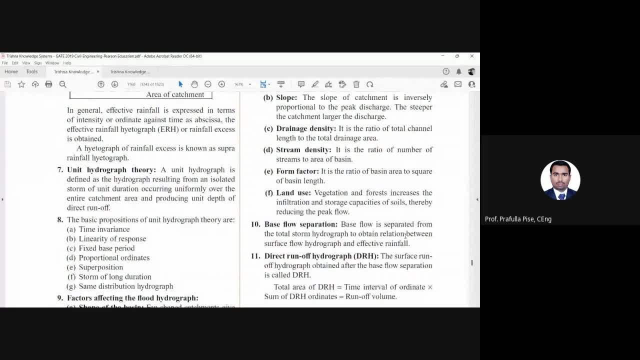 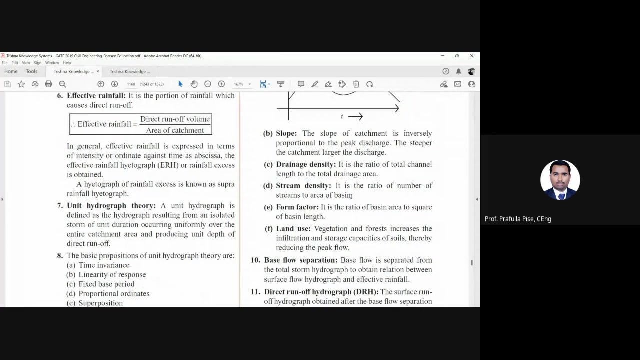 stream density: it is the ratio of number of streams to area of basin. form factor: it is the ratio of basin area to square of the basin length. it is something you have to again remember. form factor: it is ratio of basin area to the square of basin length. okay, so this is length from the uh furthest. 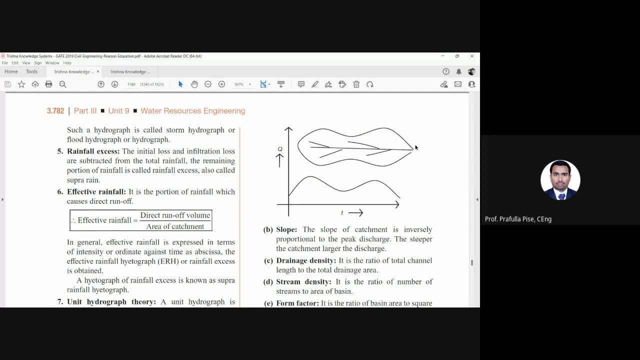 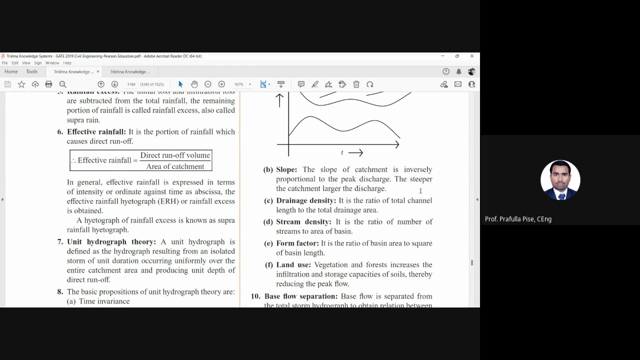 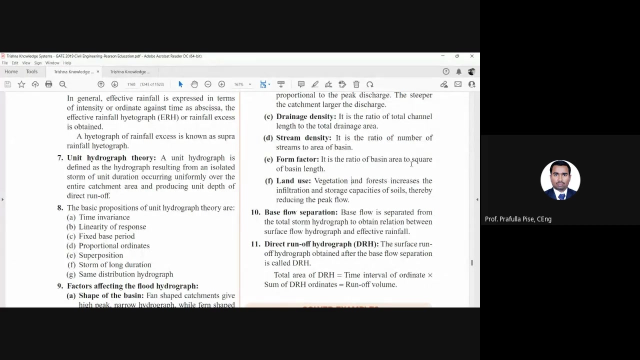 point from the yield point. okay, this is the end point. yield point or mouth. you call it as a yield or mouth. okay, from this point to furthest point, for this point means the second lamp point. that is something what we call as a ratio of basin area to the square of basin area. okay, form factor. 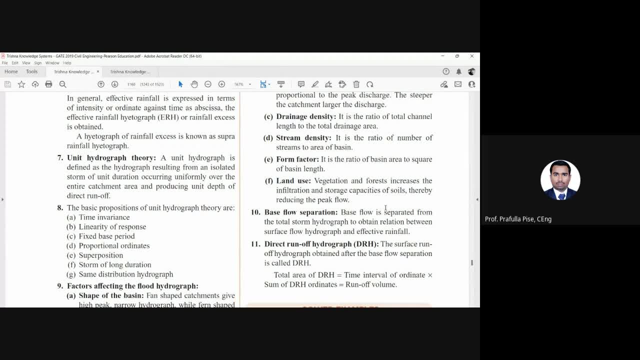 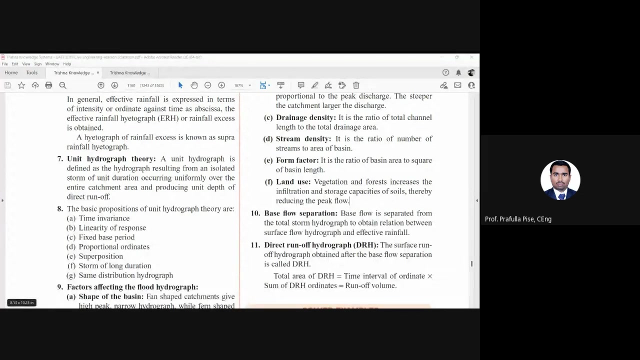 land use, vegetation and forest increase the infiltration and storage capacity of soils, thereby reducing the peak flow. remember that's generally what we think. if you have any questions doubt, please do ask me. if you have any questions doubt, please do ask me. okay, okay, okay, okay, okay, okay. 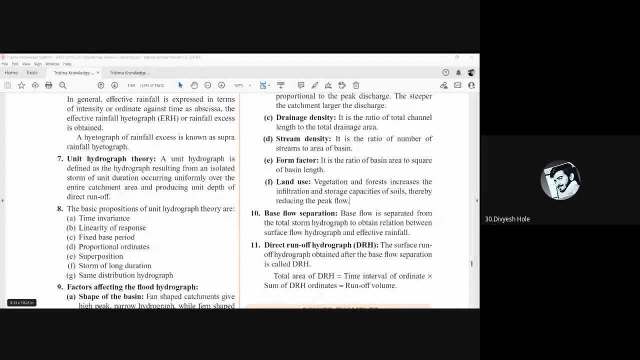 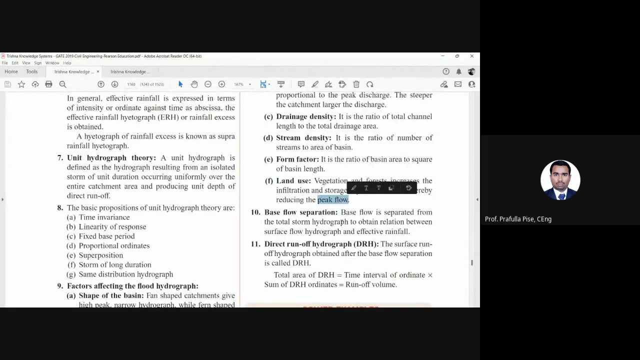 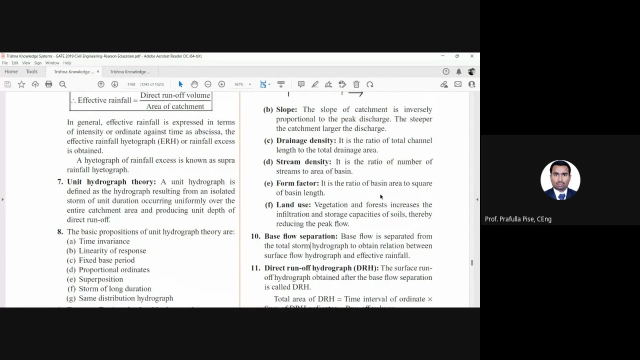 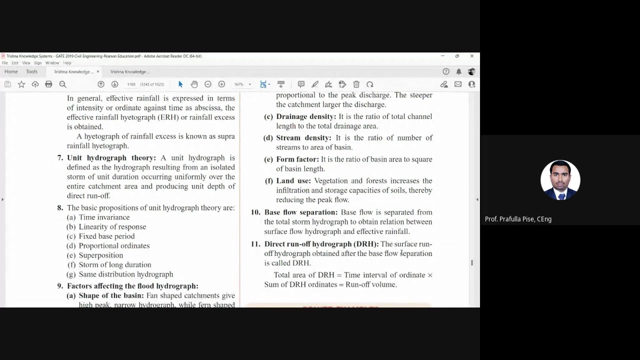 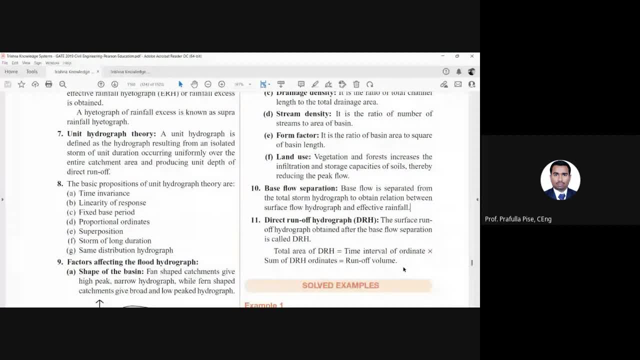 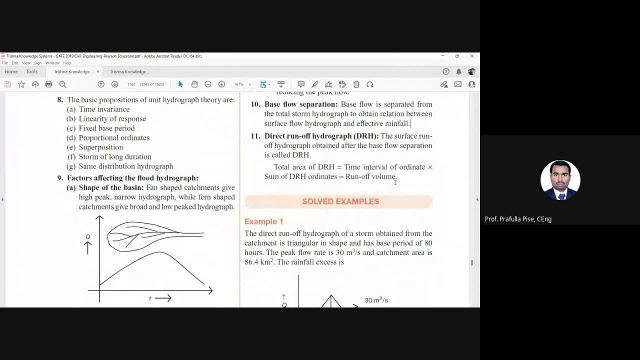 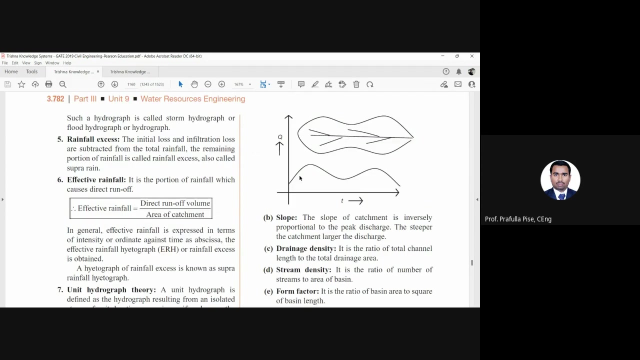 okay question point, but best for best flow separation. best flow is separated from the total storm hydrograph to obtain relationship between surface flow hydrograph and effective rainfall. so we already know what is base flow, right, where best flow is basically, you know. so, at this one here, which is constant, that's called that. we call it as a 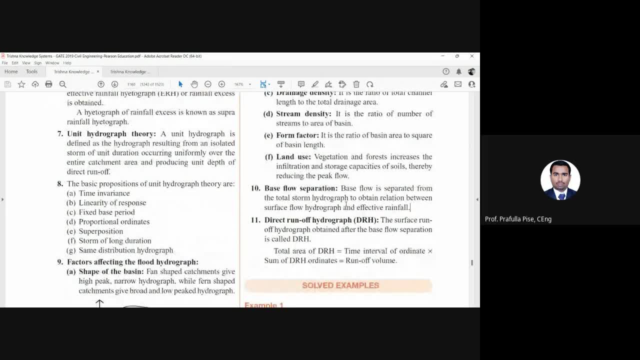 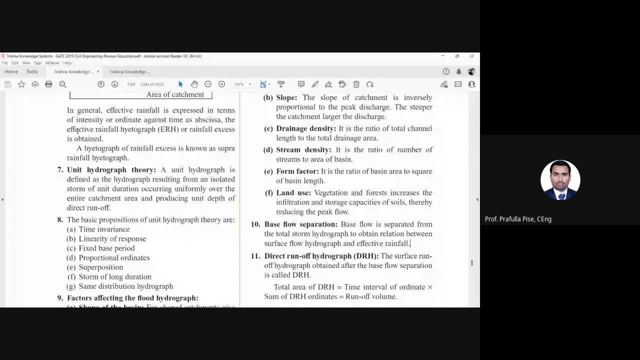 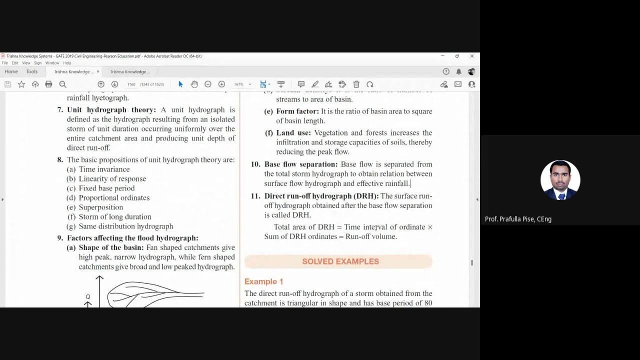 best flow. and if you take it out now, drh, direct runoff hydrograph, okay, there is one term here, erh effective rainfall hydrograph and here drh direct runoff hydrograph. the surface runoff hydrograph obtained after the base flow separation is called drh. the total area of that red for uh hydrograph equal to time interval of ordinate. 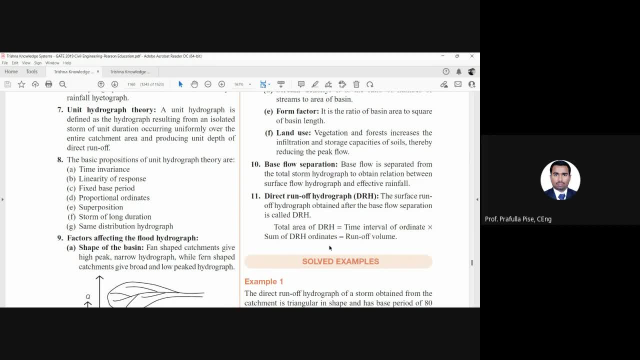 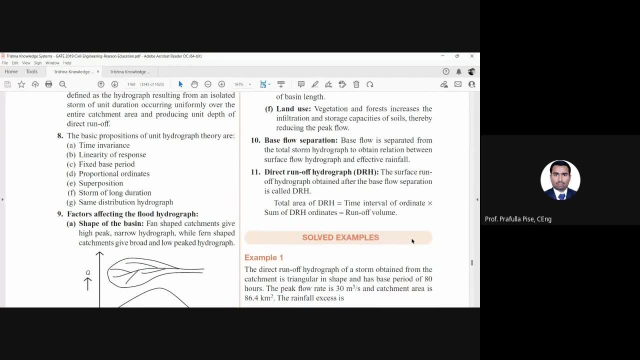 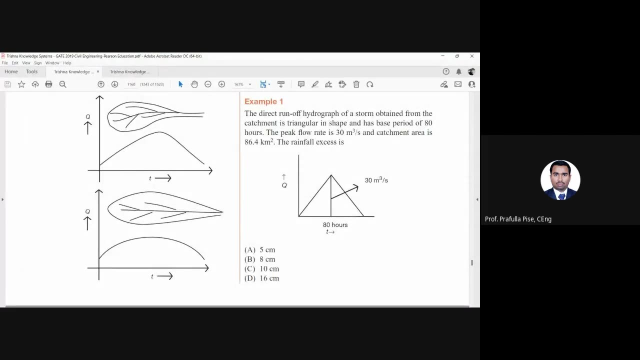 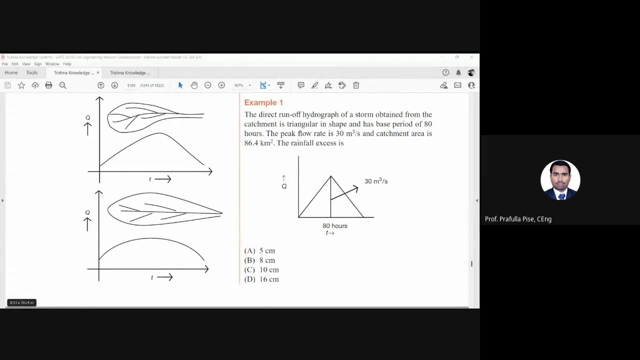 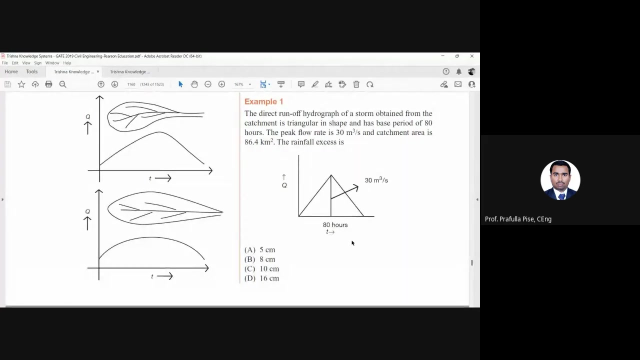 times multiplied by sum of drh ordinates. okay, that will give you a runoff volume. okay, now we will see one problem. um, now, now try this first problem. direct runoff hydrograph of a storm obtained from the catchment is triangular in shape. okay, triangular shape. so basically, maybe this kind of catchment area we have. that's why we get a. 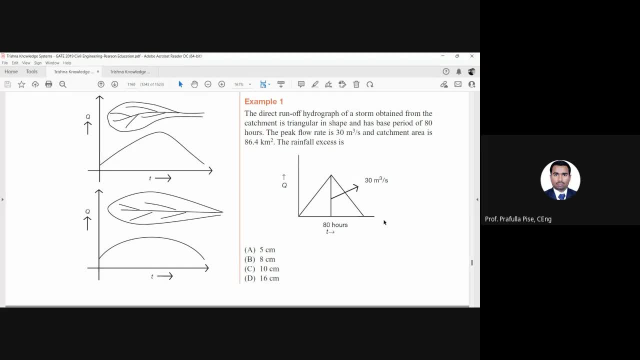 triangular shape okay and has the best spread of 80 hours. so 80 hours best rate they are already, i think. take out the peak floor rate is 30 meter cube per second, peak. that is the peak, so it is 30 meter cube per second and catchment area is 86.4 kilometer square. 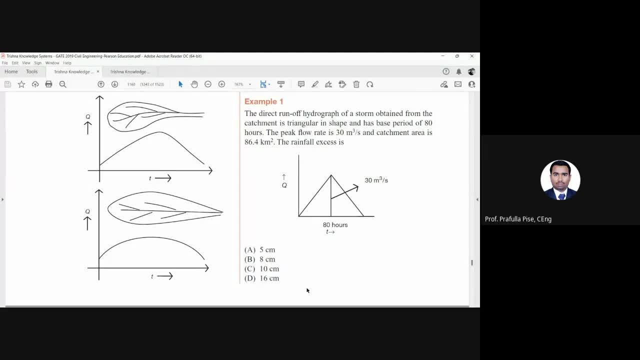 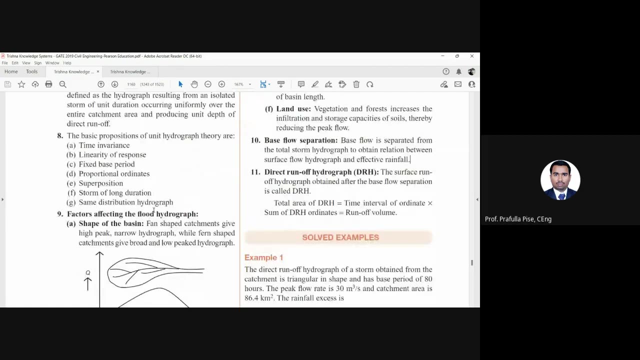 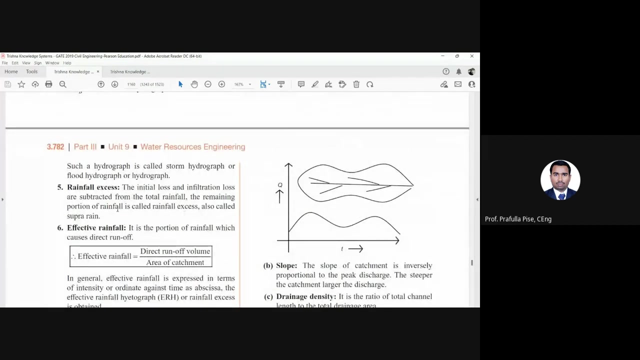 the rainfall excess is. now we have to find out the rainfall excess. so how can we find the find out the rainfall excess? so we already know the rainfall excess is what we have here- effective rainfall- okay, and if you keep going for the rainfall excess, so we have. 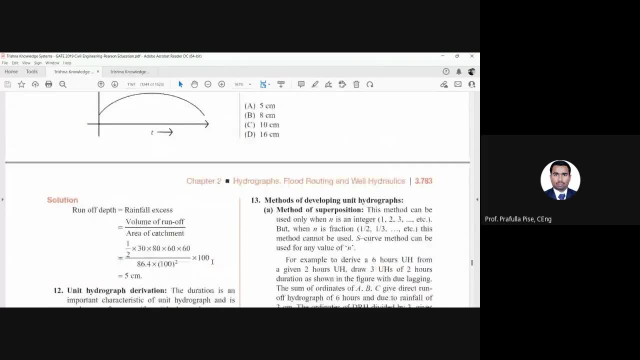 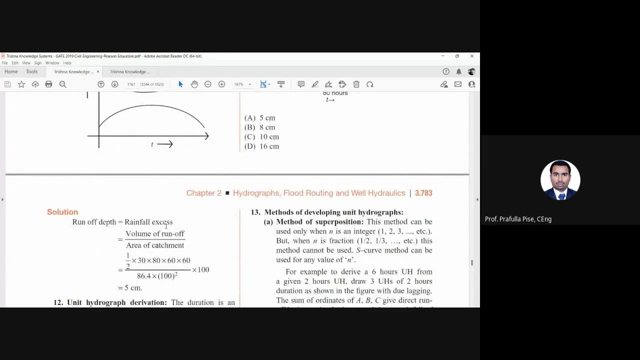 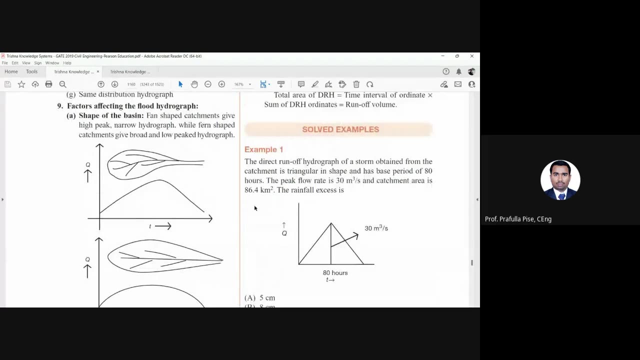 to first find out the effective or we can directly find out the influxes. so the volume of runoff depth equal to rainfall excess equals to volume of runoff over the area of catchment. so area of catchment, we know 86.4 kilometer square. so kilometer squares means 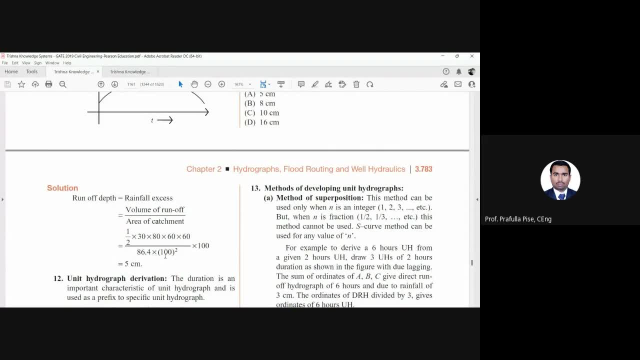 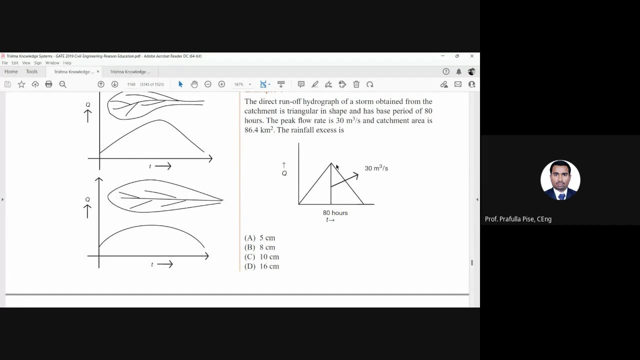 we are going to convert into meter square, so 86.4 times 100 square, so that will give us a meter square. but now what is the volume? so we have to find out the volume. the volume is nothing but the area of this triangle. okay, so wherever the diagram is one half. 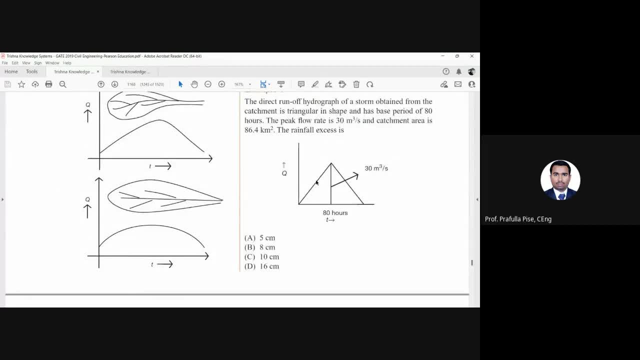 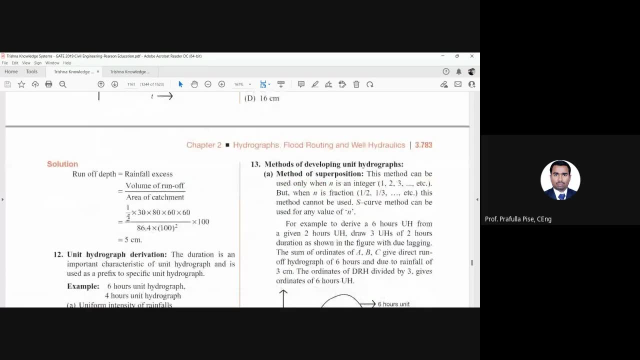 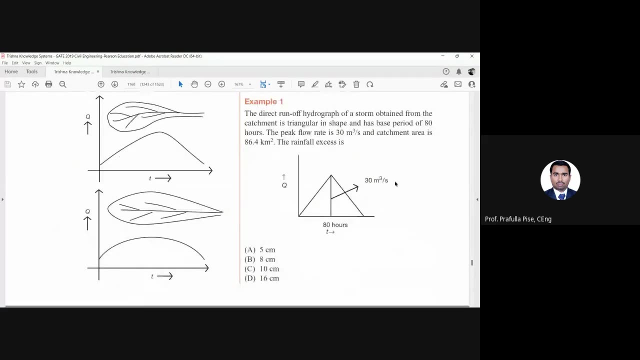 80 times 30.. area of this triangle is one half 80 times 30 base times height. right, so, one half 80 times 30.. now why they have 60 times 60? because that is in per second, okay, and this is in hour. 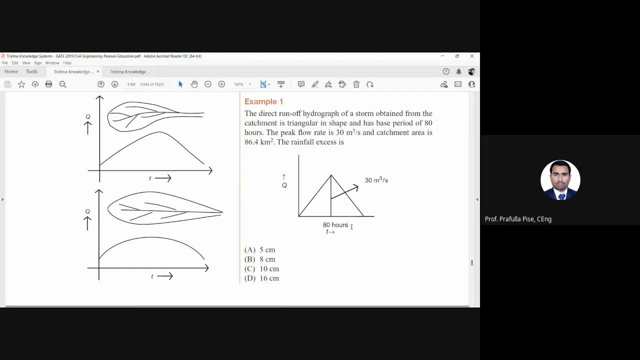 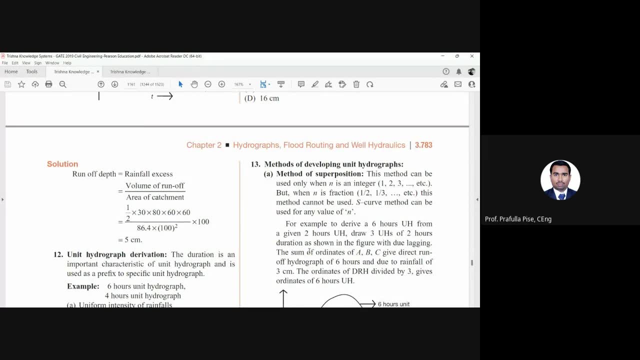 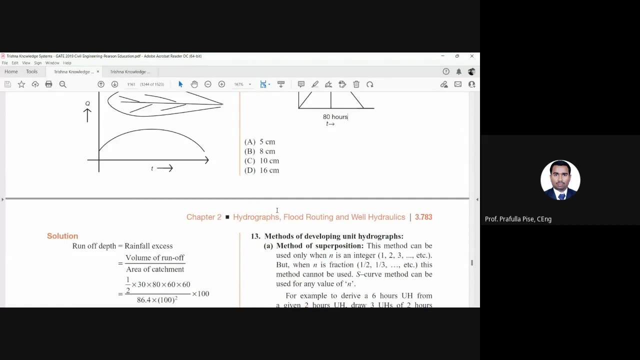 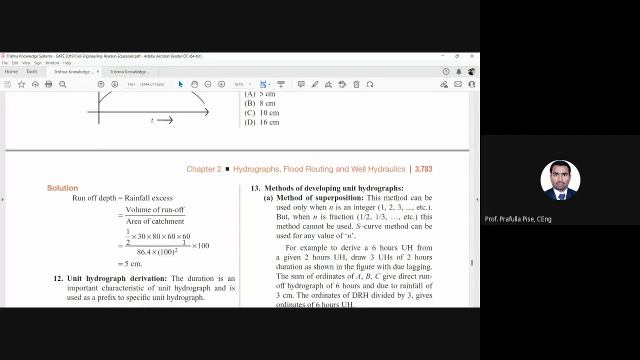 so we have to convert that. we have to convert that into hour or into the second. we have to get both things in same unit. so instead of hours, we are going to take everything in second. okay, so that's why 30 times, 80 times, 60 times, 60, 60 minutes, 60 seconds, so the 80 hours becomes. 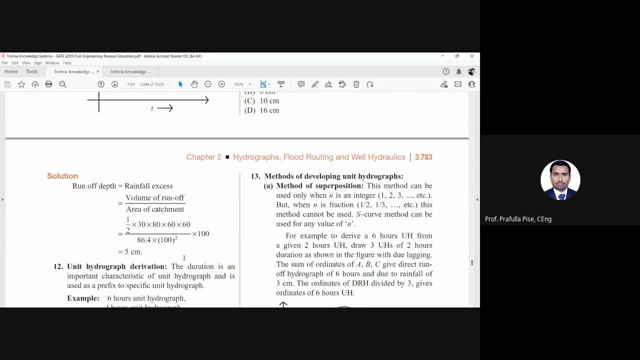 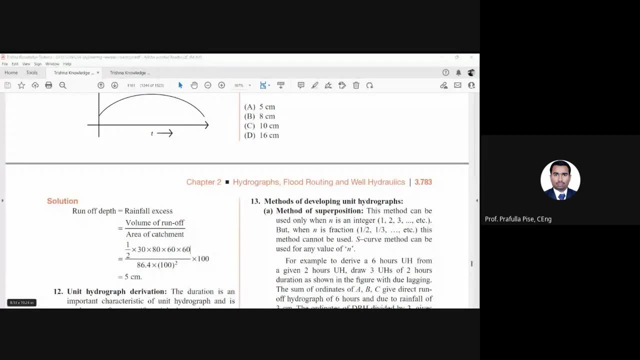 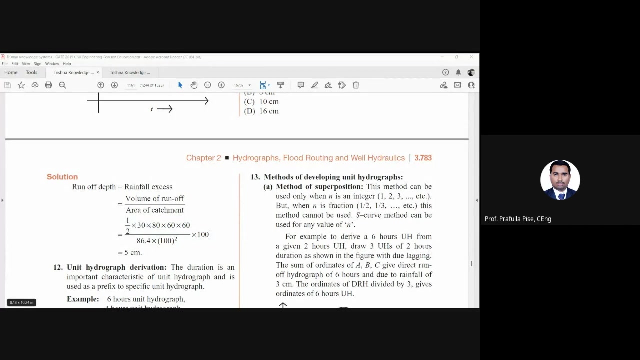 this many seconds, okay, so show you it. why, why, why, why, why they have multiplied by 100 here, Sanika, in Lugari, Lugari- I should have gone to Lugari, Sanika, do you have any idea how they have multiplied by 100?? Sanika, do you have any idea how they have multiplied by 100?? 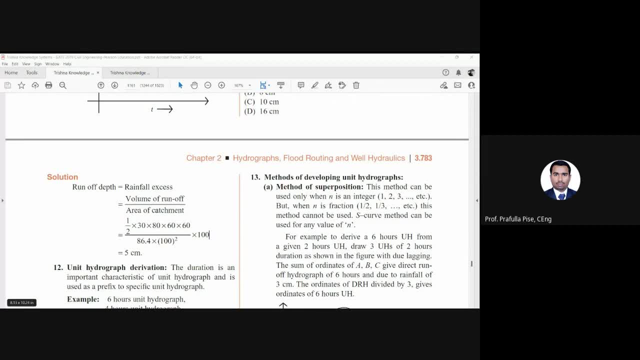 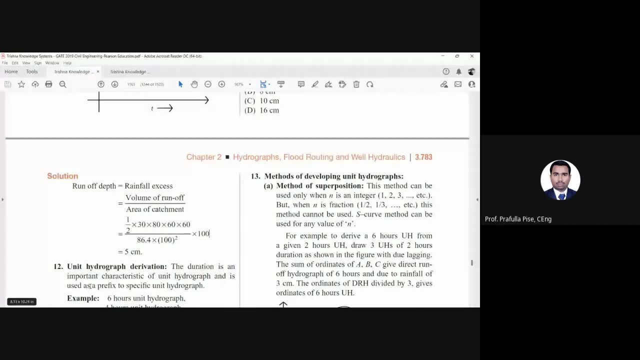 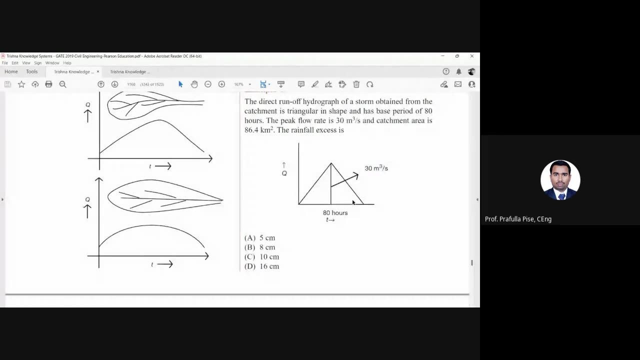 Sanika. Ok, so keep in mind how we are working. We are working in meter cube. Ok, so keep in mind how we are working. We are working in meter cube, And in meter cube we have multiplied by 100 How you were given the options. 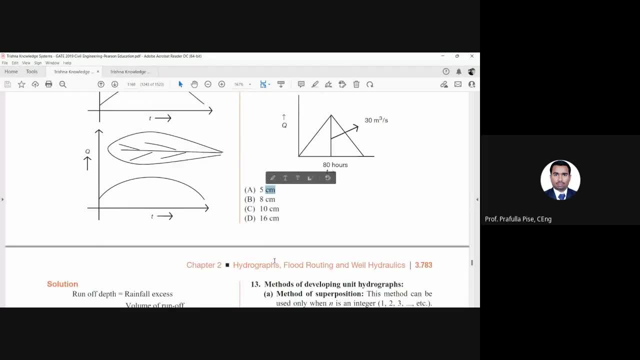 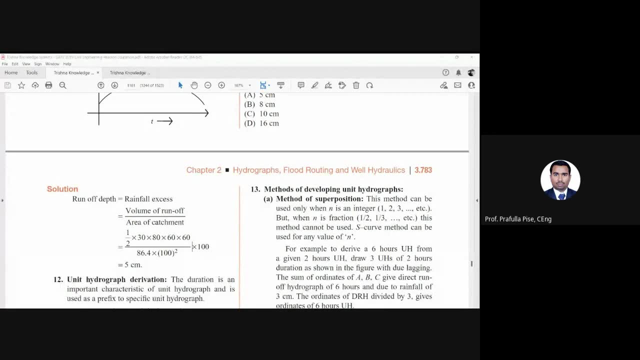 They were given at centimeter And they were given at centimeter And they were given at centimeter. So these are the tricks they used in, now use in the gate examination. So these are the tricks they used in, now use in now use in gate examination. 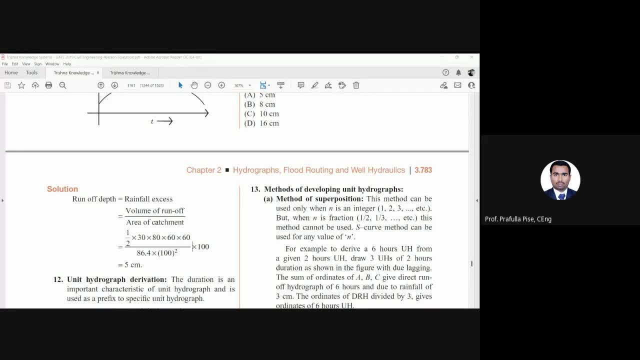 The time they have given is Hour. 90% of the time that they have given in hour- okay, area- they have given in kilometer. okay, discharge they have given in meter cube and the options, the answers, they have given in centimeter. so everything is in different unit. 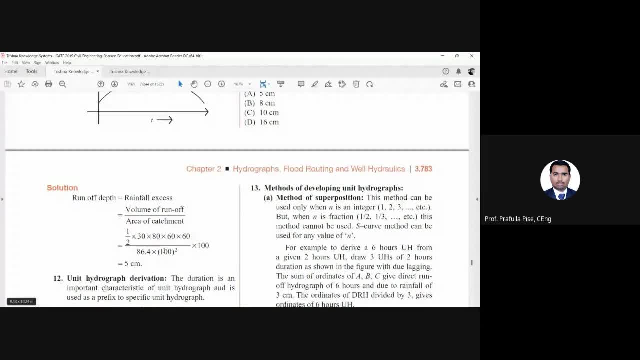 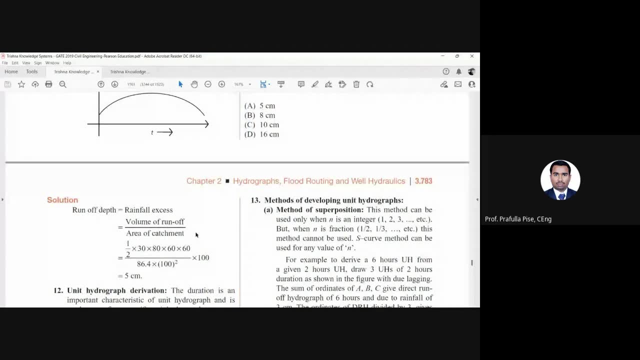 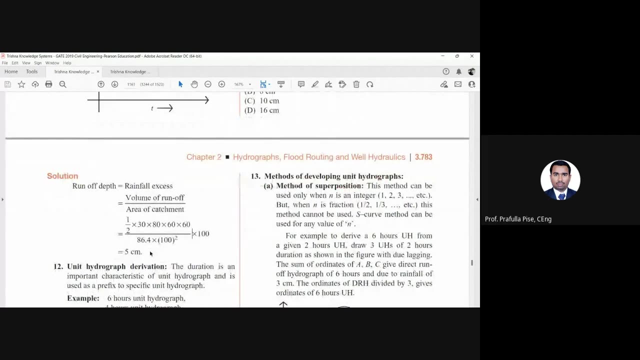 okay, everything is in different unit and that's where people do mistake, okay, so you have to understand, you have to remember, get everything into one unit and then you have to do collection. then your answer will be: the answer is simple: one half times 30 times 80, divided by 86.4. 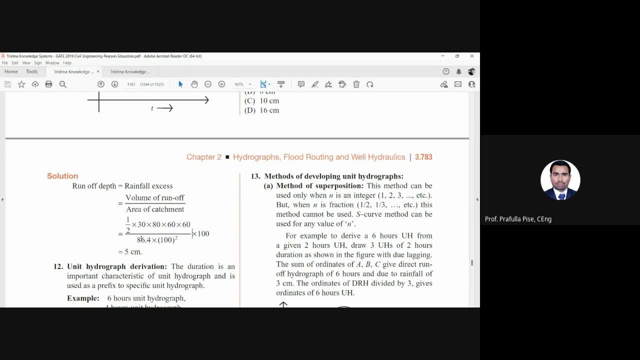 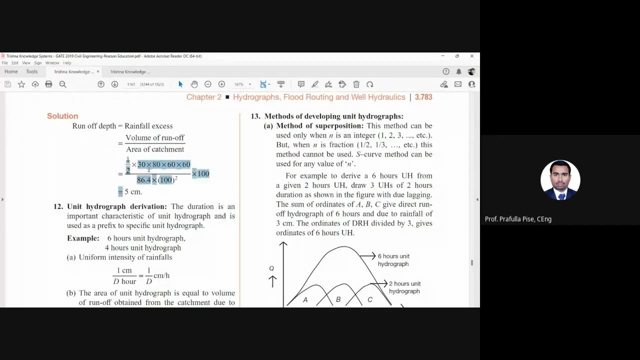 but since this was kilometer square, so we have to convert it into meter square. this was in hour, so we have to convert it into second and everything was in meter, so that's why we have to convert that into centimeter. okay, keep this in mind when you are looking at the answer. solution. 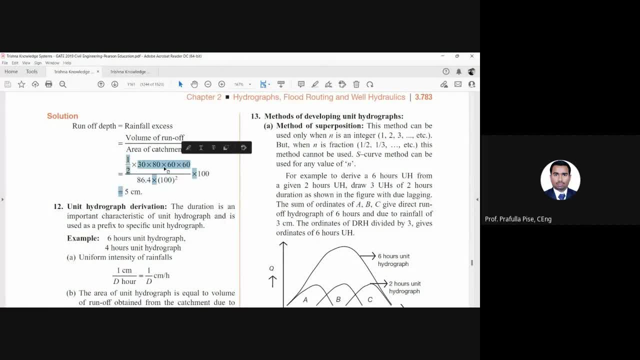 you have to remember that. how did we get this 100?? how did we get this 60?? how did we get this 100?? how did we get this? this is nothing but the unit conversion. that's the trick they use in gate examination. okay, 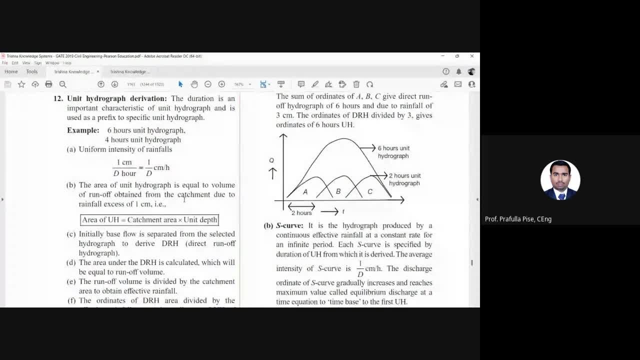 so please be attentive or be pay attention to the minor details. these are very important details. now, unit hydrograph derivation: the unit hydrograph is an important characteristics of unit hydrograph and is used as a prefix to specific unit hydrograph. and all these things. have you taken them? 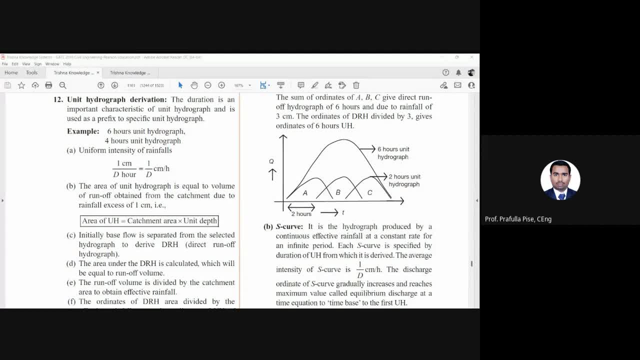 have you taken them? okay, you have taken them. the question which I am asking you- you should have asked me that question- that, sir, where did this 100 come from? where did this 60 come from? I am not asking you the question, I am asking you the question in reverse. 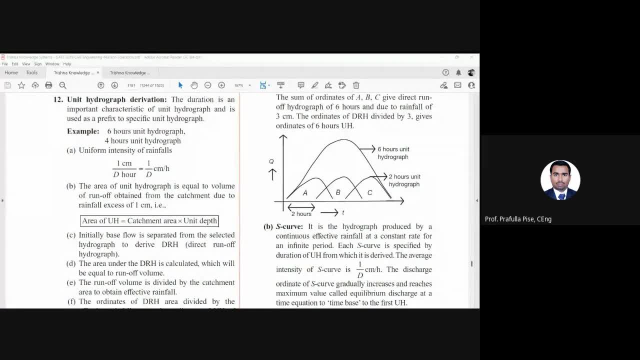 do you understand what is going on, because I was not able to find out. Rohan Vaishnavi. Harsha Vardhan. Sir. yes, sir, you are listening to what is going on. you are sitting in the lounge. I am listening, sir, so why are you not answering such questions? 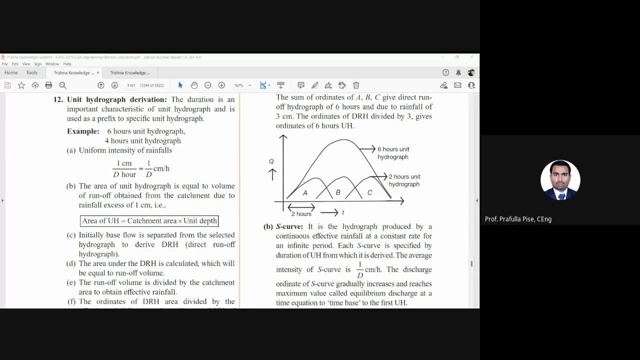 that, sir, tell me which unit is 60? or tell me which unit is 60?. when should I ask you the question? because we know which unit is 60 and which unit is 100?. knowledge number: the might as it's on your stay. might as it's a, whichever that's a class. 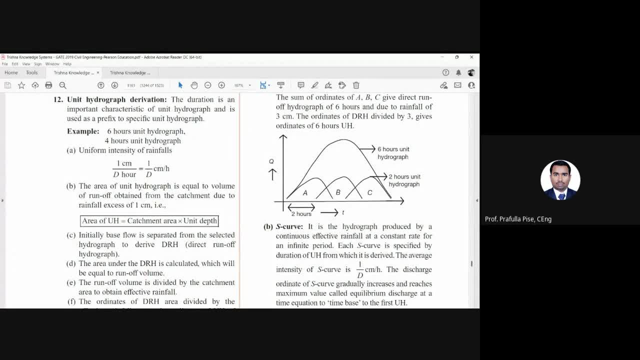 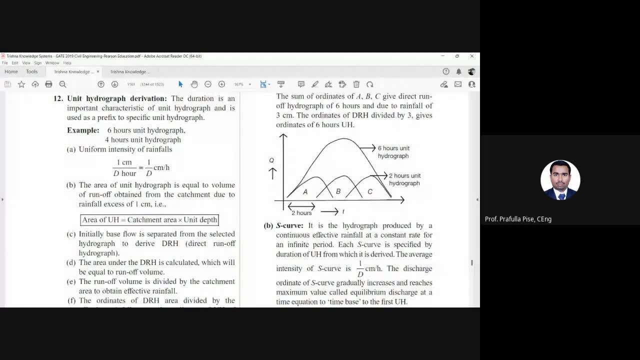 I have a platicate, so much it's a doubt, clear cutting, and so put them in question. it's written. I don't know, I don't check, I doubt it. there I'm gonna tell me what you're going to say. that's our attack. that's our attack. okay, Englishman at the Marty me, which I mean. 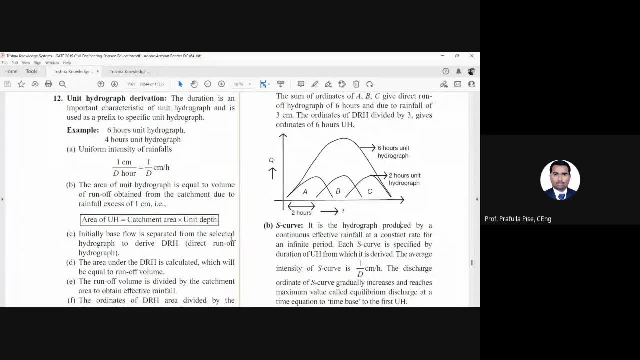 my teammates on tour. I probably think I'm put the water unit hydrograph derivation. the duration is that important characteristics of mid hydrograph and he is used as a prefix to specific unit hydrograph. okay, now prefix my castor upon me. me I will do six hours. four hours, that is called. 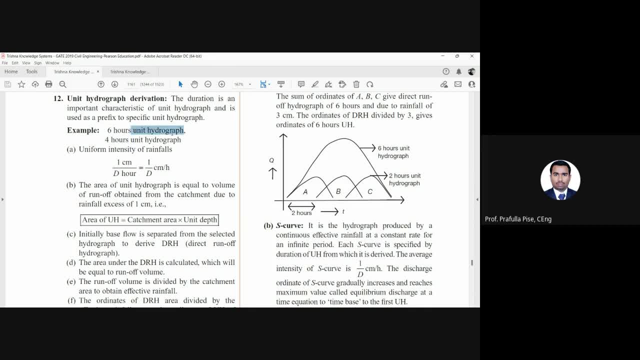 prefix: okay, and that is the top of unit hydrograph okay. however, the third time little, and then second video. uniform intensity of rainfall one centimeter over D hour equal to one hour, be centimeter per hour. that's called in form intensity of them for Java coming to me into steam antenna electricity. whenever they say intensity, it is: 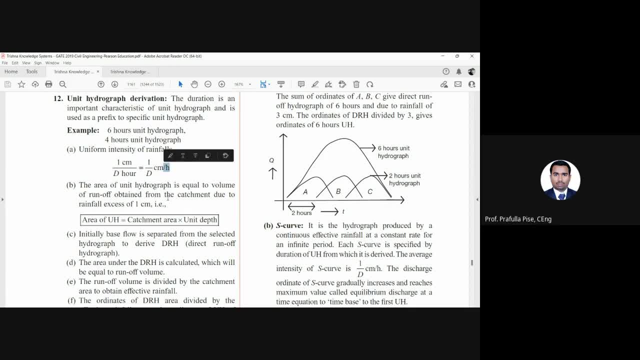 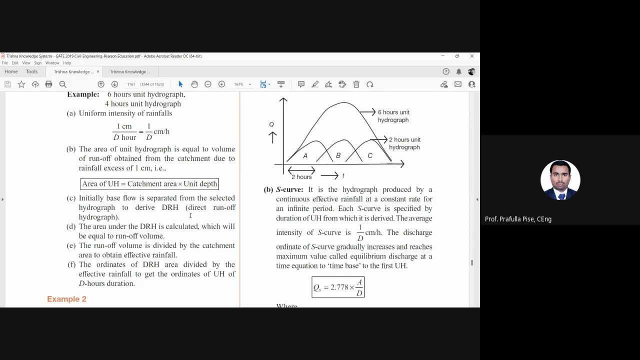 always with respect to time. okay, that's what they have. intensity and the area of unit hydrograph is equal to volume of runoff obtained from the catchment due to rainfall excess of one centimeter. that is area of u, h, u, h. is unit hydrograph equal to catchment area times unit depth? 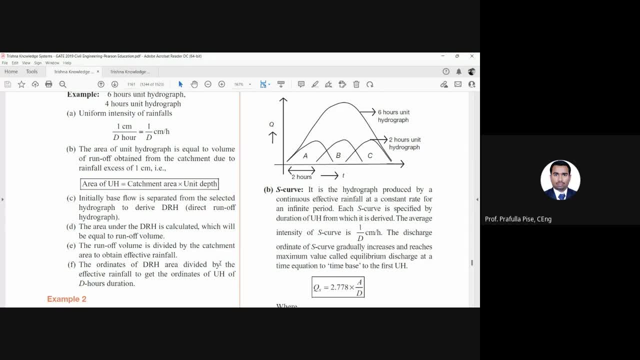 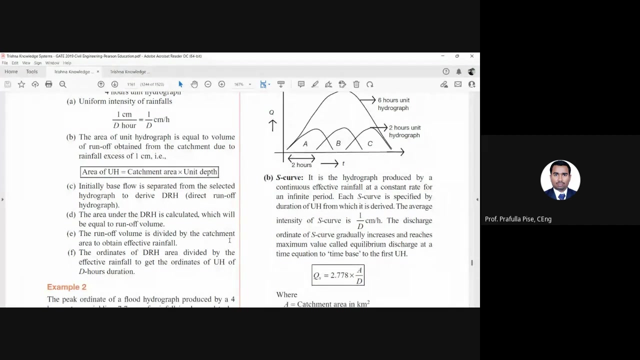 initially, base flow is separated from the selected hydrograph to derive drh diagram of hydrograph. the area under the drh is calculated, which will be equal to runoff volume. the runoff volume is divided by the catchment area to obtain effective rainfall. the ordnance of drh area divided by the effective rainfall to get the ordnance of. 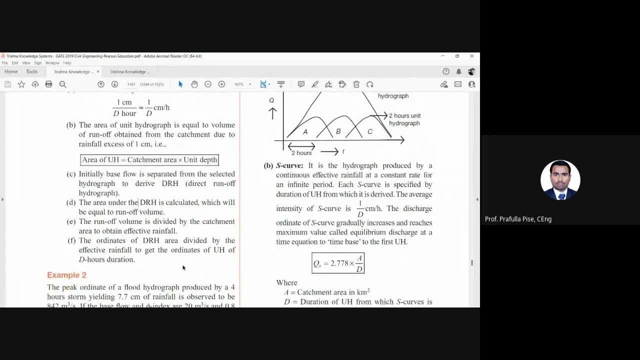 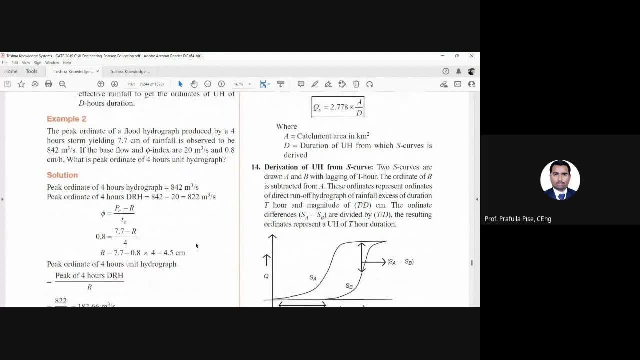 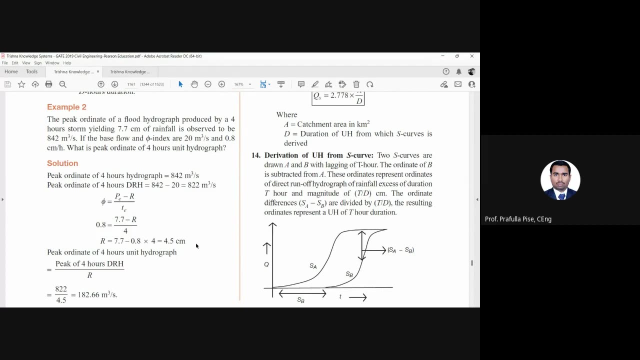 u h unit hydrograph of a d hour duration. so let's see the problem: the peak ordinate of a flood hydrograph produced by an four hour storm. okay, remember, they say four hour storm for our storm. they hydrograph the actual storm of the both side. okay, so for our storm. 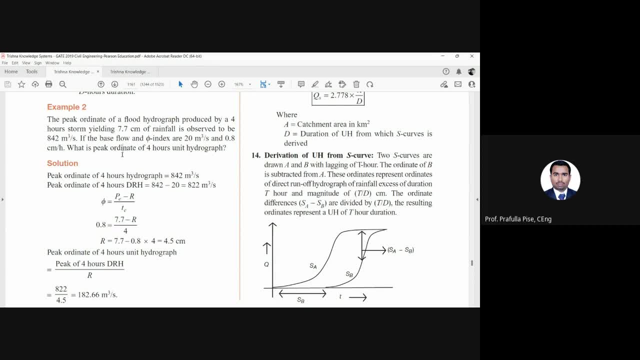 yielding 7.7 centimeter of rainfall is observed to be 842 meter cube per second if the base flow and phi index are 20 meter cube per second and zero point eight meter centimeter per hour. so base flow is 20 meter cube per second and phi index is: 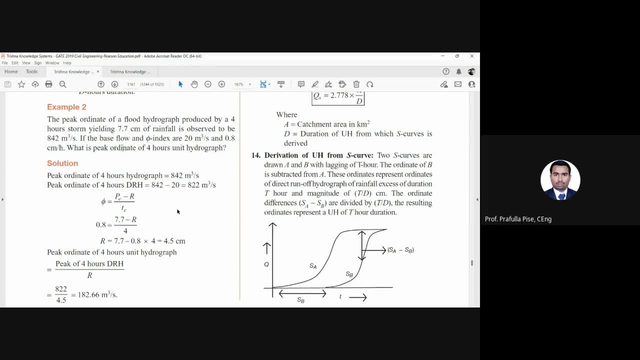 uh, 0.8 centimeter per hour. what is the peak ordinate of four hour unit hydrograph? okay, now they ask about the four hour unit hydrograph, so how we can solve it. the peak audit of four hour hydrograph is equal to: that's what they given us. 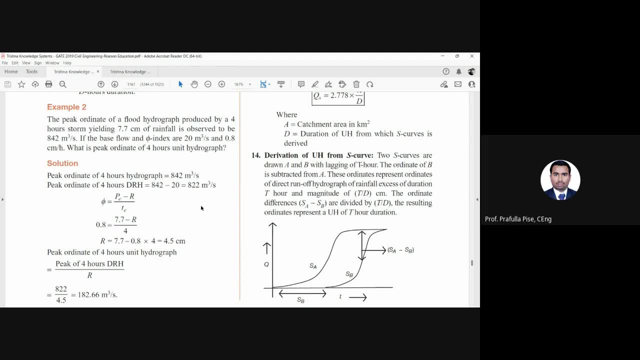 842 meter cube per second, because that's what they say: peak ordinate. okay, peak ordinate this much. so that's why we know this is in forward, the peak order for a hydrograph at the- uh sorry, director of hydrograph. so we have to subtract the base, the base flow to get 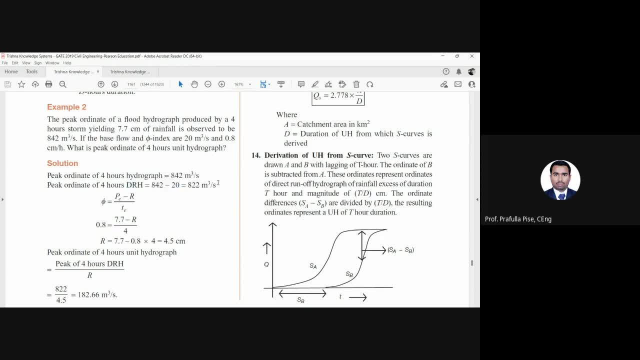 time runoff. so subtract 20, we get the peak of drh. now we have the formula for phi index: p e minus r over t e. okay, so what was the effective uh or precipitation? so that was 7.7 centimeter minus r runoff, runoff uh divided by: 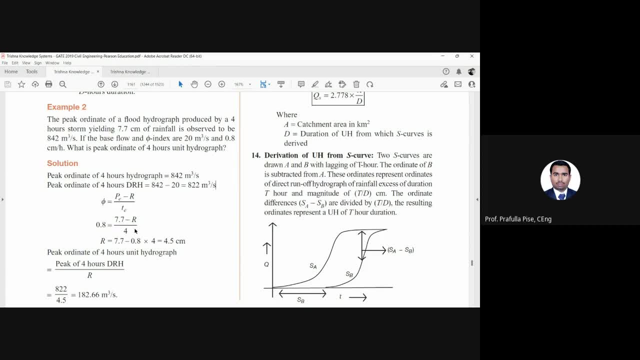 t the time of effective time, so which is uh. four hour, yes, that's what they have given us: four hour. so 7.7 minus r over 4 equals to 0.8. if you rearrange it, you will get the r, which is uh. 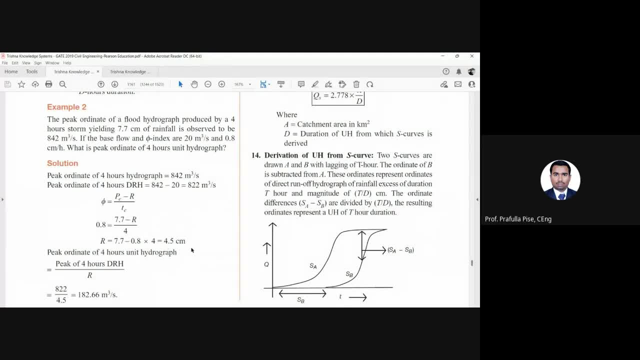 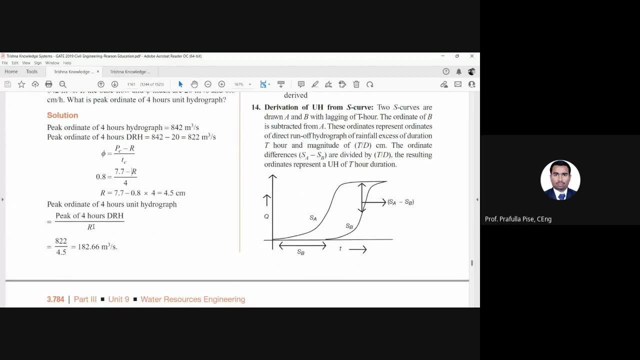 runoff: uh, 4.5 centimeter. so the peak orders of four hour unit hydrograph: okay, peak divided by r. so what was that? uh, we got 822 divided by 4.5 centimeter will give us 182.66 meter cube per second. 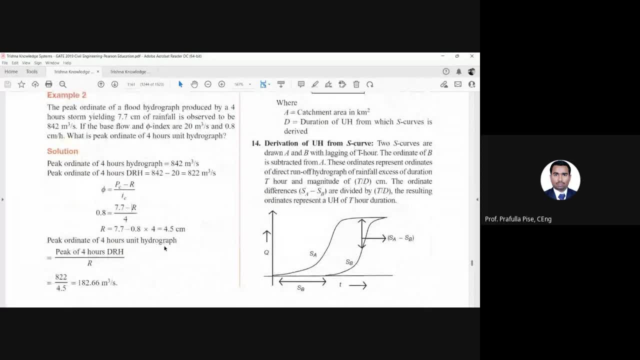 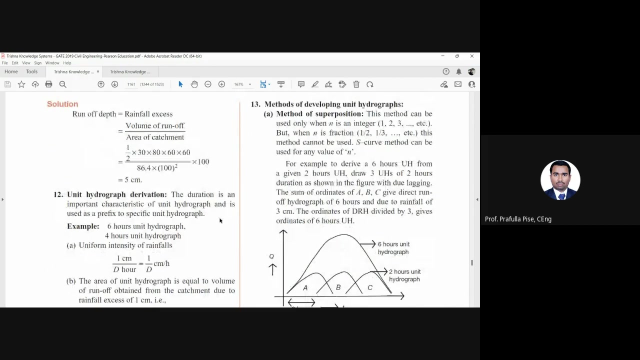 understood how we got this answer. they have not given us any of the options, but that's how you can find out the answer. next, move on to next methods of developing unit hydrographs. method of superposition: this method can be used only when n is an integer. okay, 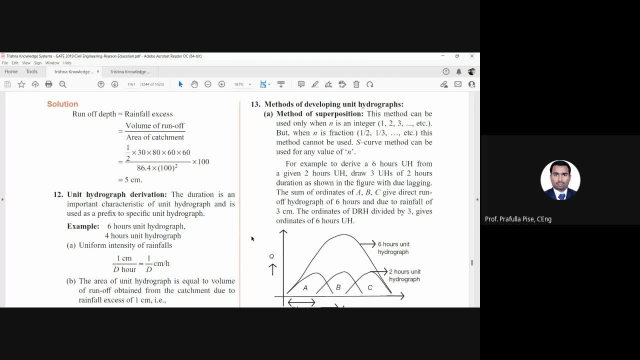 so basically one, two, three, four. but when n is a fraction, so one half, one third, this method cannot be used. s curve method can be used for any value of n, so superposition and s curve superposition is for when n is integer s curve when n is either integer or fraction. 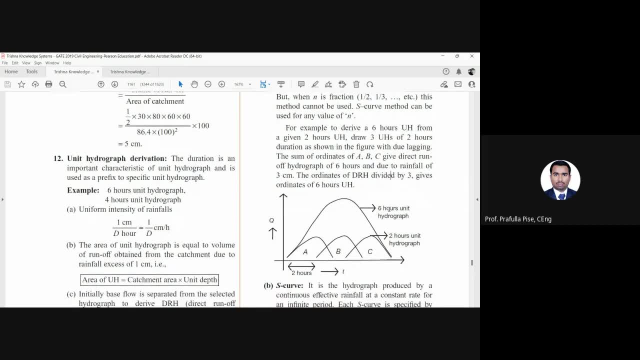 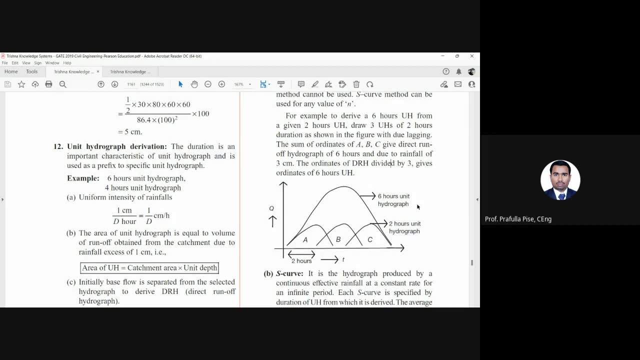 For example, to derive a 6-hour unit hydrograph from a given 2-hour unit hydrograph, draw 3-hour unit hydrographs of 2 hours duration as shown in the figure, with due lagging, The sum of ordinates of A, B, C give direct runoff hydrograph of 6 hours and due to rainfall. 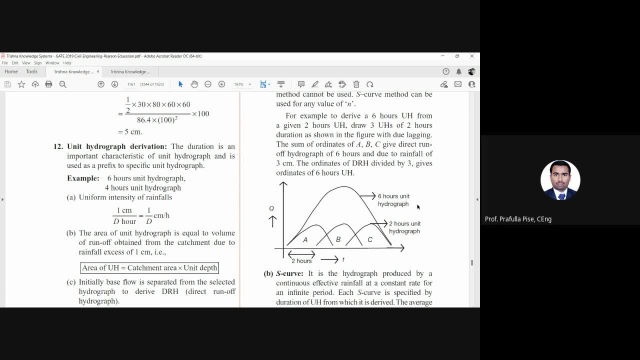 of 3 cm. The orders of DRH divided by 3 gives orders of 6-hour unit hydrograph. So we have A, B, C. these are the 3 unit hydrographs of 2 hours And if you superimpose the 3 unit hydrographs of 2 hours, 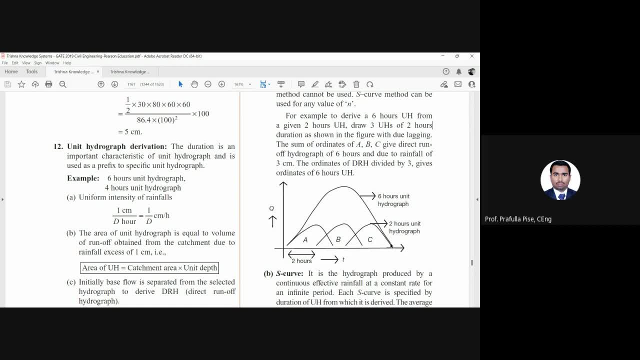 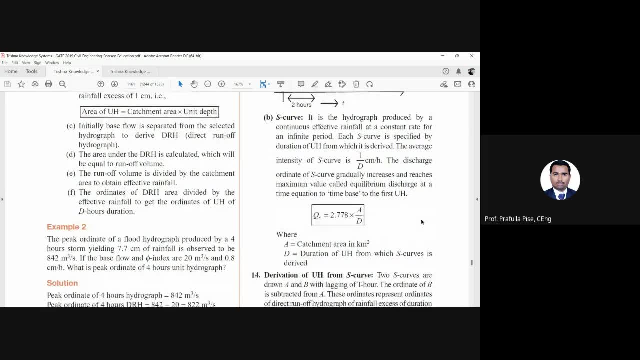 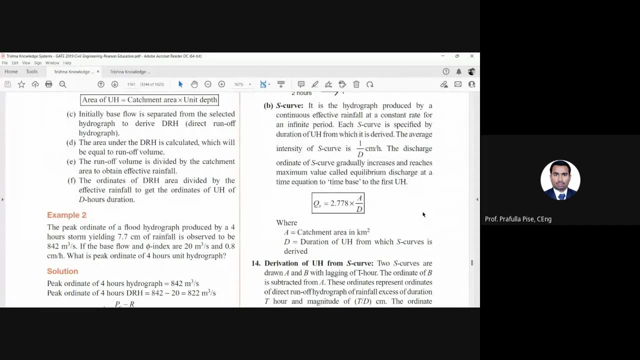 And if you superimpose the 3 unit hydrographs of 2 hours, Then we get the 1 6-hour unit hydrograph. Now S-curve, it is the hydrograph produced by a continuous effective rainfall at a constant rate for an infinite period. 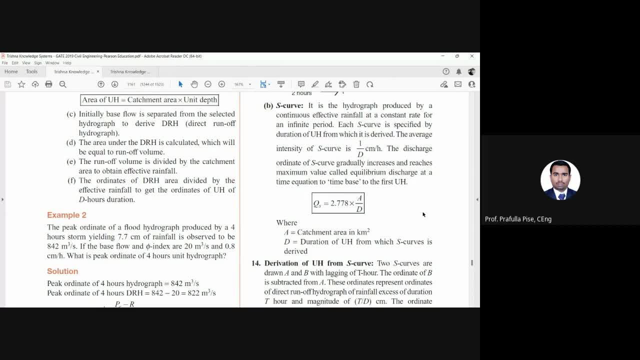 Its S-curve is specified by duration of unit hydrograph from which it is derived. The discharge intensity of S-curve is 1 over D cm per hour. The discharge ordinate of S-curve gradually increases and reaches the maximum value called equilibrium discharge at a time. equation to time base to first unit hydrograph. 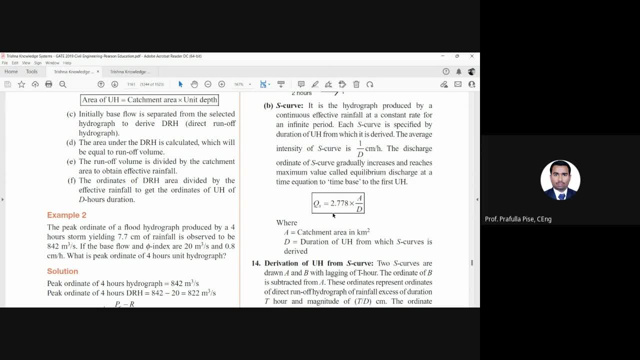 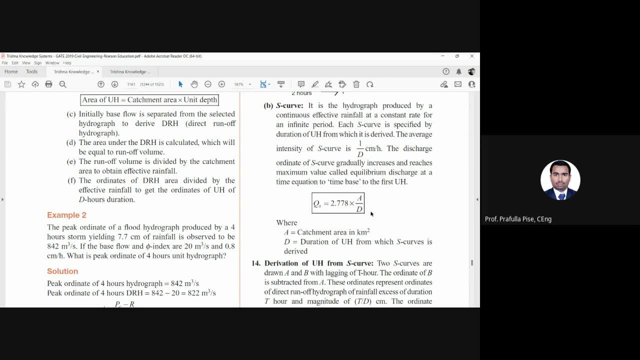 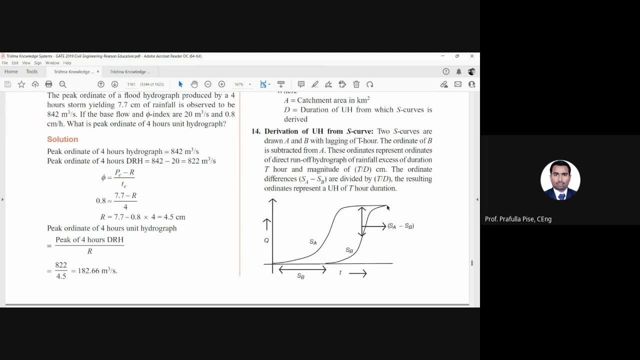 So Q is equal to 2.778 times S-curve. D is area of catchment, A is area of catchment, D is the duration of unit hydrograph from which S-curve is derived. So you can see, this is what is called as S-curve. 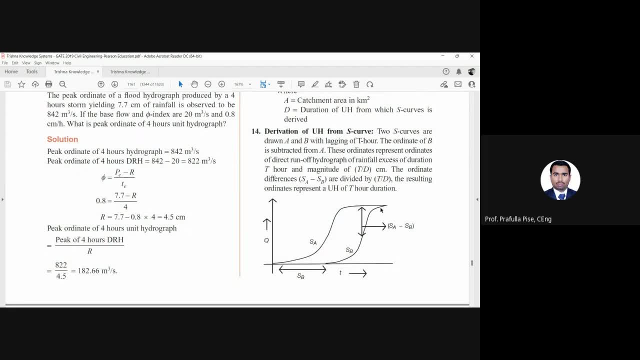 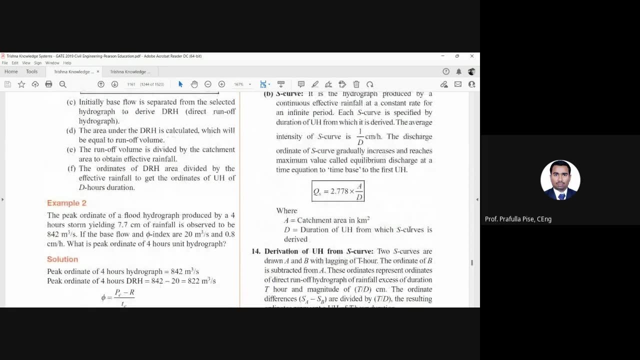 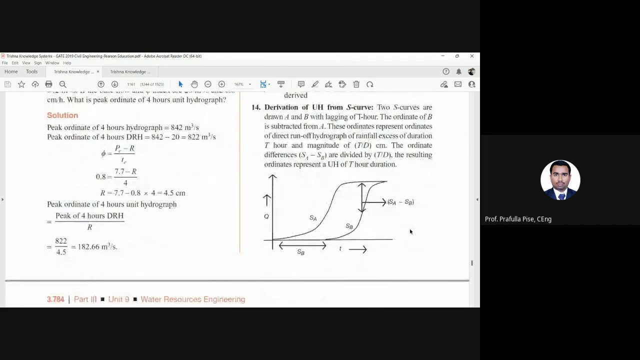 direction of unit hydrograph from s curve. two s curves are drawn: a, so this is s a and is sb with lag of t hours. okay, there is a lag of t hours. uh, the order of b is substituted from a. b is substituted from a. okay, so we can find this difference. uh, these ordinates represent: 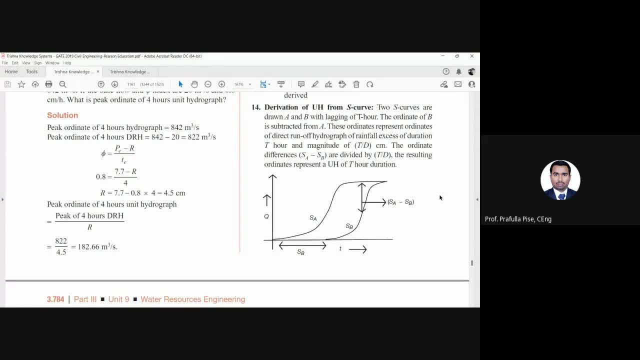 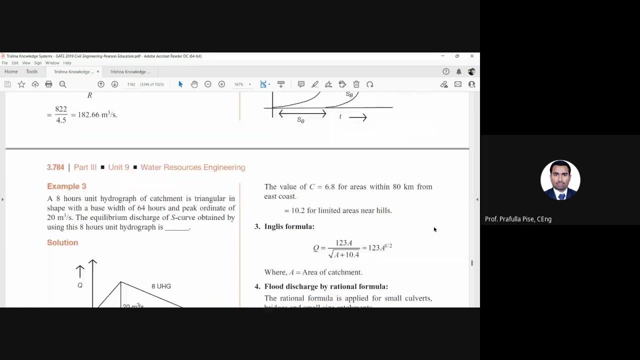 ordinate of diagram of hydrograph of rainfall, x of duration, t hour, and magnitude of t over d centimeter. so the ordinate difference s a minus sb are divided by t over d, the resulting order represent a unit hydrograph of t hour duration. we will see an example. then you will get an idea what we are talking about. 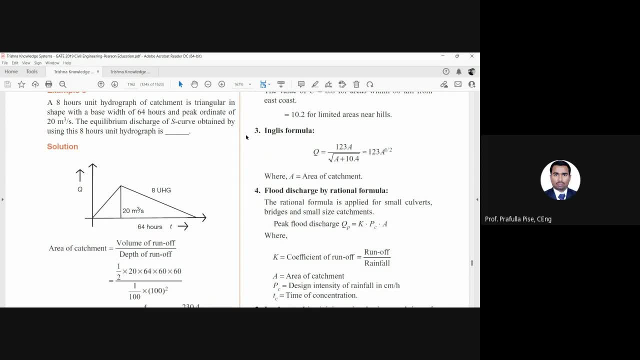 a 8 hours unit hydrograph of catchment is triangular in shape, so that's the triangular shape with best. width of 64 hours, so 64 hours, that's the best, and peak ordered of 20 meter per second, so peak is 20 meter per second. the equilibrium discharge of s curve obtained by using this eight hours unit. 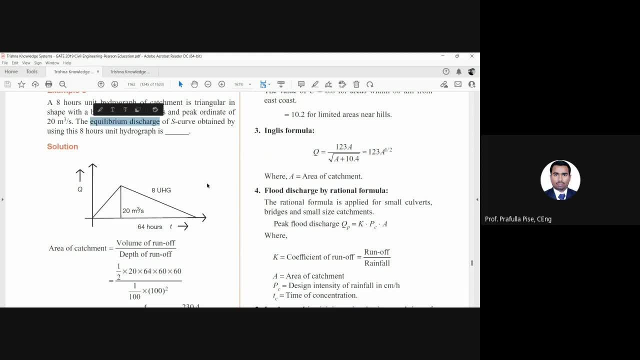 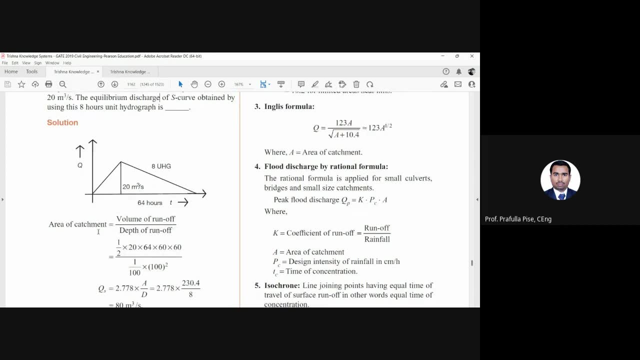 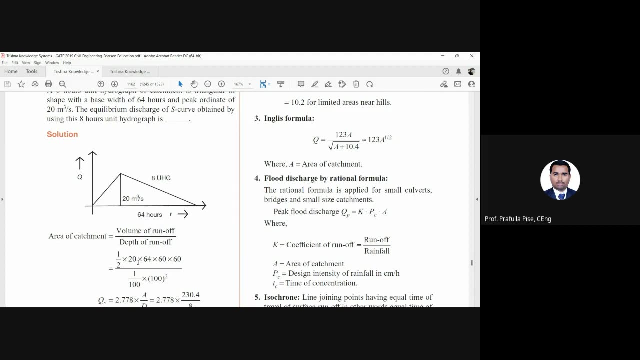 hydrograph is. so we are trying to find out the equilibrium discharge. so, first thing, what we're going to do, area of catchment, so how we can find an area of catchment. so we already know the volume of runoff which is the area of this triangle. so one half times 20 times 64 times, 60 times 60.. 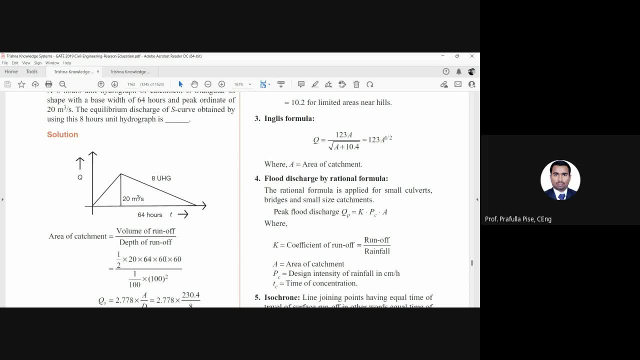 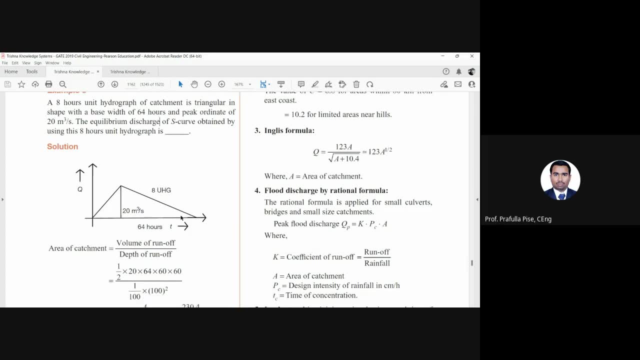 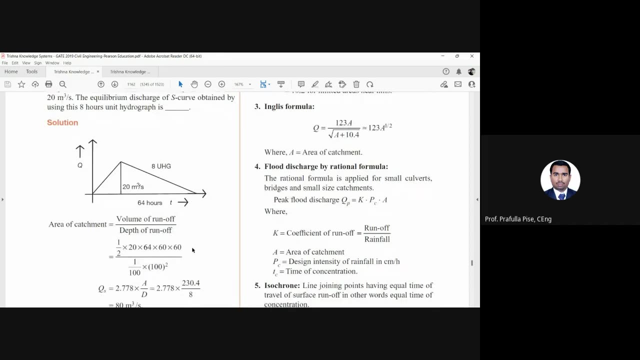 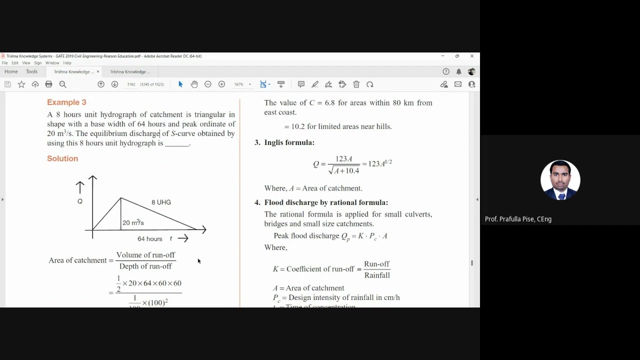 it was 64 hours, so we tried to convert into: uh, we tried to convert into seconds and, okay, the depth of runoff. so depth of runoff it's 1 over 100 times 100 centimeters square. so why they say 1 over 100? anyone have any idea why they have 1 or 100? 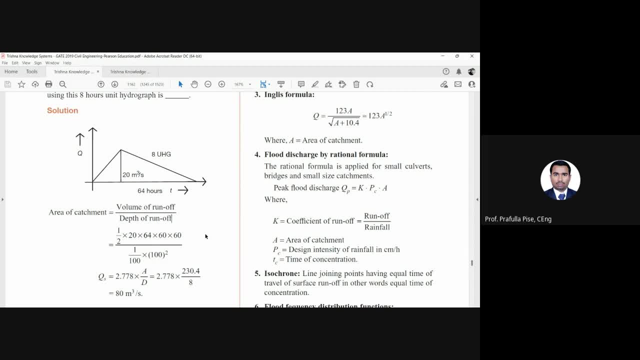 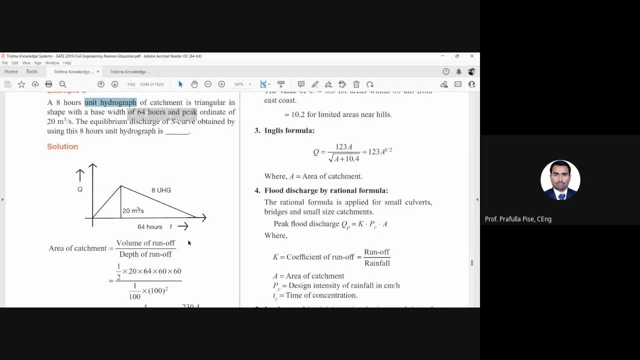 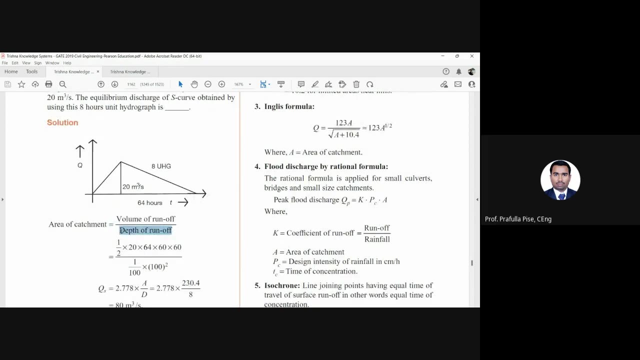 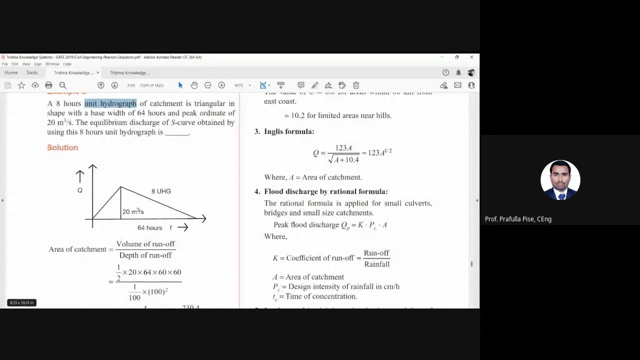 because they're talking about the depth of runoff. so, whenever they say depth runoff, since it is a unit hydrograph, since it is a unit hydrograph, so depth of runoff is one meter. depth runoff is one meter because it's a unit hydrograph. samastika. 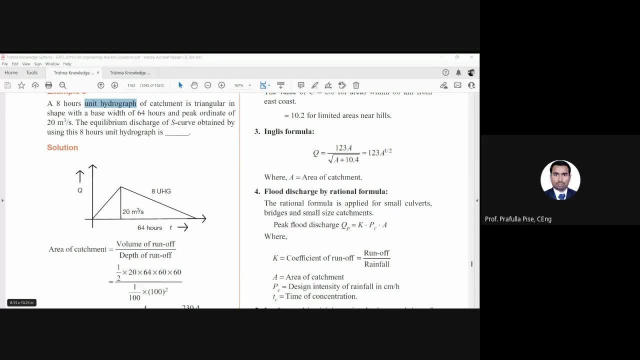 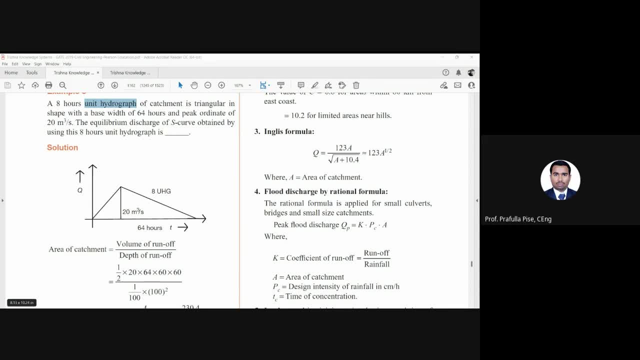 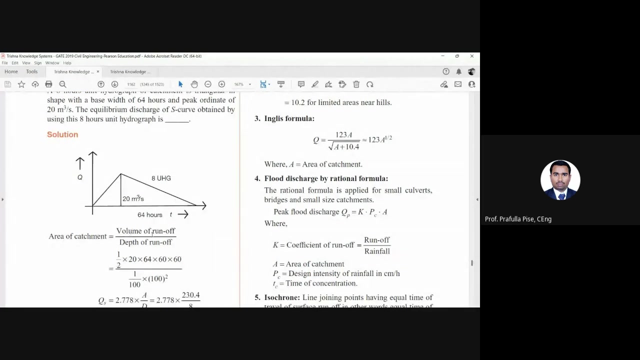 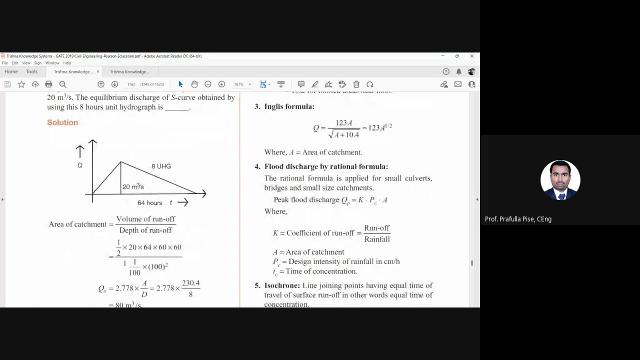 there then, is it okay? volume of triangle will give you the volume, but depth of runoff. depth runoff, because since it is a unit hydrograph, so depth is one meter. okay. so one meter divided by 100, a centimeter. okay, one centimeter, sorry, one over 100 centimeter. 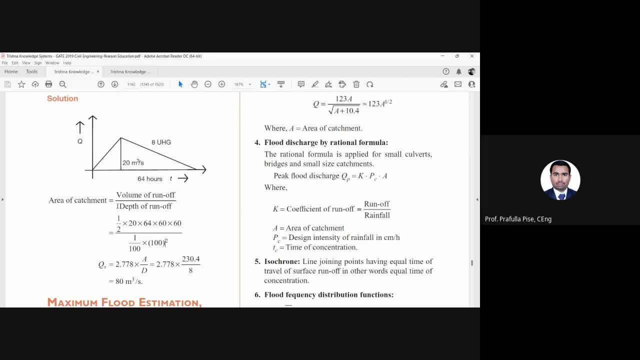 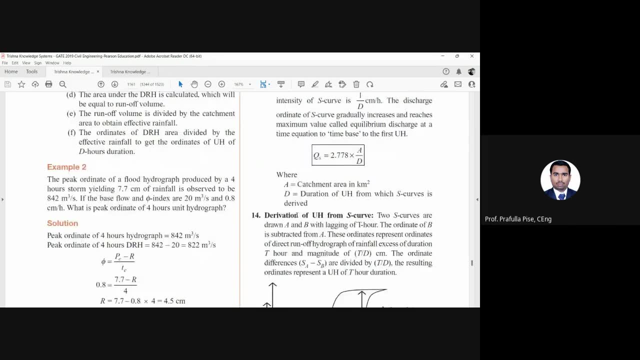 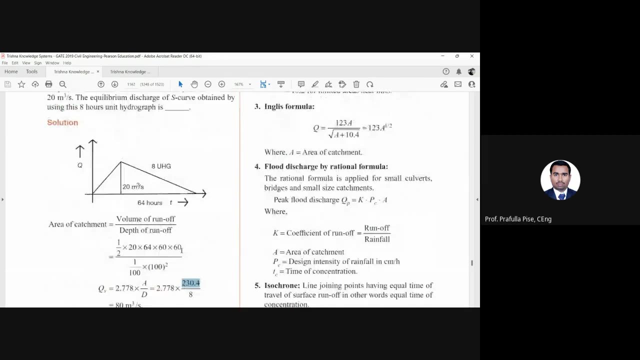 okay, this will give you the area of catchment. now, since you get the area of catchment, which will be about 230.8, okay, we are going to use the formula here, which is: qs equals to 2.778 times area over duration of hydrograph. so area, we got it right now. and since they have asked about the 8 hours unit hydrograph, 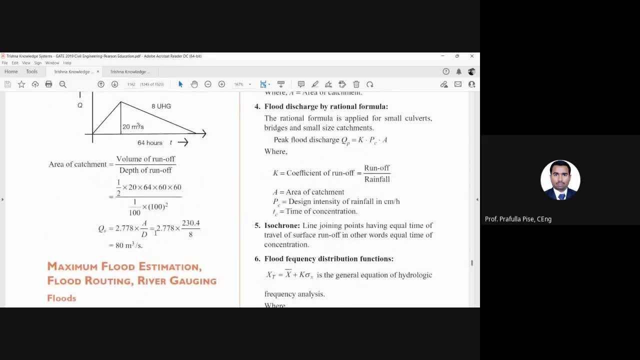 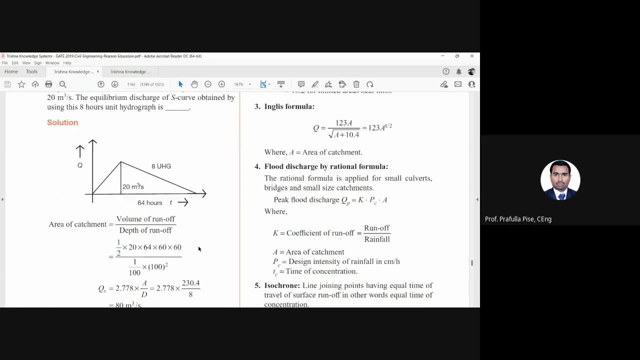 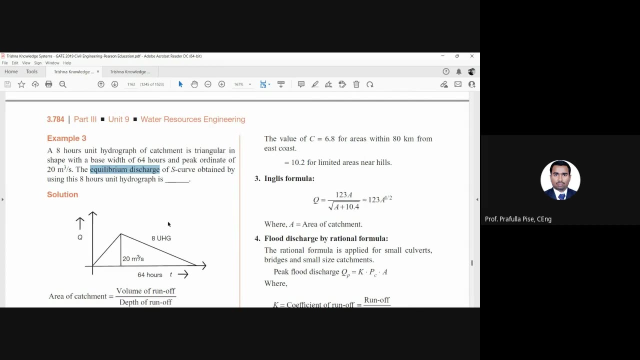 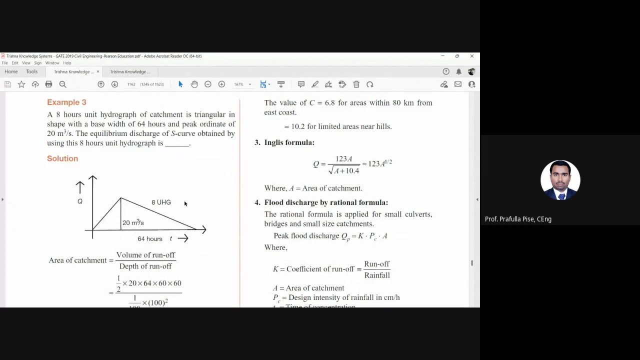 okay, so divided by 8, okay, so 2.778 times area divided by 8 hours will give you the qs. qs is nothing but the equilibrium discharge. okay, understood. now, sometimes for this type of question there will also an option. data is not sufficient, okay, a. 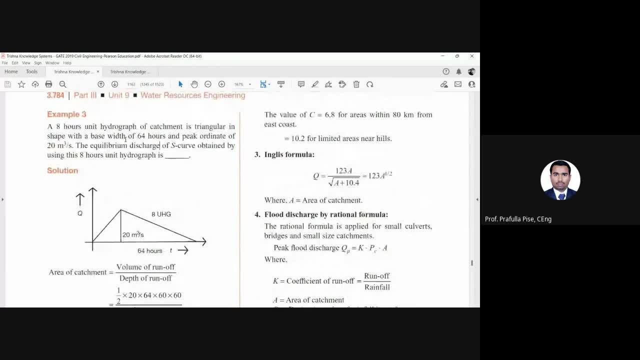 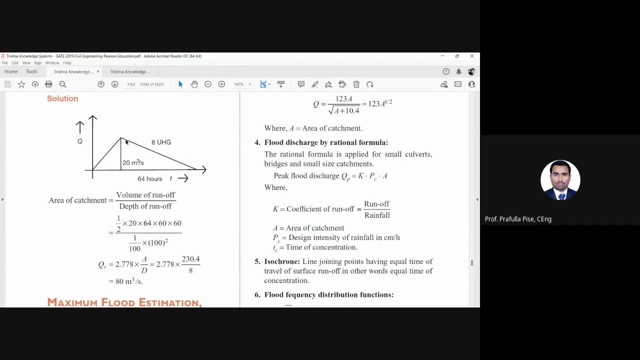 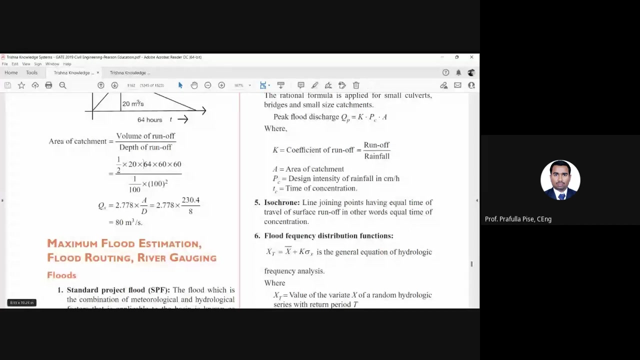 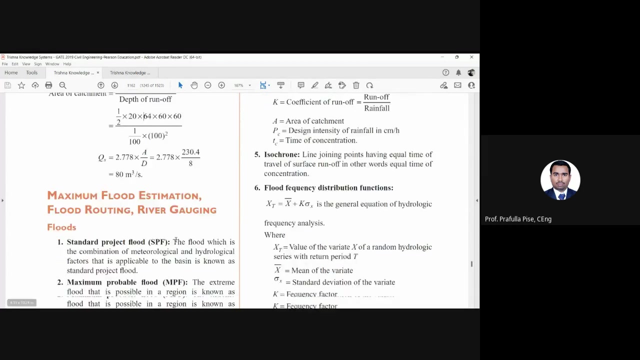 catchment is not. data is not sufficient. but you have to understand they have said unit hydrograph. that means they have given us the depth of runoff. keep this in mind. sometimes in options, data is not sufficient. that is not the answer now. next is maximum flood estimation. 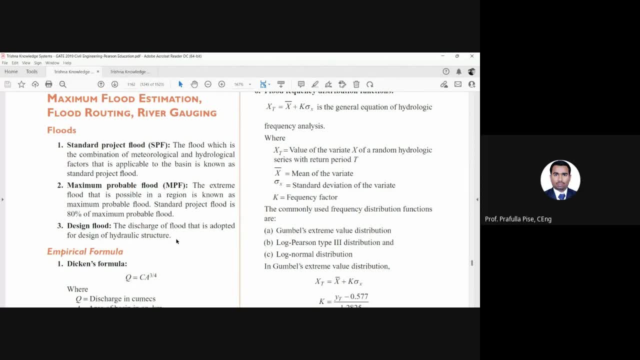 flood routing, river gauging floods, standard project flood- SPF. the flood, which is the coverage of meteorological and hydrological factors that is applicable to the basin, is known as standard project flood- maximum probable flood. that is something which we always work on. we work on this. 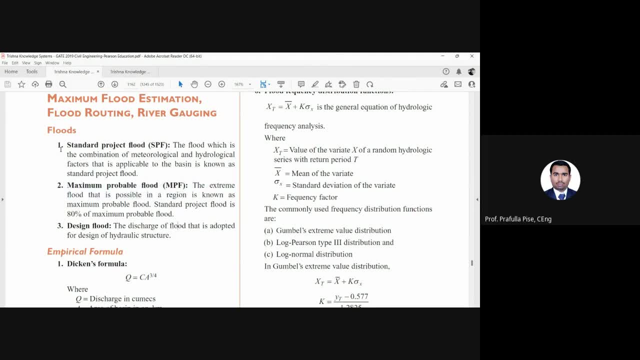 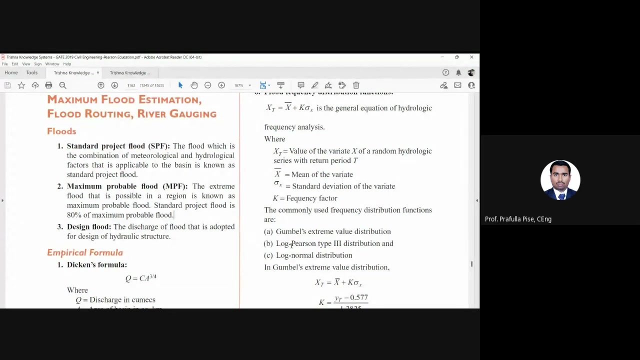 maximum probable flood. we rarely work with standard project flood. ok, when you start a job. when you start a job in real life, we use standard project flood. but in academic life, when you are a student or in college, ok, then we use maximum probable flood. ok, we are going to use this term. 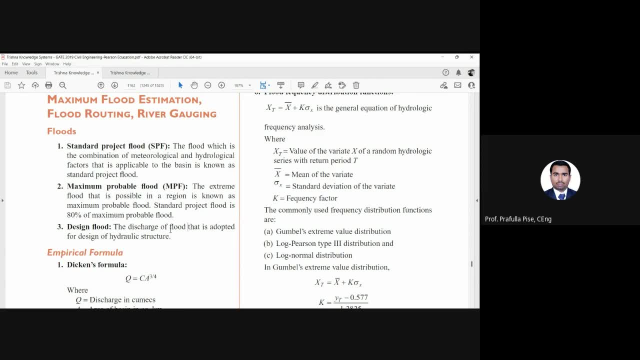 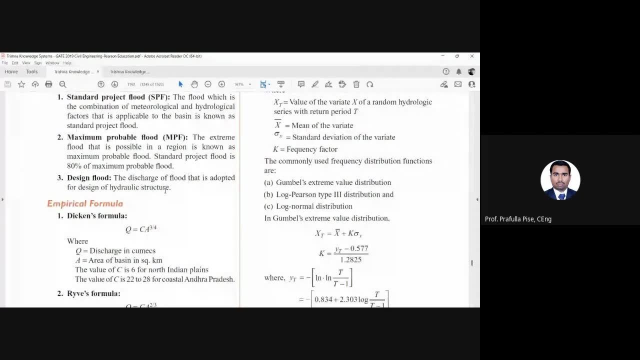 the extreme flood that is possible in region is known as maximum probable flood. standard project flood is 80% of the maximum probable flood, and then design flood. ok, this is something. design flood: you will always get in your problem statement. when you get a question, then we already. 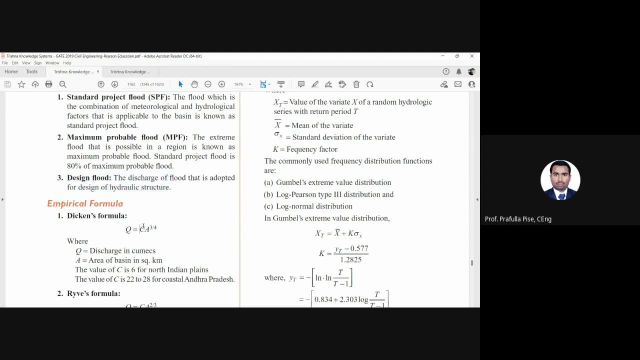 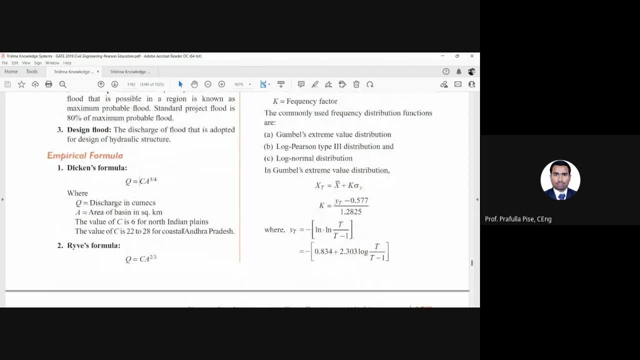 define. what is the design flood? ok, you don't have to calculate now. there are so many different formulas. ok, formula Dickinson, formula Q equal to CA over Q is the discharge increments. here is the area of basin C is 6 for north indian plains and 2228 for. 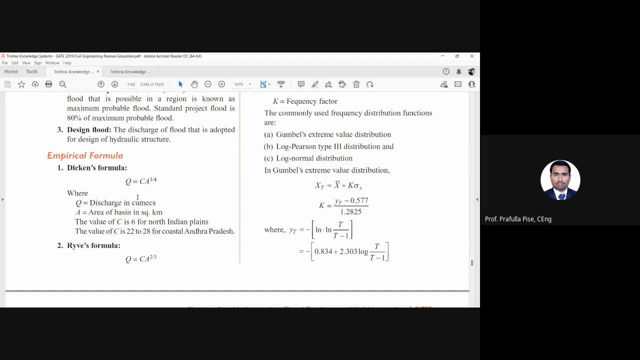 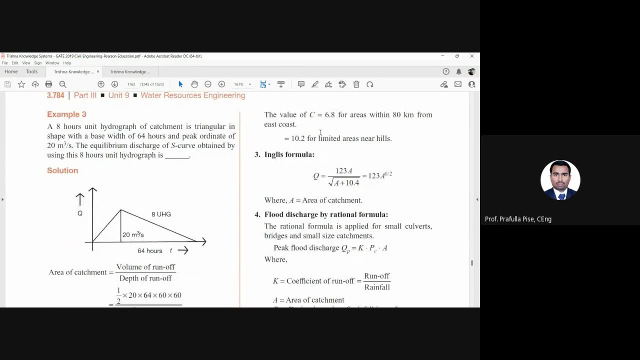 coastal Andhra place. ok, so that is the Dickinson formula. then Reeves formula Q, equal to C area to power 2, third. so the volume of C is 6.8 for areas within 80 kms from the east coast, 10.2 for limited areas near hills. 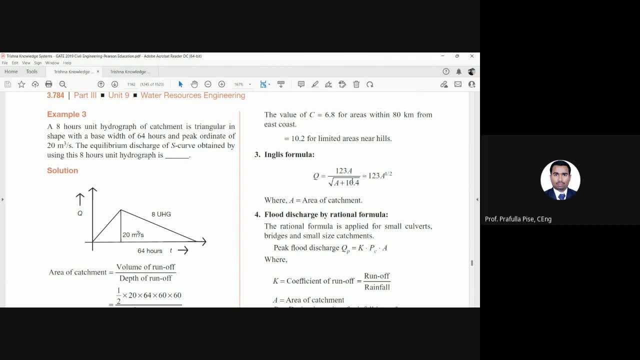 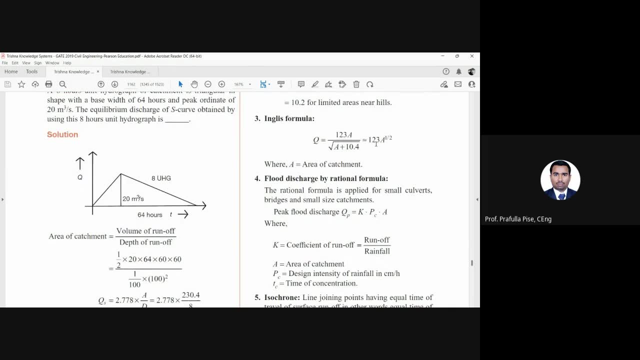 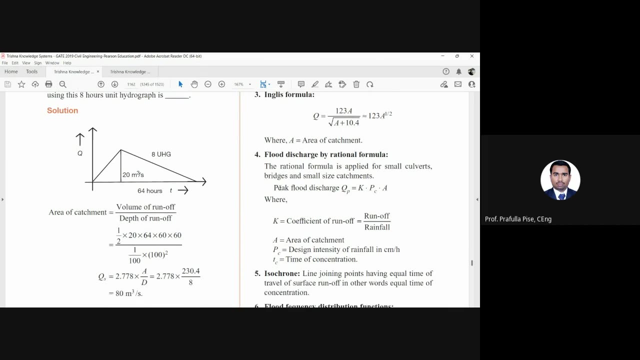 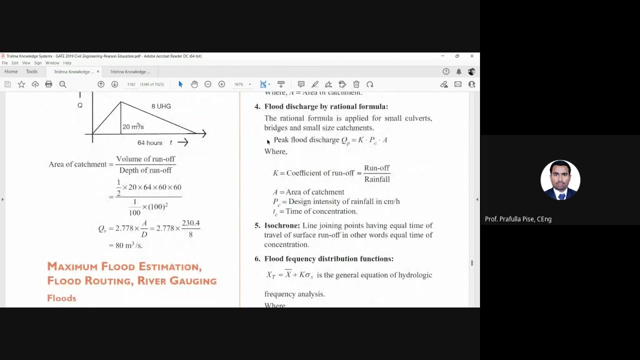 then English formula Q, equal to 123A over square root of A plus 10.4, which is nearly equal to 123A times A to the power one half flood discharge by rational formula. that is most used. rational formula is applied for small culverts, bridges and small size catchment. 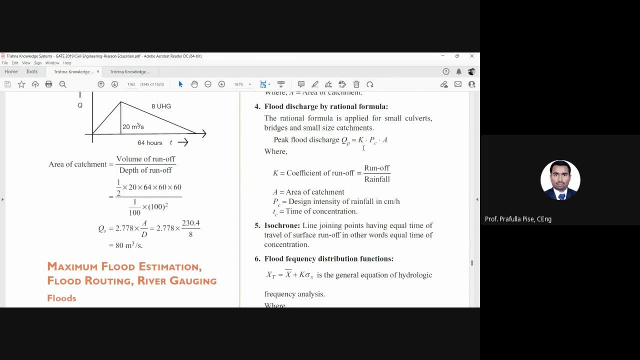 peak flood discharge. Q equals to KPC as a KPA, so K is coefficient of runoff, runoff over rainfall, A is the area of catchment, PC is density design intensity of rainfall in cm per hour and TC is time of concentration. don't worry, we are going to work on problems. 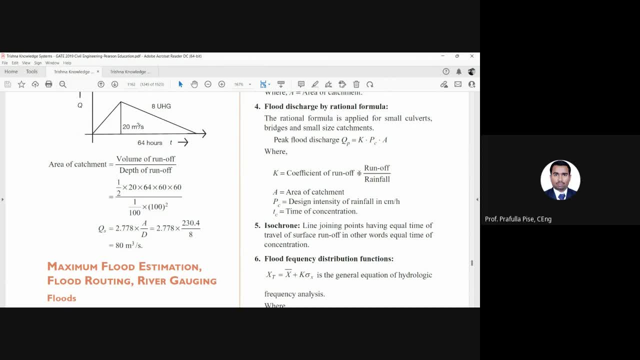 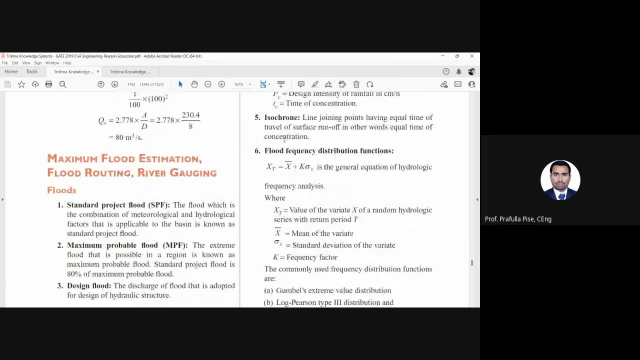 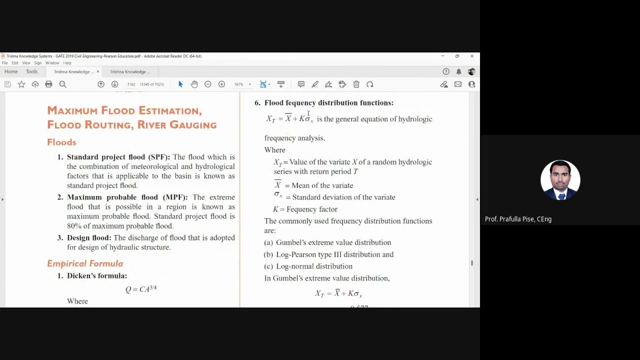 using the rational formula. ok, because that is the most popular, most used formula in India. isochrone line joining points having equal time of travel of surface runoff in order. in other words, equal time of concentration. flood frequency distribution in fluxion. flood frequency distribution functions Xt equal to X bar minus. 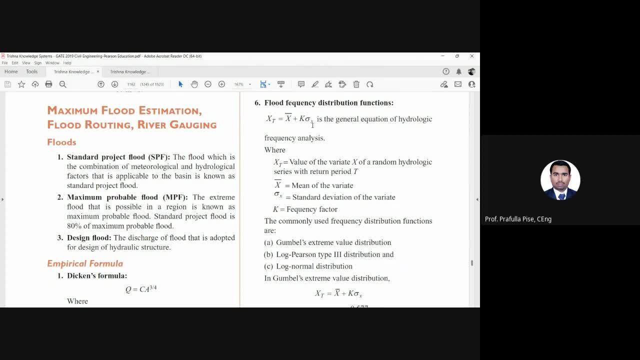 K times plus K times sigma X. so what is Xt, the value of Xt? so we can calculate X of random hydrologic series with return period of T. so T is the return period, X bar is mean sigma, X is standard deviation and K is the frequency factor. 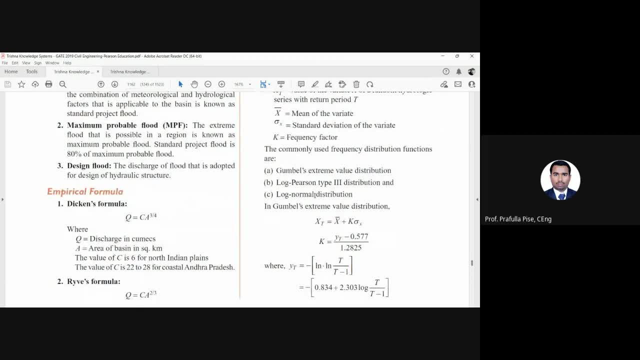 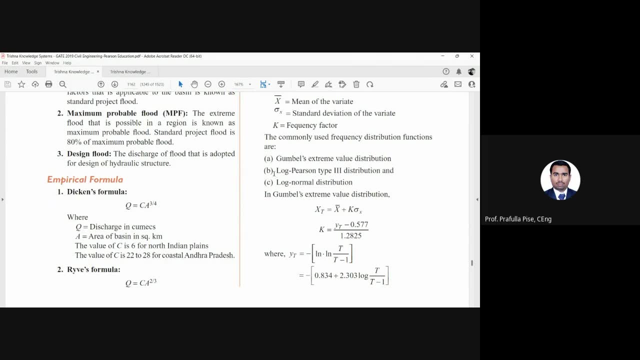 now we have different frequency distribution functions: Gumbel's extreme value distribution, log Pearson type 3 distribution and log Pearson type 3 distribution, log normal distribution. in Gumbel's extreme value distribution the formula is: Xt equals to X bar plus K sigma X. so the value of K is given by 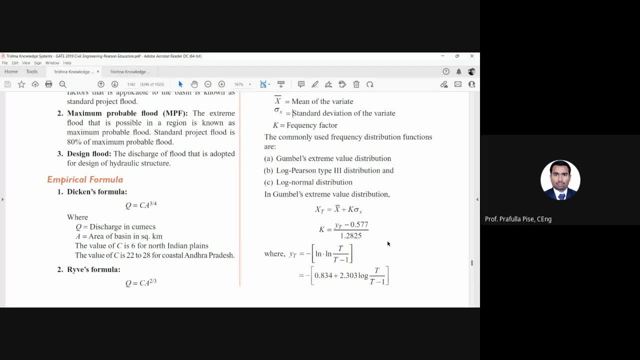 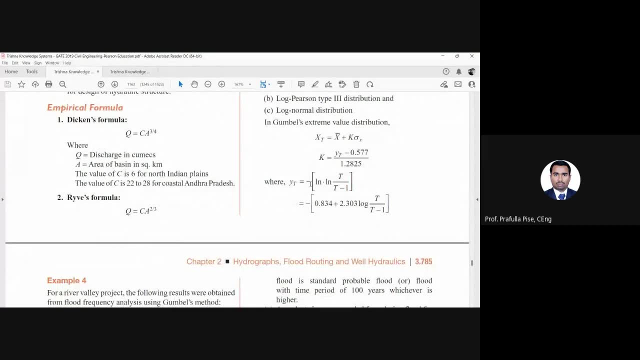 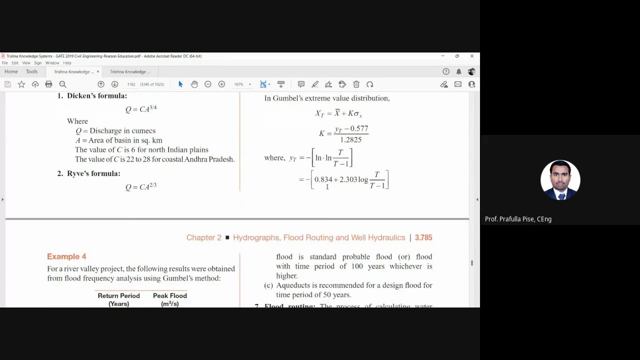 Gumbel's extreme value distribution is: Yt minus 0.577 over 1.2825, where Yt equals to negative natural log of T over T minus 1, which equal to negative 0.834 plus 2.303 log. this is the 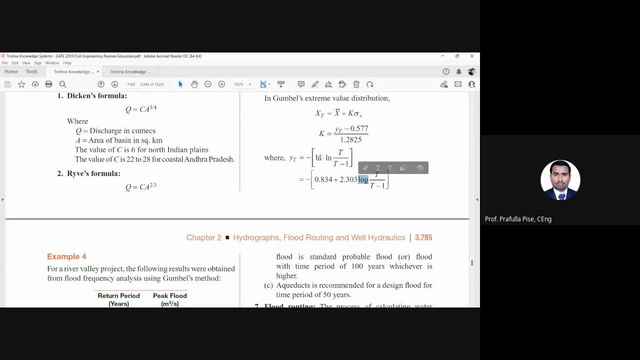 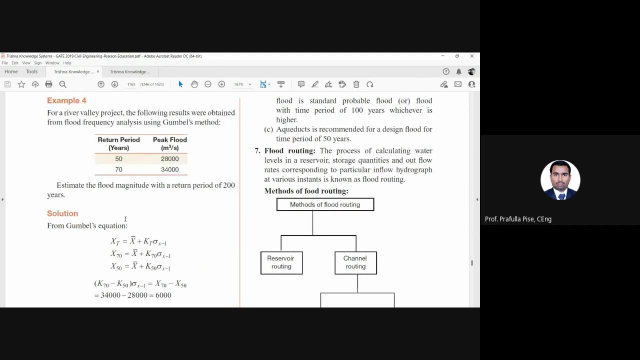 log 10. this is the natural log. so log base E, log base 10, T over T minus 1. now we will see the example for a required value project. the following results were obtained from flood frequency analysis using Gumbel's method. so return period 50. 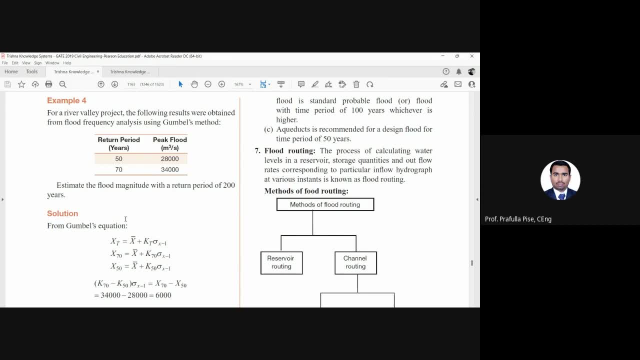 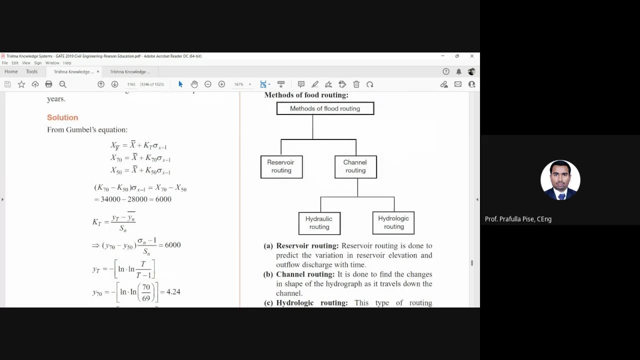 the peak flood is 18000 m3 per second and return period 70. the peak flood is 34000 m3 per second. estimate the flood magnitude with the return period of 200 years. so from the equation we know, Xt equals to X bar plus Kt sigma. 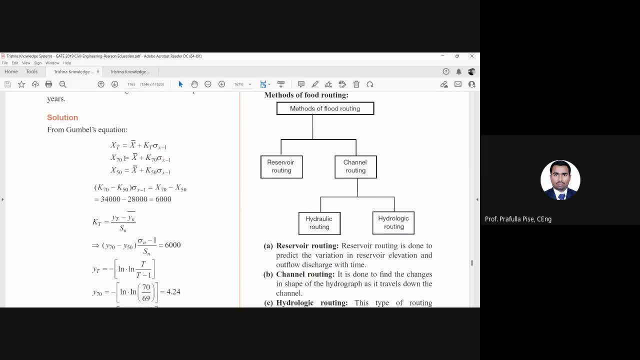 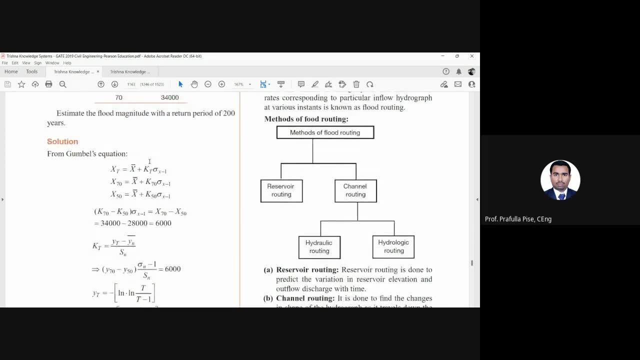 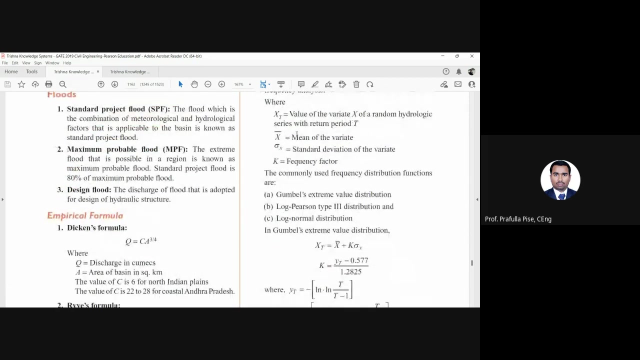 X minus 1, so they have given us X17, X50- ok. they have also given us- or we can find out- K70 and K50- ok, so they have not given us the X bar. X bar is mean of variate, so we don't have mean. 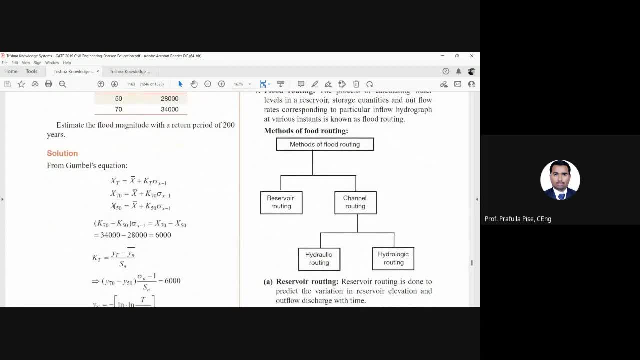 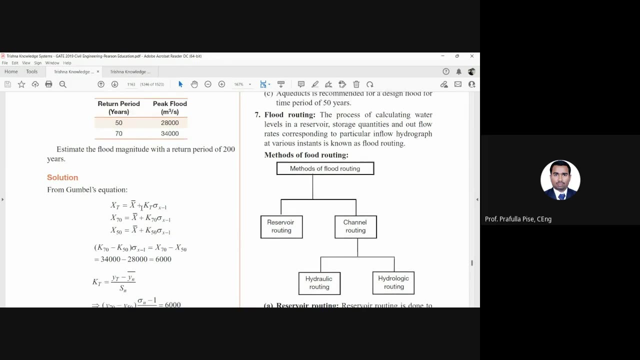 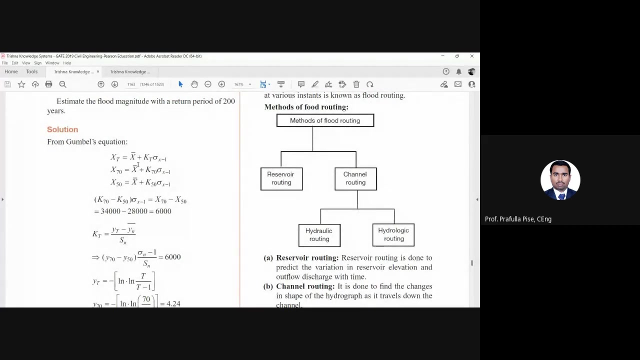 so we are going to subtract X70 minus X50 to get rid of this X bar. let's say: then we have mean mean or mean what we are going to do. we are going to use two equations to get rid of the X bar and use the. 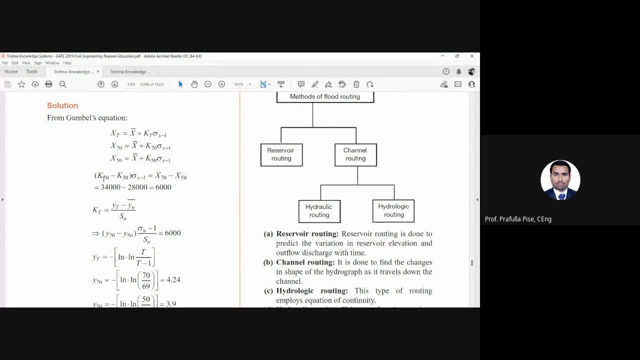 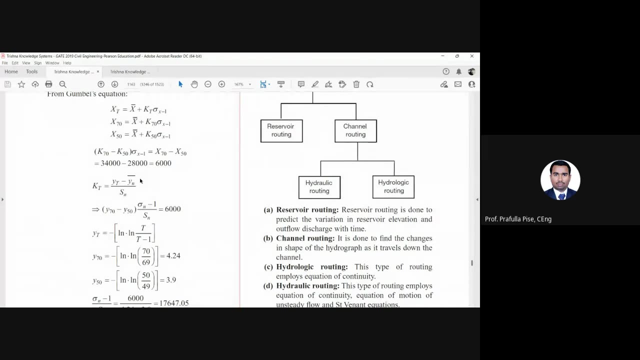 to find out the sigma X minus 1, so you can see: X70 is 34000, X50 is 28000, so difference is 6000. ok, so Kt equals to Yt minus Y, bar n over Sn. so Y70 minus Y50. 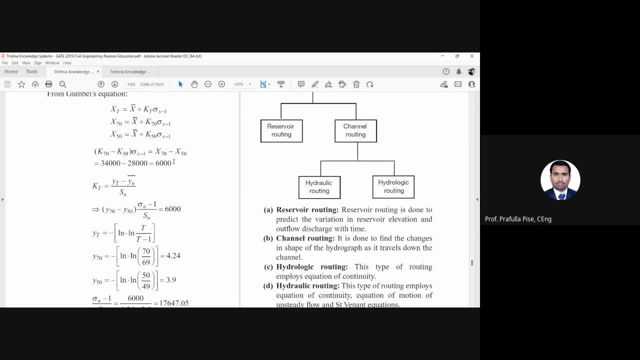 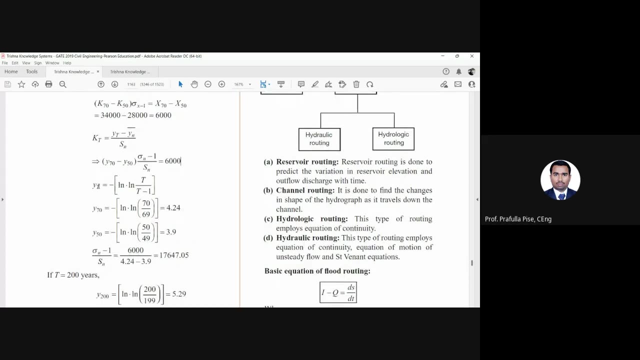 times sigma n minus 1 over Sn 6000. so we have one equation here and another equation here. so using these two equations we are going to solve for the sigma n. so Yt equals to again negative double natural log of T over T minus 1. 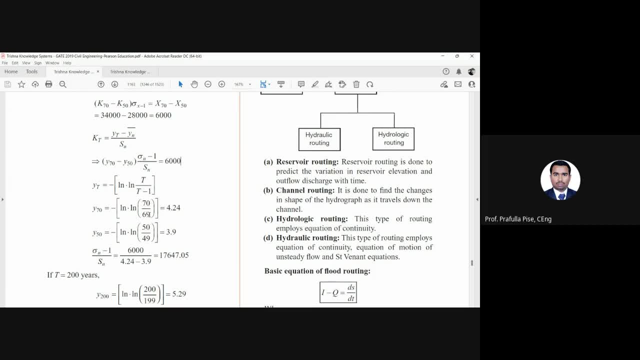 ok, so T it is 70 T minus 1, 69. same T: 50 T minus 1, 49. ok, so we can get the Y17 Y50. so if you substitute this Y17 Y50 in this equation, you get sigma n minus 1 over Sn. 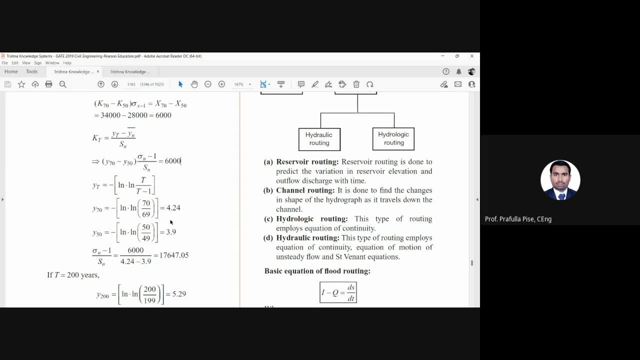 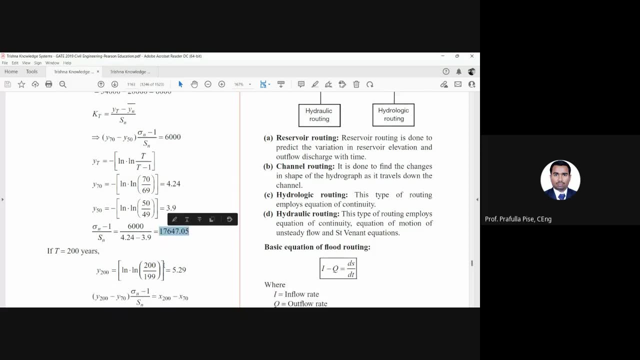 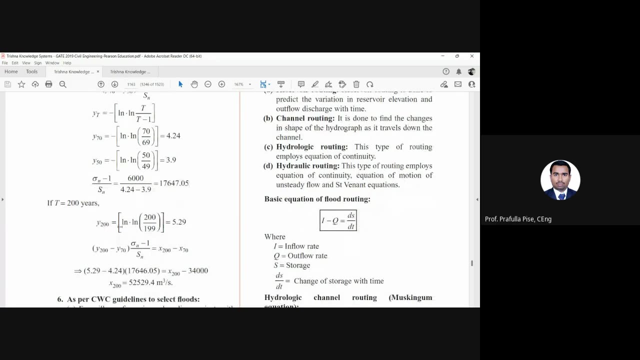 which is equal to 6000 divided by this 4.254 minus 3.9. we got this equation now, for the T equals to 2000 years. Y2000 equals to double natural log of 200 divided by 199, so it will give you 5.29. 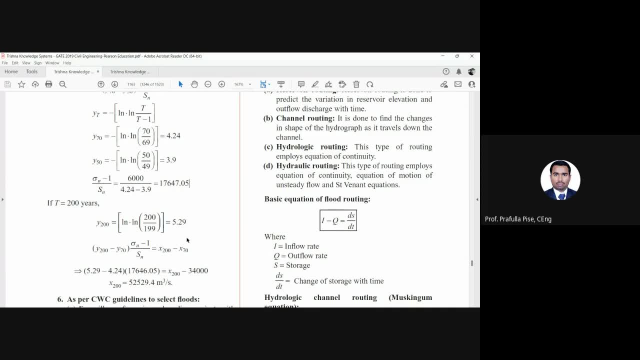 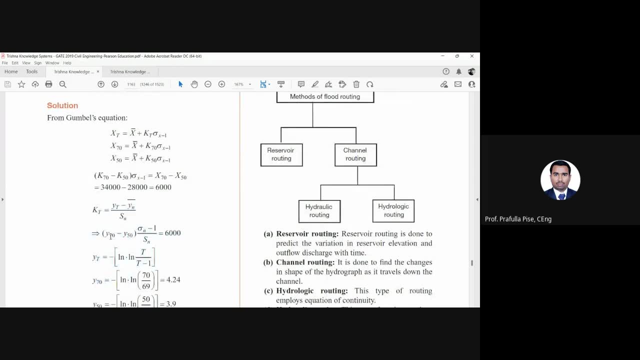 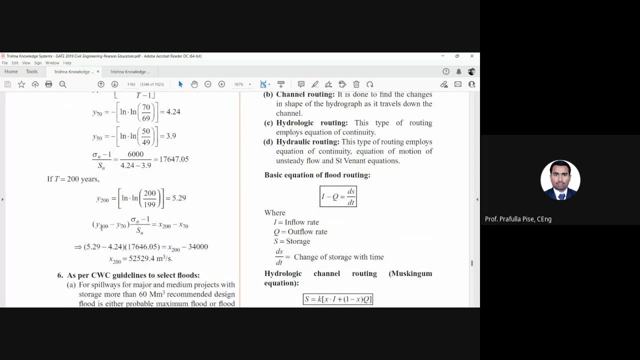 ok, so again we go back to the equation this, but instead now we have Y17, Y50, we are going to use Y200 and Y70. so Y200 minus Y70 times sigma n minus 1 over Sn equals to X. this should be capital X. 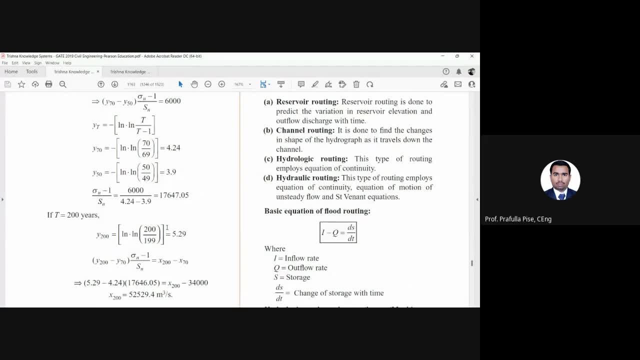 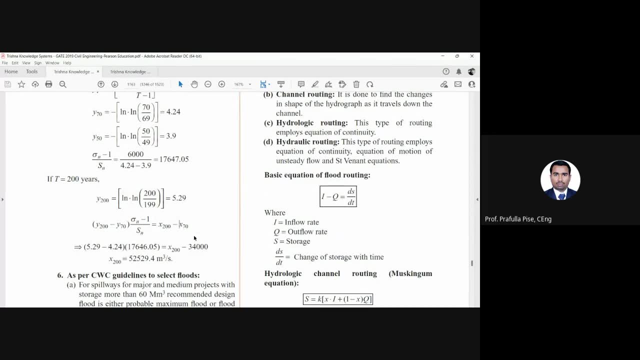 capital X, this one. this is not the small x, remember, this is the capital X, so capital X200 minus capital X70. ok, so if you try to solve that, you can find out the X200 capital X200. ok, so this is the 52529 point 4. 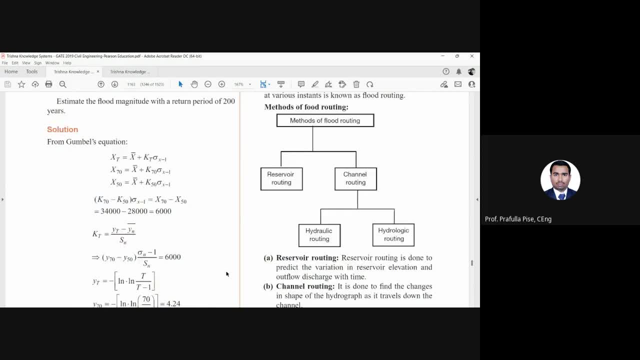 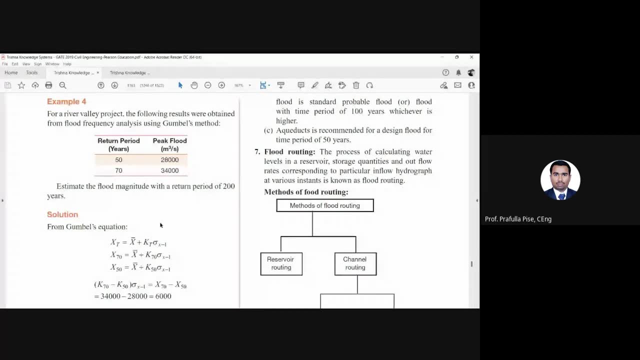 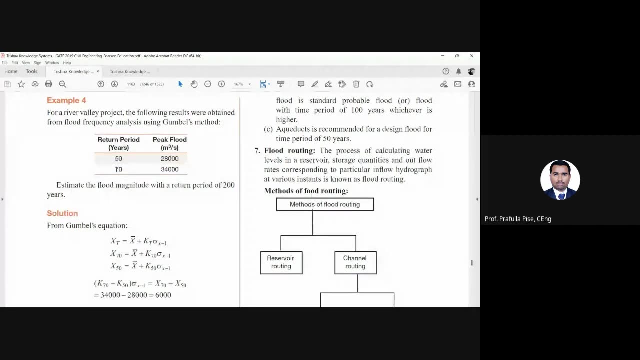 meter cube per second. now, since they have not given us any options here, it is difficult to find the answer. you have to do the calculation. but remember: for 50 years is 28000, for 70 years is 34000, so obviously for 200 it should be more. 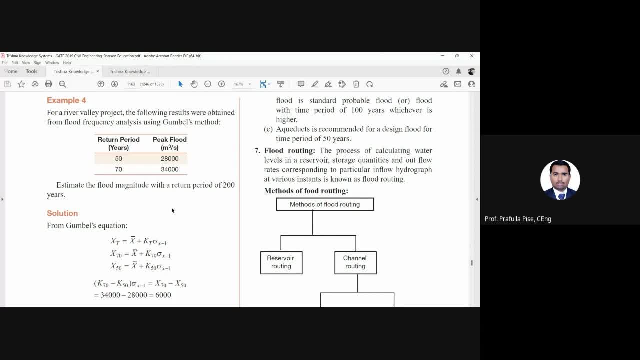 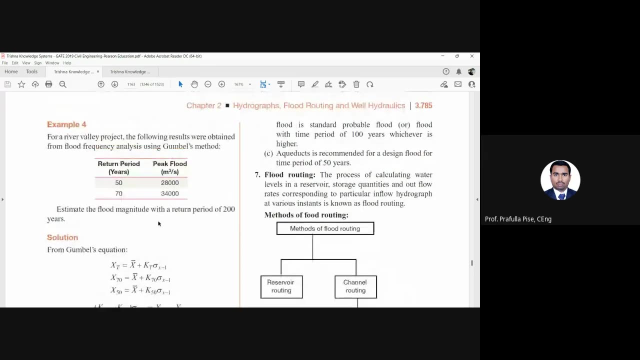 than 34000. that is logic you can use. ok, you cannot use ah. or if you don't have time to do the calculation, ok, you can use this other ah logic, ok. so what we can do, take the ratio: ok, suppose 50 is 38000, 70 is. 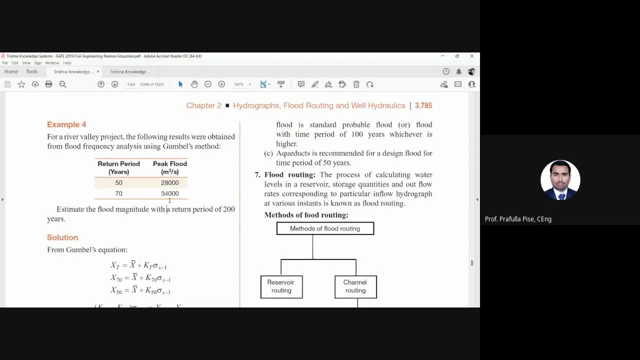 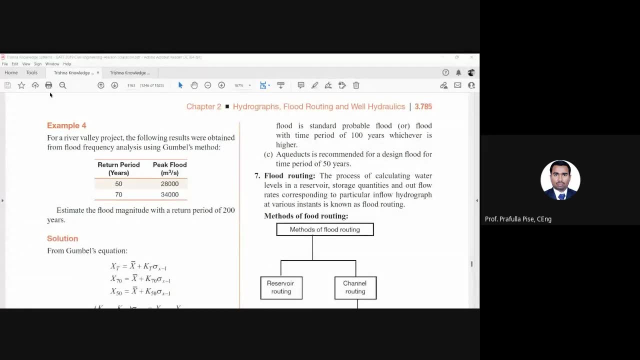 34000, so how much is 200? generally we do cross multiplication. suppose we do it like that, what happens? ok, ok, so what did you do? suppose, ah, ah, ah, ah. 20 years increased. so how much we increased? ah, 34 minus 28, 6000. 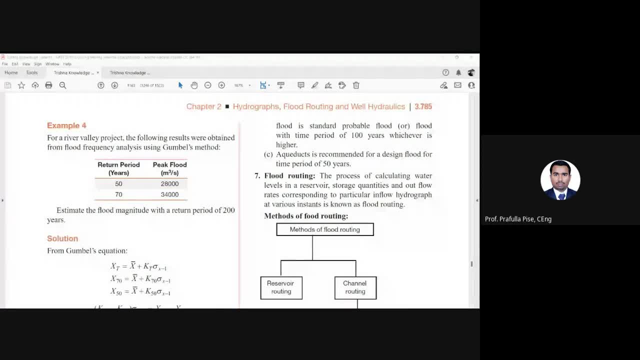 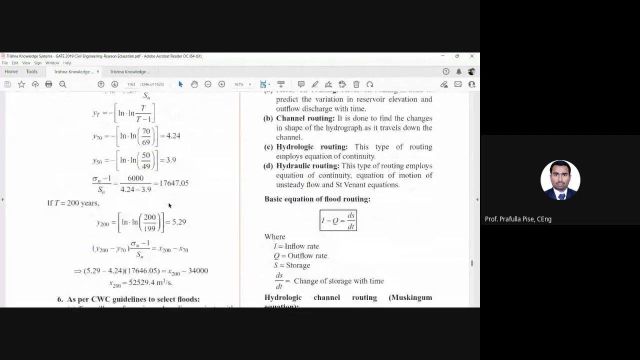 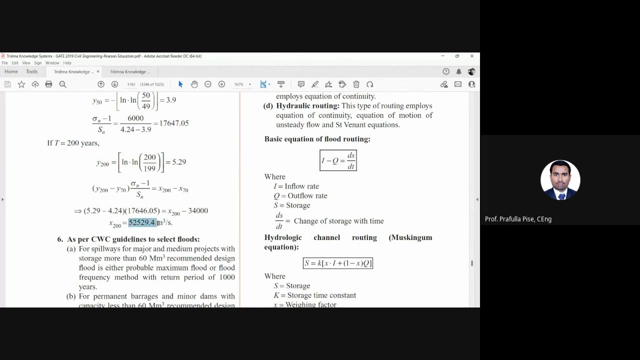 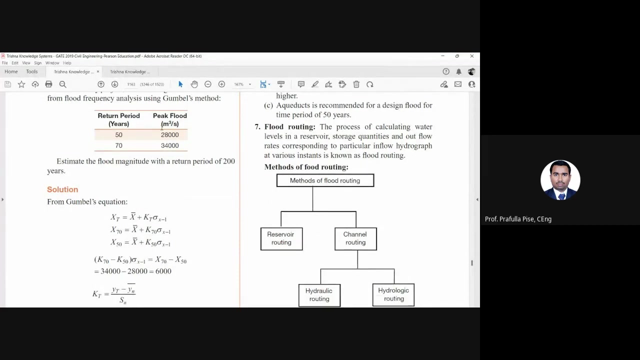 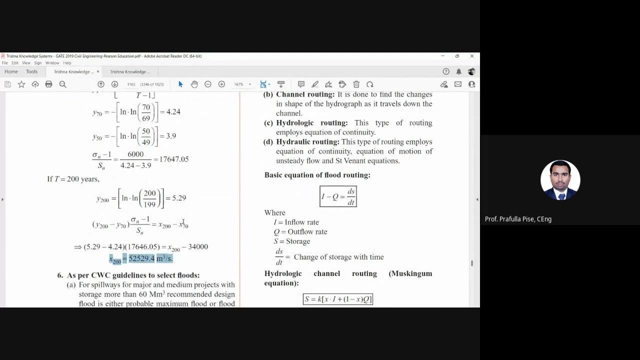 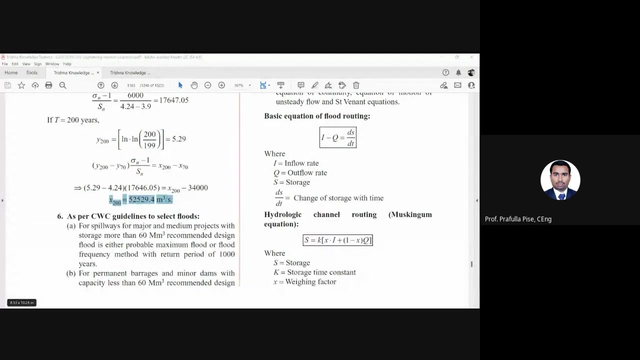 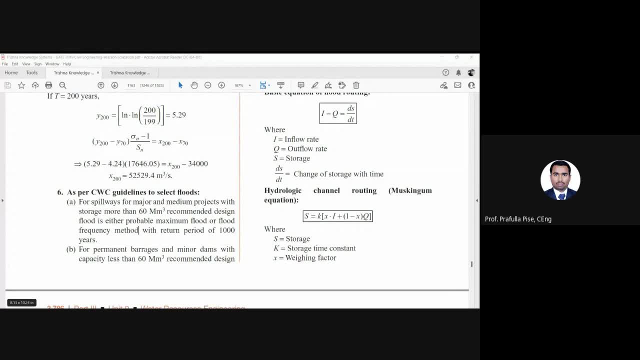 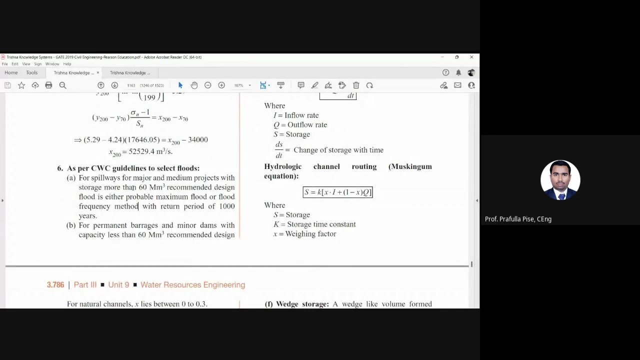 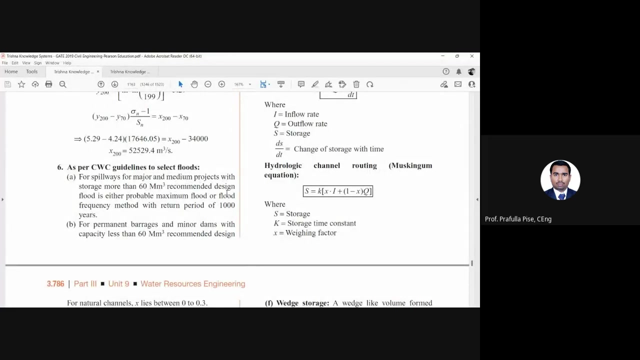 question the question problem. Can we move on to the next slide? As per the solution guidelines to select floods For spillways for major and medium projects with storage more than 60 million m3, recommended design flood is either probable maximum flood or flood frequency method with return period. 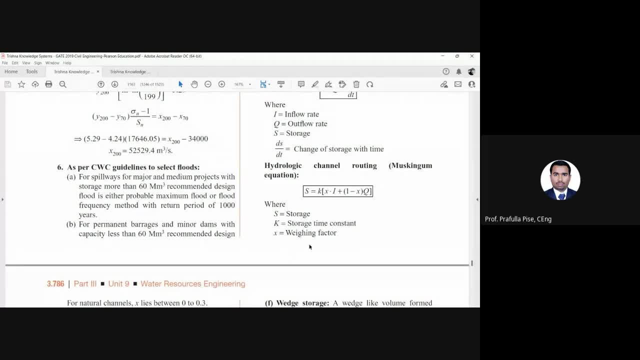 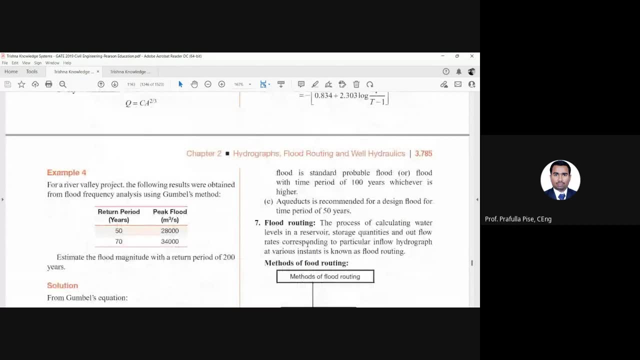 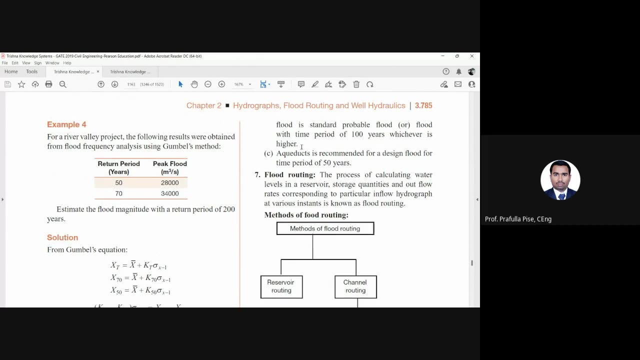 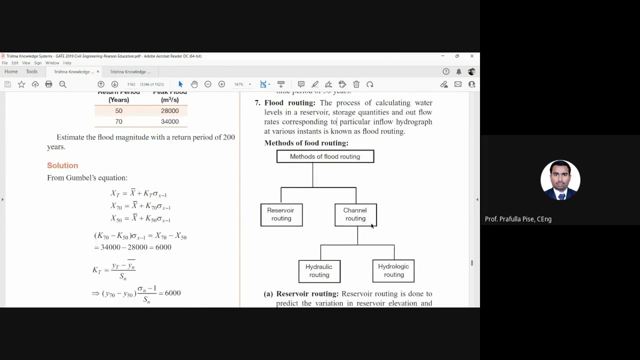 of 1000 years For permanent barrages and minor dams with capacity less than 60 million m3. recommended design flood is standard probable flood or flood with time period of 100 years, Whichever is higher. Aqueducts is recommended for a design flood for time period of 50 years. 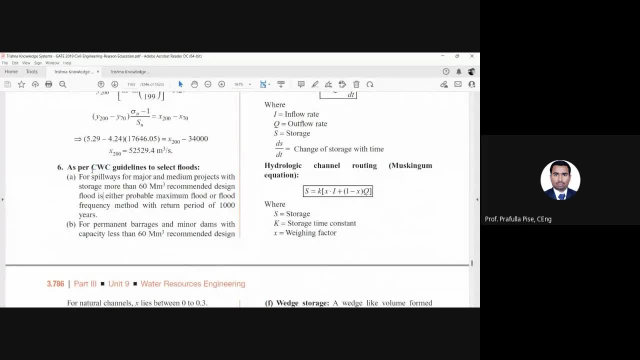 You understand what is SUDOSU right. SUDOSU is Central Water Commission, Delhi. That is the autonomous body of Government of India which controls or which monitors the water flow. SUDOSU SUDOSU In India. 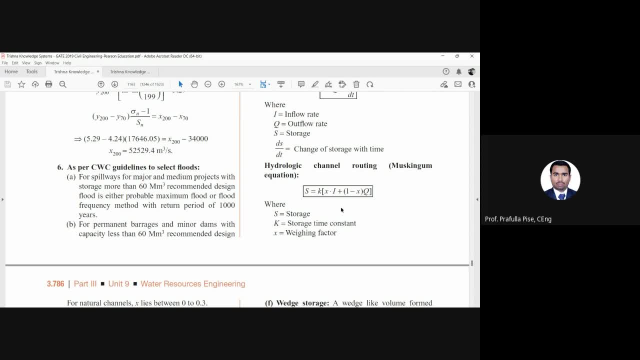 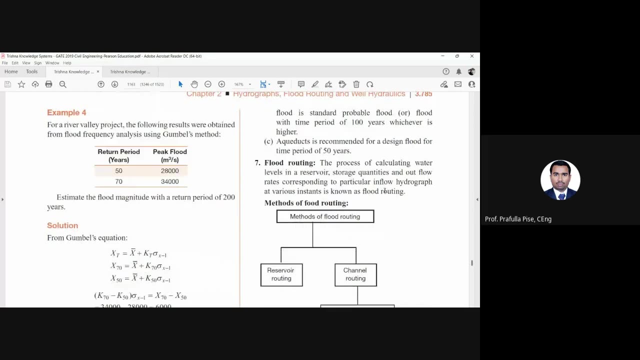 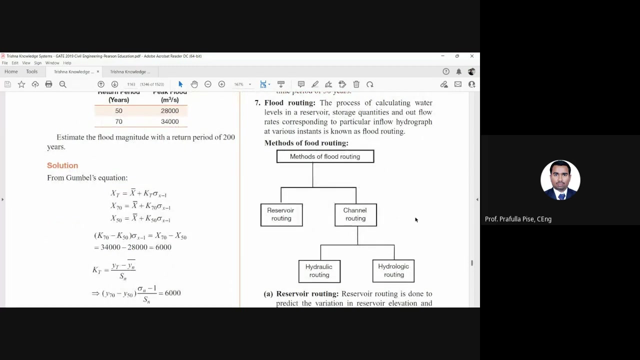 Okay, When there is an interstate involved or more than one state involved. okay, that is something which comes under the CWC Flood Routing: The process of calculating water levels in a reservoir, storage quantities and outflow rates corresponding to particular inflow. hydrograph. 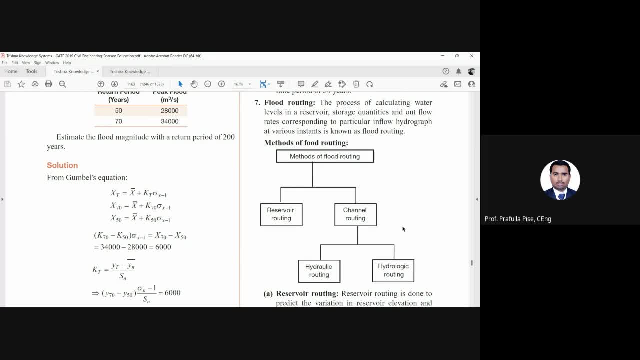 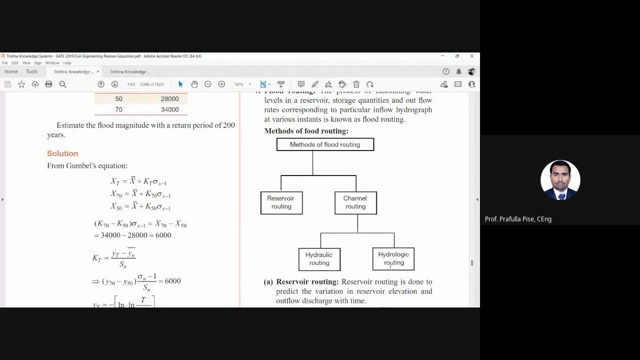 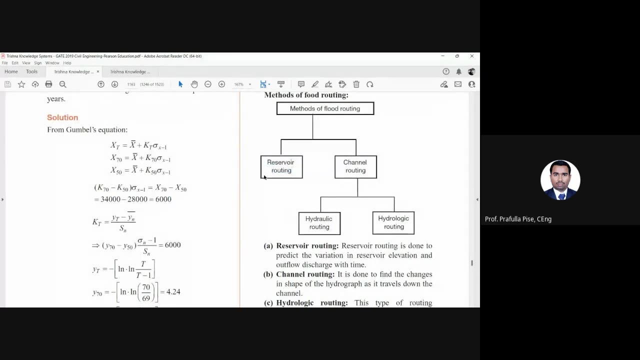 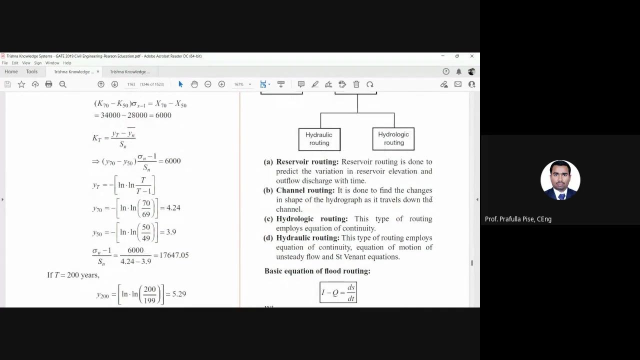 graph at various instant is known as flood routing. so methods of flood routing: reservoir routing, channel routing. so hydraulic routing and hydrological routing. most of times we use the reservoir routing. okay, for the flood routing. this is our routing. is done to predict a variation in reservoir elevation and outflow discharge with. 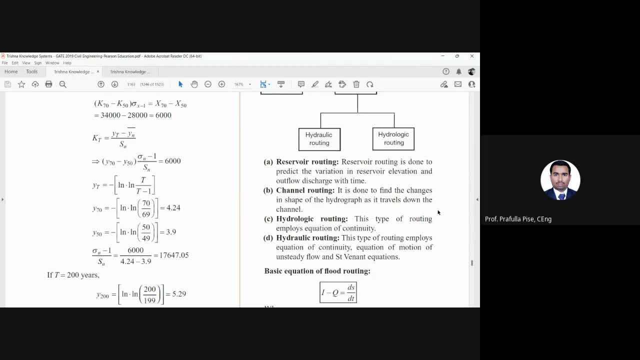 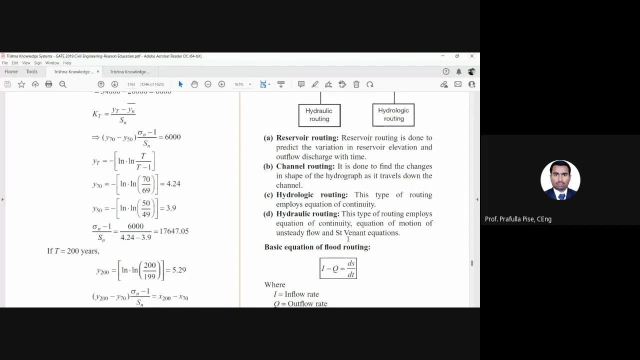 time. the channel routing. it is done to find the changes in shape of hydrograph as it travels down the channel. hydrological routing is the type of routing employs equation of continuity and hydraulic routing. this type of routing employs the equation of continuity. equation: motion of unsteady flow and scent: imminent equation. 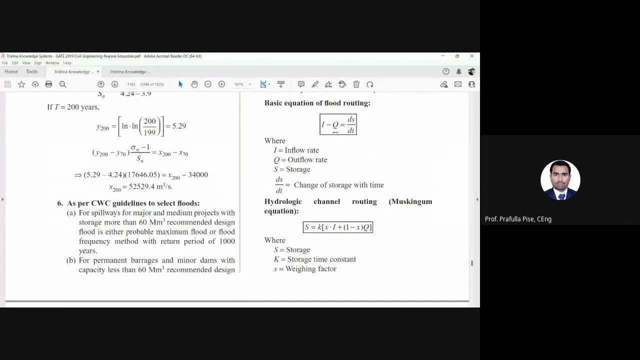 so the basic equation of flood routing is I minus Q, equal to DSVDT, where I is the inflow rate, Q is the outflow rate, S is the storage and DSVDT is change of storage with time. remember, this is rate, so in flow, okay, there is also rate when we say rate, so it is always respect to time. 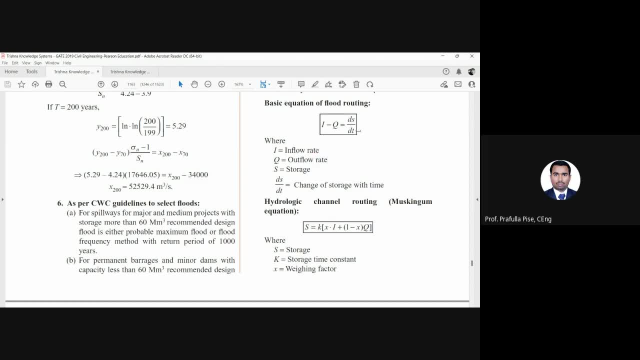 so there is a divide by time. okay, that's why we can make an equation. this is also ds over. dt means divided by time. otherwise it's going to be difficult to do the calculation. hydraulic channel routing- ah, must england. equation X equals to K times in the bracket, X times I plus. 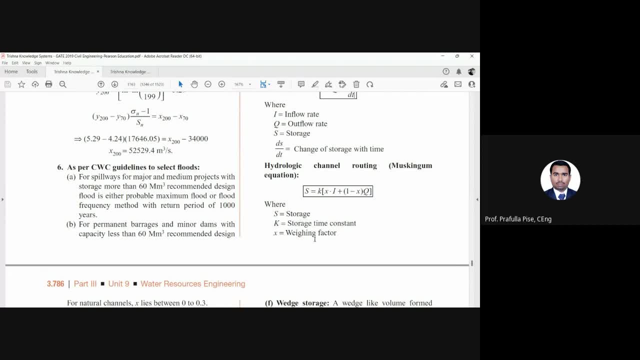 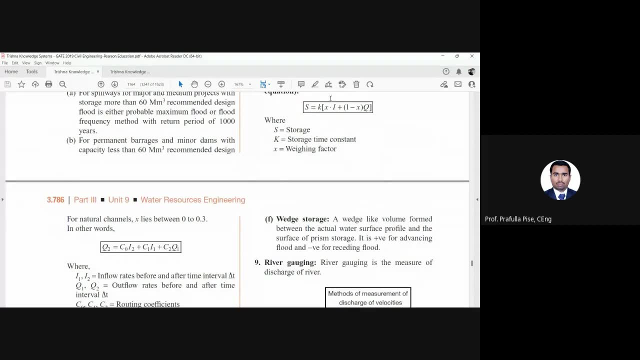 1 minus X times Q, where S is the storage, K is the storage time. constant X is weighing factor. I is inflow, okay, and T is a power factor, okay and T is a positive factor. therefore, this is Ballbeit always input goal, 24 times unto 10 a �m per second, plus 0adorat times i times q2- curioussيتcasting time. constant x is varying factor if plus one minus X times q or y, they side, if the flowllen co partnerships forces or not, sum to infel gale function of flow inogie with coverageavailability of flow. 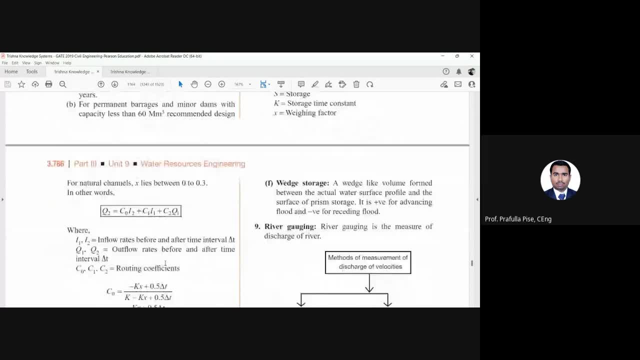 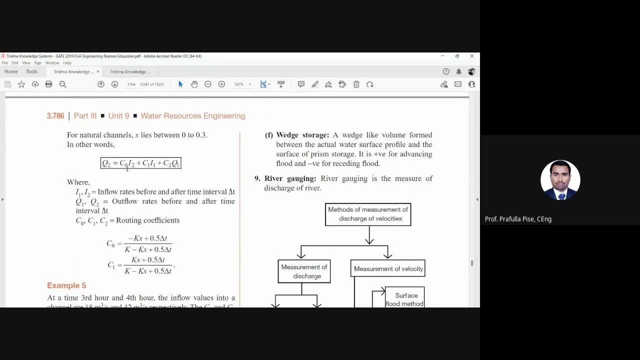 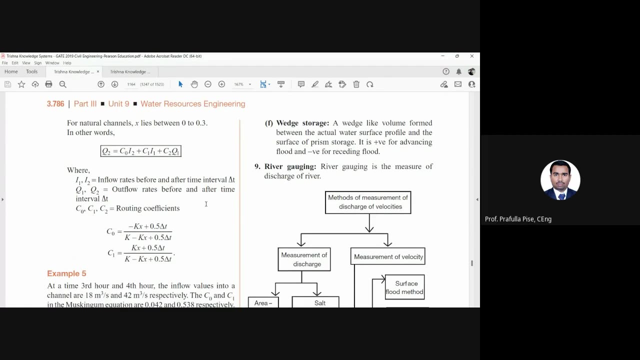 is, you know, uh, outflow for natural channels x lies between 0 to 3- 0.3. so in other words, q2 equals to c0, i2 plus c1, i1 plus c2, q1, where i1- i2 are the inflow rates between and after time interval delta. 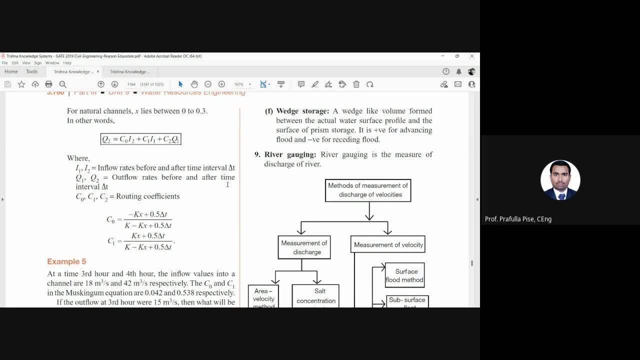 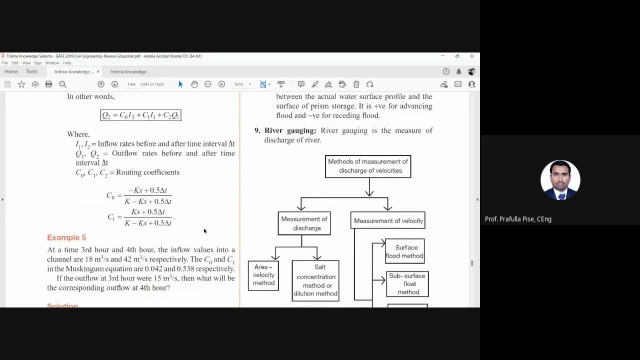 t, q1, q2 are flow rates before and after time interval. delta t, c0, c1 and c2 are routing coefficients, so c0 equals to negative kx plus 0.5 delta t. okay, why they are 0.5, so 0.. basically. 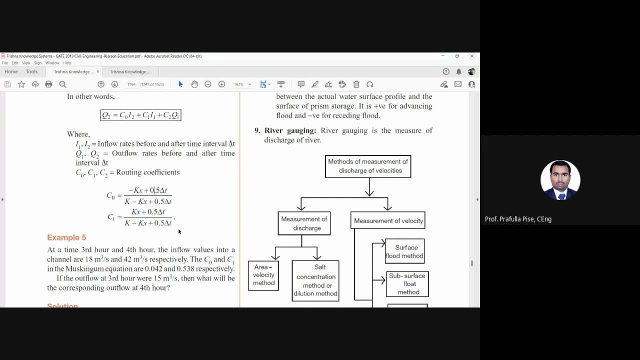 they are trying to find out the average. that's why they multiply by 0.5. okay, k minus kx plus 0.5 delta t, and c1 equals to kx plus 0.5 delta t, or k minus kx plus 0.5 delta t. 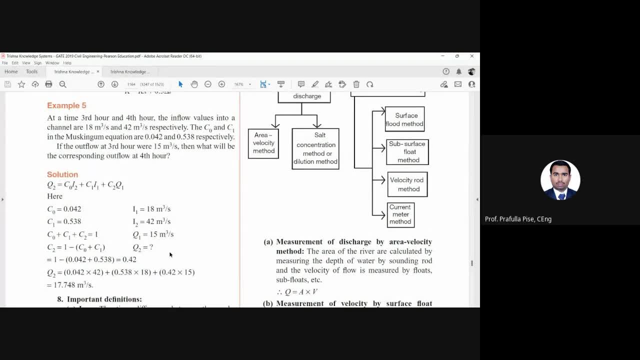 let's see an example at a time, third hour and fourth hour, the inflow values. so they said three and four, so there's basically delta t will be uh, one hour. okay, the inflow values into a channel are 18 meter cube per second and 42 meter cube per second. 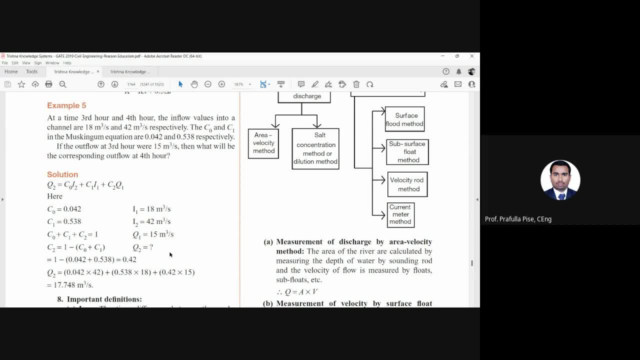 respectively, the c0 and c1 in the muskingum equation are 0.042 and 0.538 respectively. if the outflow at third hour were 15 meter to per second, then what will be the corresponding outflow at fourth hour? so if you, if you use this equation, q2 equals to c0, i2 plus c1, i1 plus c2, q1. 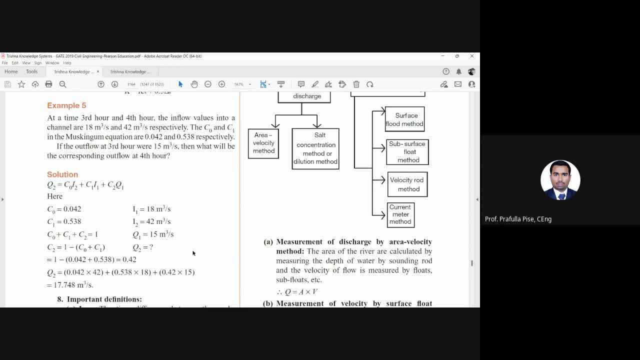 so they have given us uh c0 and c1, which is 0.042 and 0.538. they have given us i1, i2, which is 18 meter cube and 42 meter cube. they have we can uh get the value of c2, because c0 plus c1 plus c2 will. 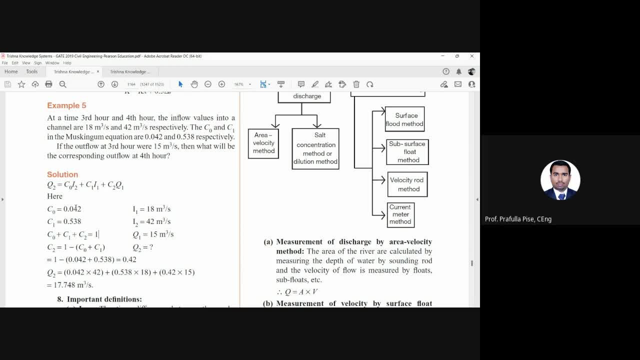 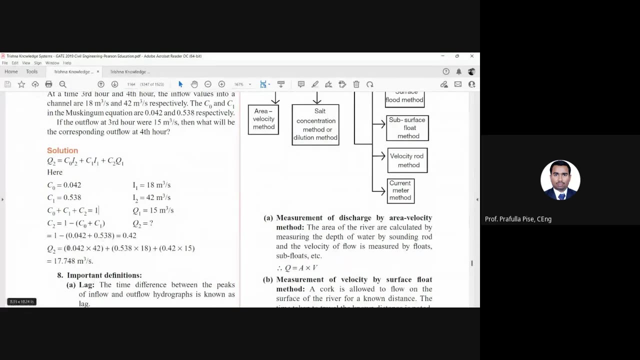 give always be one. so if you add this, two subtract one, will give us the c2, the q1, they have given us the 15 meter per second and we want to fire the q2. so now you put everything- uh, you substitute everything in the equation. you can get the q2 value. okay, that's quite easy. only the trick here: 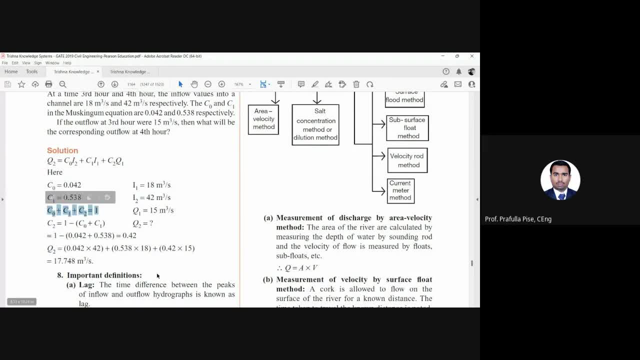 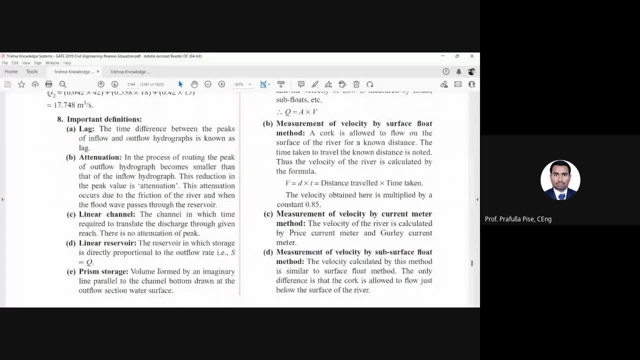 you have to understand, you have to remember: is c 0 plus c 1 plus c 2 equal to 1? okay, it is always 1.. now, what are the? these are some important definitions. lag- the time difference between the peak inflow and outflow, or hydrograph, is known as lag. 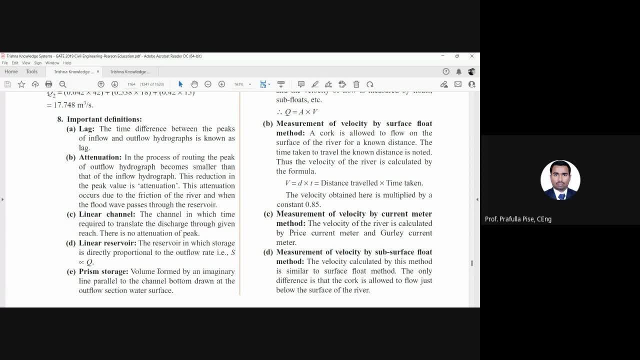 attenuation. in the process of routing, the peak of outflow hydrograph becomes smaller than that of the inflow hydrograph. this reduction in the peak value is attenuation. this attenuation occurs due to the friction of the river and when the flood wave passes through the reservoir linear channel, the channel in which time required to translate the discharge. 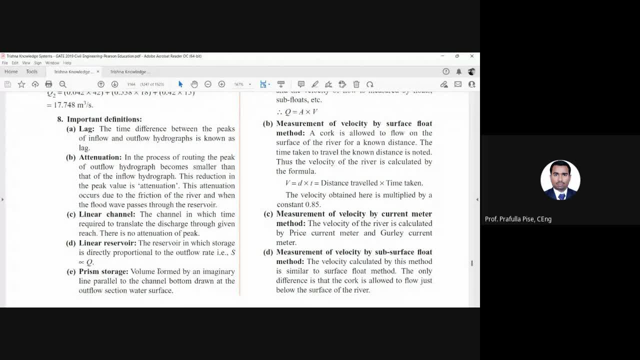 through given reach. there is no attenuation of peak linear reservoir. the reservoir in which storage is directly proportional to the outflow rate, that is, s is directly proportional to q prism storage, the volume formed by imaginary line parallel to the channel bottom down at the outflow section, water surface. 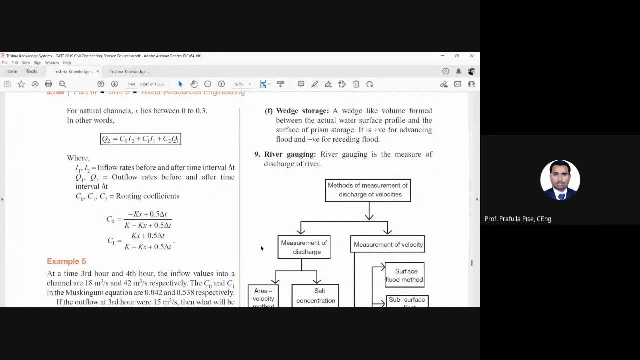 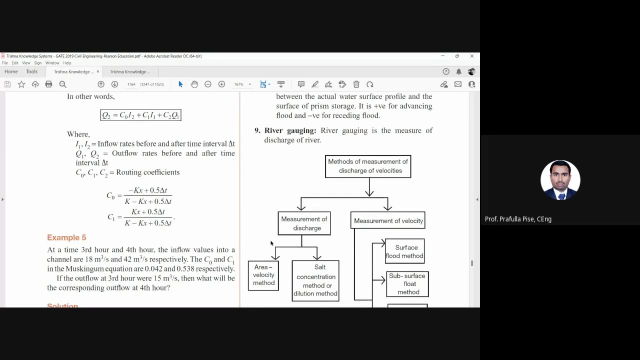 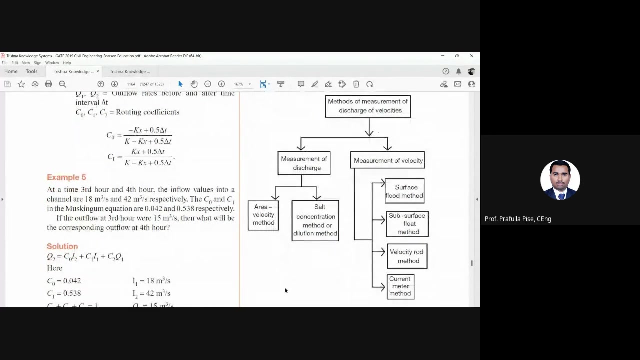 wedge storage, a wedge-like volume formed between the actual water surface profile and the surface of prism storage. it is positive for advancing flood and negative for receding flood. so that is a growth improvement and we are at this round one. the third aspect is the river gating. river gating is the measure of discharge of river. 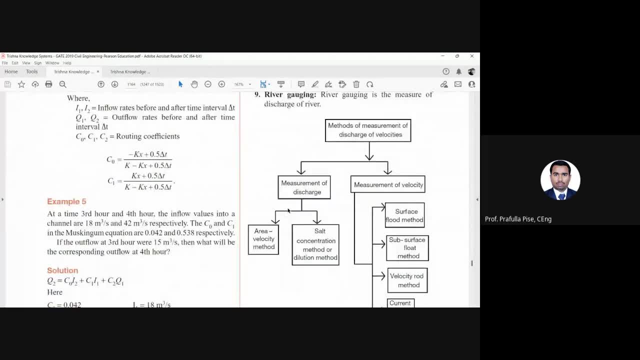 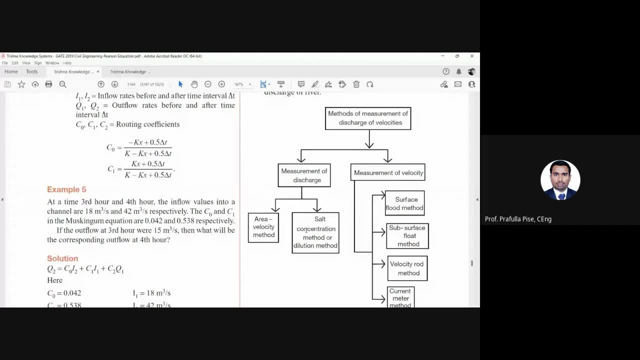 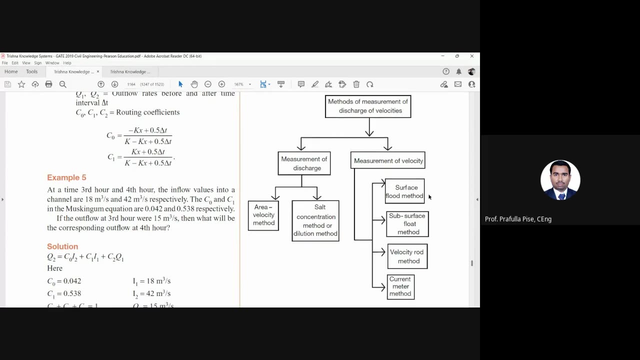 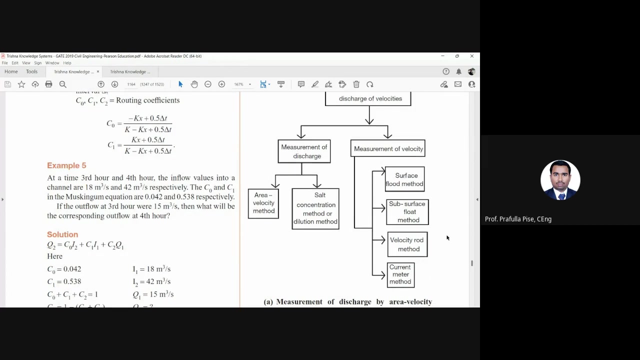 methods of measurement of discharge, of velocities. so measure of discharge and measurement of velocity. so there are two things okay, and this is salt concentration method or dilution method. this is the chemical method they use and how we can measure the velocity. so surface flood method, subsurface float method, velocity rod method and current material method. so most 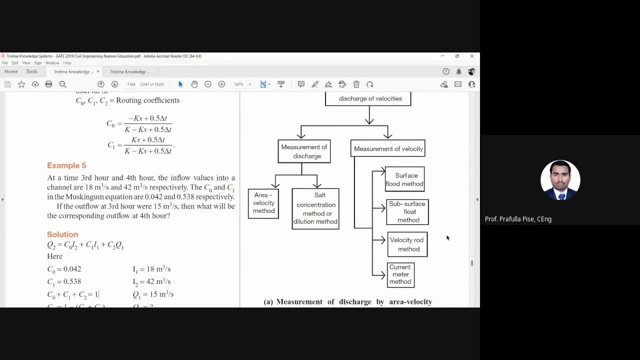 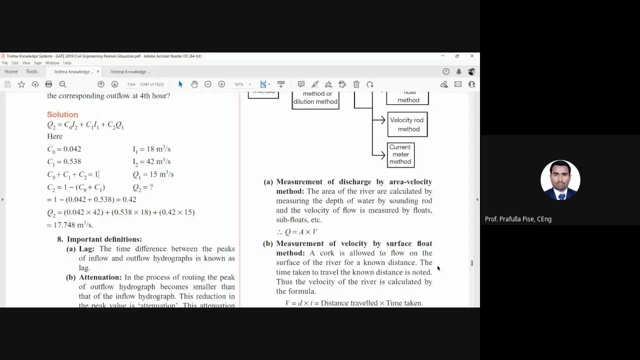 common methods used for measurement of velocity is current method method or velocity rod method. okay, measurement of discharge by area. velocity method: the area of the river is calculated by measuring a depth of water by sounding rod, and the velocity abroad is measured by floats. so a velocity flow is measured by floats. 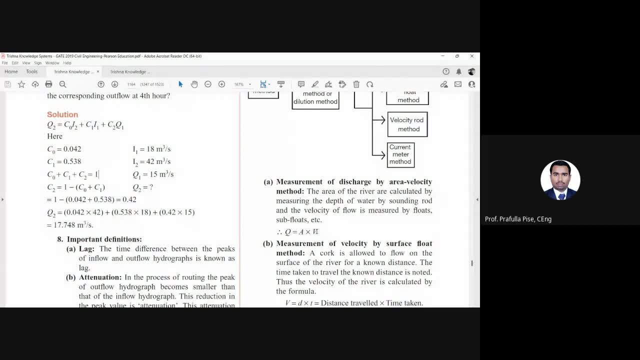 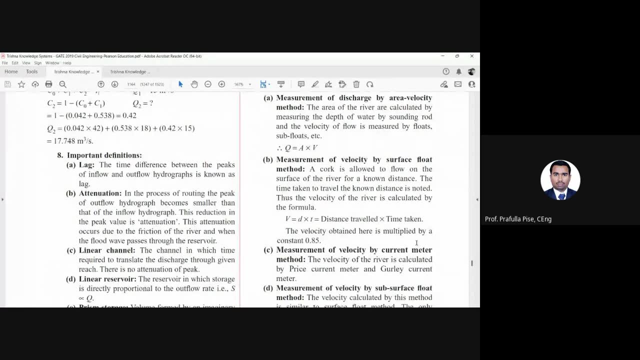 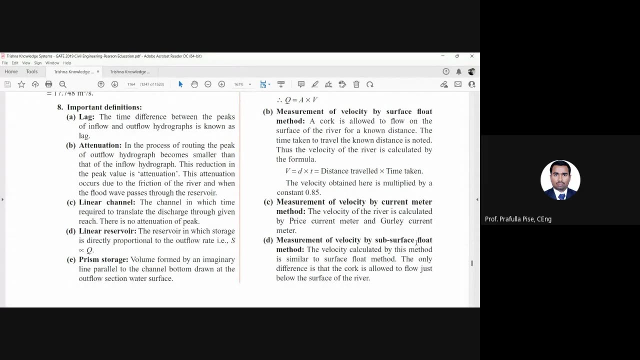 sub floats etc. so q equals to a times b, so a cross section area times. velocity- measurement of velocity by surface float method. a cork is allowed to flow on the surface of the river for a known distance. the time taken to travel, the known distance, is noted. thus the velocity of the river is calculated by the formula. 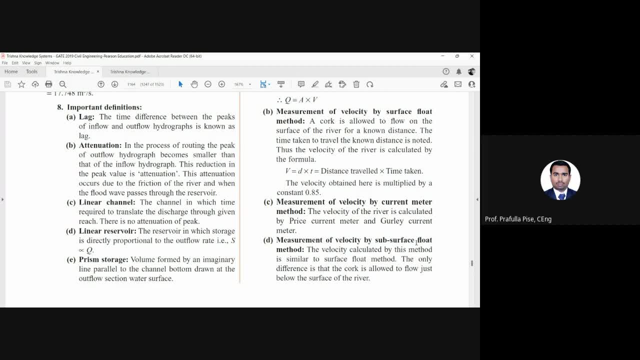 v equals to d times t. distance, travel time, time taken. the velocity obtained here is multiplied by constant 0.85. why? because you have to remember the velocity profile for a river. so surface flow, a surface value, is less than the velocity at 0.6 times height. okay, so that's why, um, they call it okay. so it's. basically, it becomes a parabola. 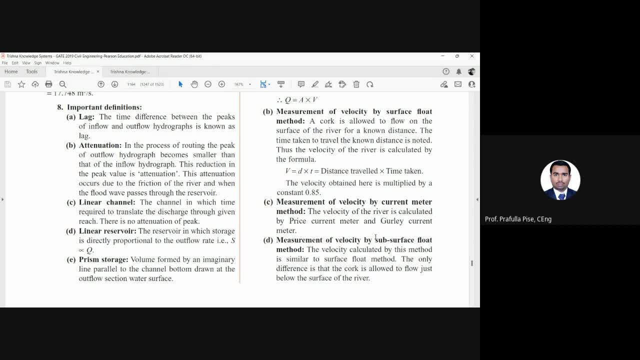 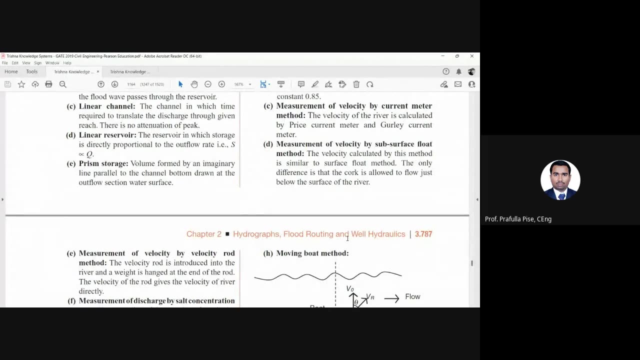 okay, and the maximum uh velocity, if we can find, is at the 0.6 times h height. okay, the measurement of velocity by current meter method. the velocity of the river is calculated by the price of the river. so, themmethrd, all five measures are shown here and you can see they arejmeter. 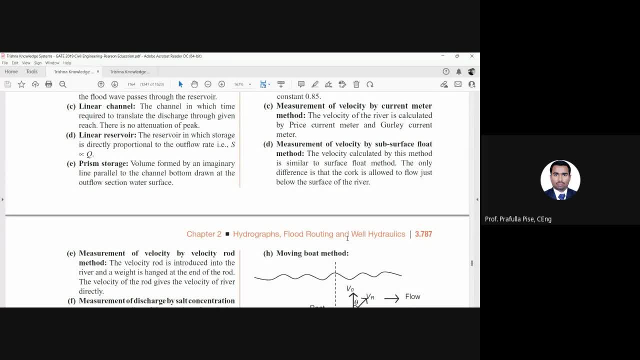 priorZ vector, price current method and Girly current meter uh in measurement of velocity by subsurface float method. the velocity calculated by this method is similar to surfaceThe velocity calculated by this method is similar to surfacebfloat method. the only difference is that the cork is allowed to flow just below the surface of river. 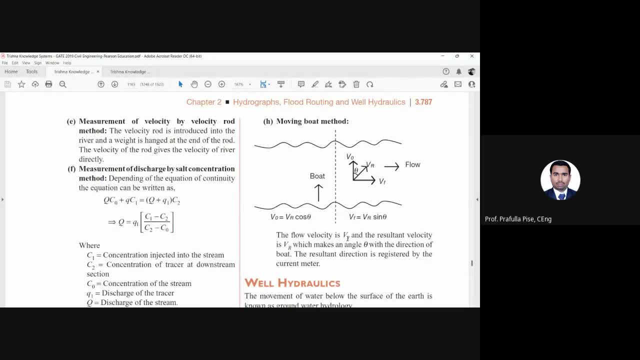 Curc is the measure of velocity byמ�. program ㅋㅋㅋ 年的 of measurement ____AJ 73 ____ about velocity Window ______. Velocity rod method. the velocity rod is introduced into the river and the weight is hanged at the end of the rod. the velocity of the rod gives the velocity of the river directly. 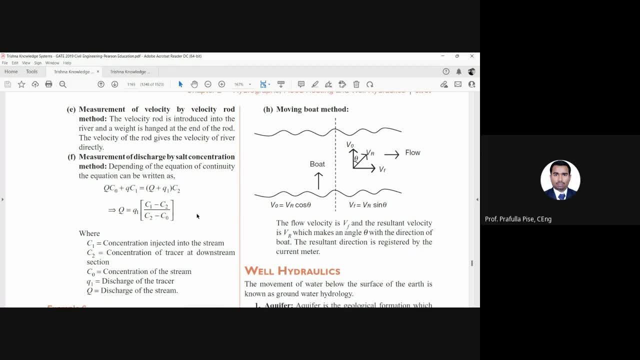 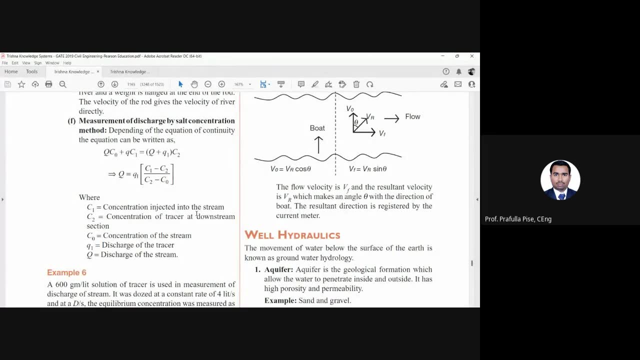 Measurement of discharge by salt concentration method, depending the equation of continuity. the equation can be written as: Q times C0 plus QC1 equals to Q plus Q1 times C2, so Q equals to Q1 times C1 minus C2 over C2 minus C0, where C1, C2, C3, C1, C2 and C0 they are. 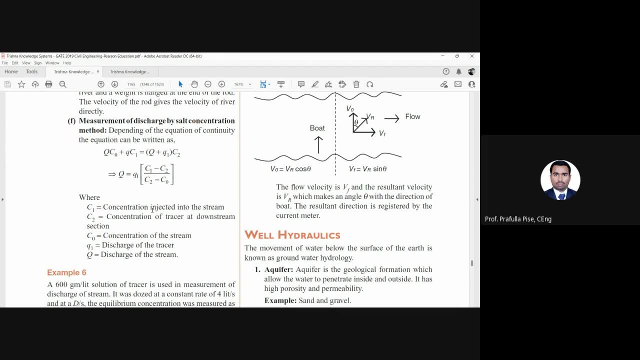 the concentration. so C1 is constantly injected in the stream. C2 is the concentration of trace, So C1 is constantly injected in the stream. C2 is the concentration of trace. So C1 is the concentration of trace at downstream section and C0 is the concentration. 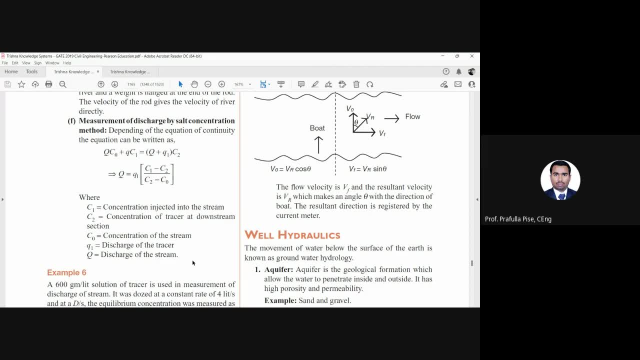 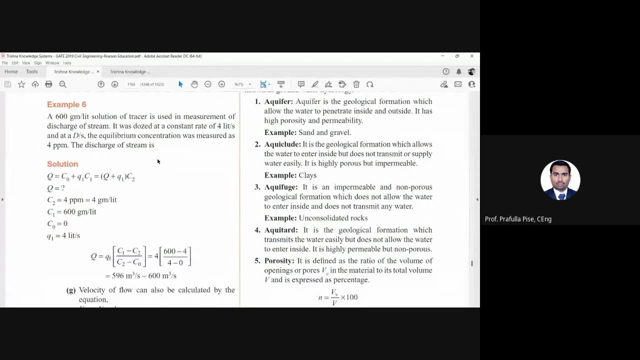 of stream. Q1 is the discharge of tracer and Q is the discharge of stream. that is something you have learned in your applied chemistry or engineering chemistry in first year. okay, concentration method. Now let's see an example. a 600 gram per liter. 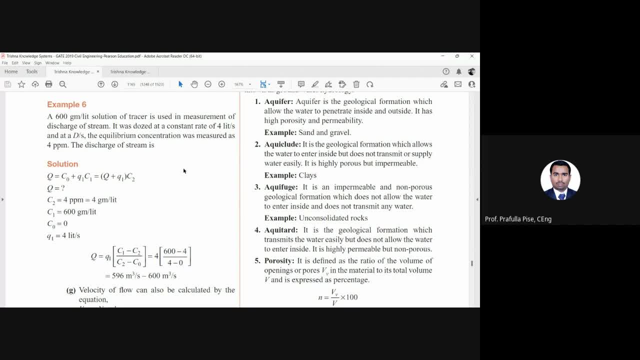 solution of tracer is used in measurement of discharge of stream. it was dosed at a deconcentrate of 4 liter per second and at a downstream. okay, here they say yes. the equilibrium concentration was measured as 4 ppm, 4 parts per million the discharge. 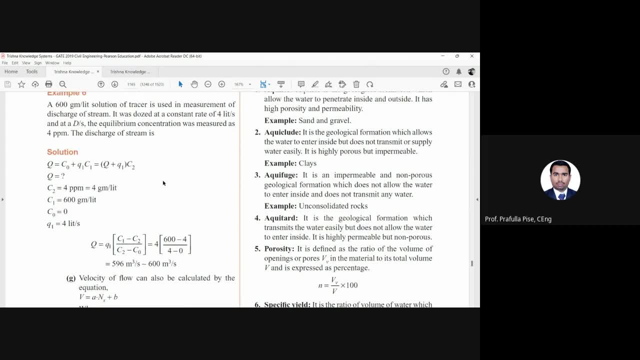 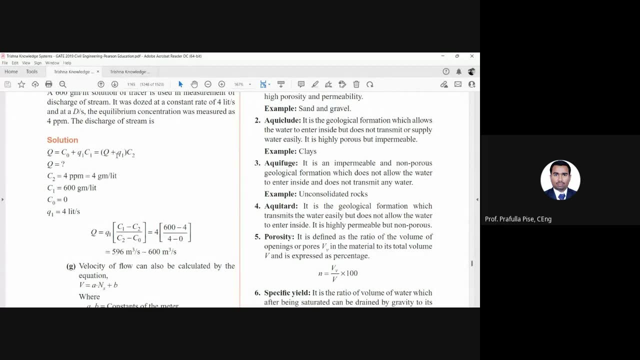 of stream is so that we are trying to say 4 ppm, We are trying to find out the discharge, so Q equals to C0 plus Q1, C1 equals to Q plus Q1 over C2, we are trying to find out the Q, so C2, they have given us 4 ppm, okay, so 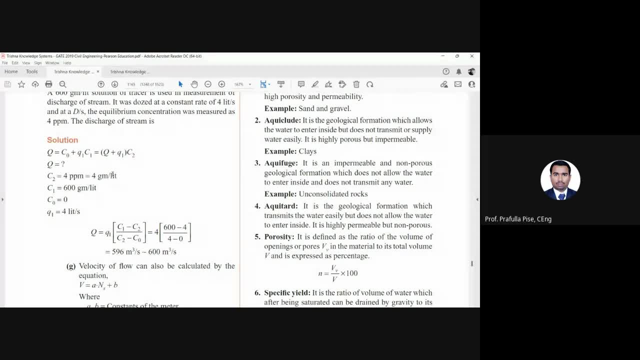 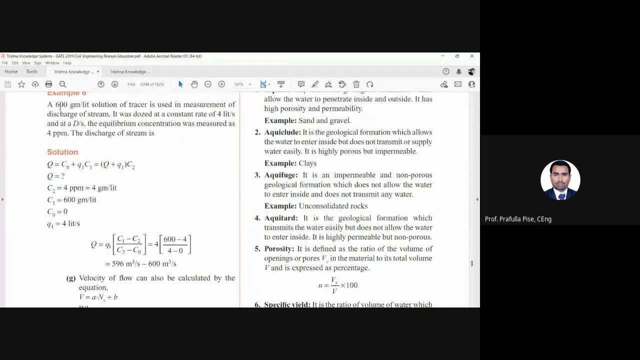 4 parts per million, so basically 4 grams per liter. C1 equals to. they have given us 600 grams per liter. See what they did. they gave one in ppm and they gave one in gram per liter. so we have. 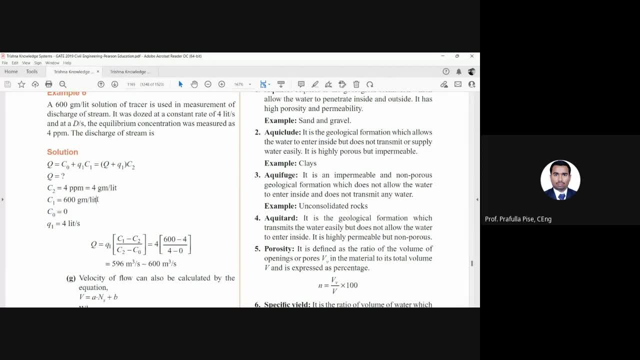 to either make both them in grams per liter or make both them in ppm, okay. so, since we are working hydrology, not in chemistry, so we are going to make them in gram per liter, not in ppm, okay, In chemistry, whenever we work, we work only in ppm, so we have to make them in grams per 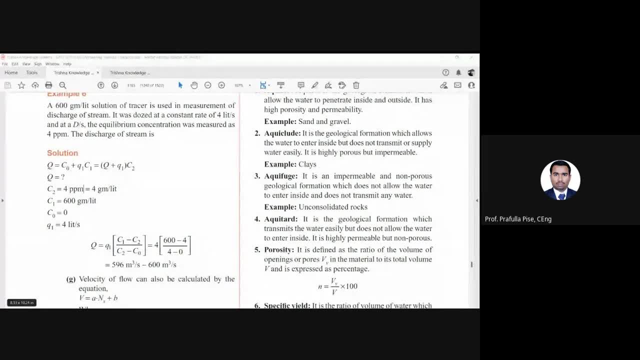 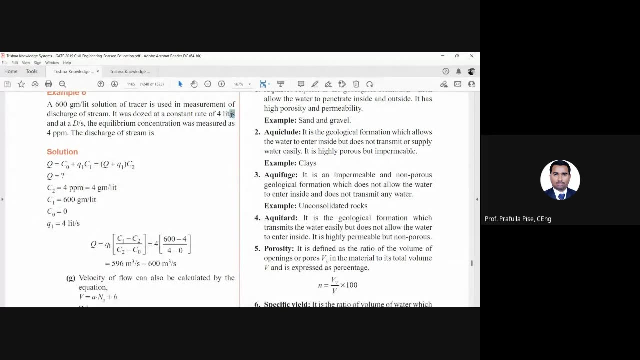 liter. But in hydrology, civil engineering, we don't work in ppm, we work in gram per liter. So it will be easy for us to, you know, convert into meter or second. okay, in SI system- Now Q1,, they have given us in liter per second. okay, 4 liter per second. C0 is zero, C0 is: 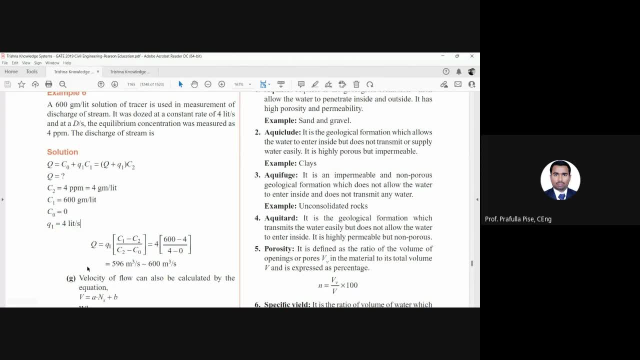 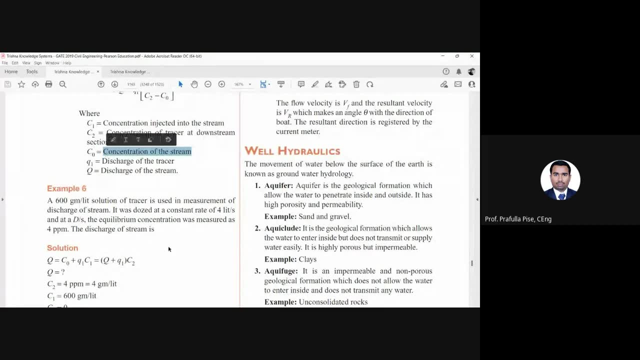 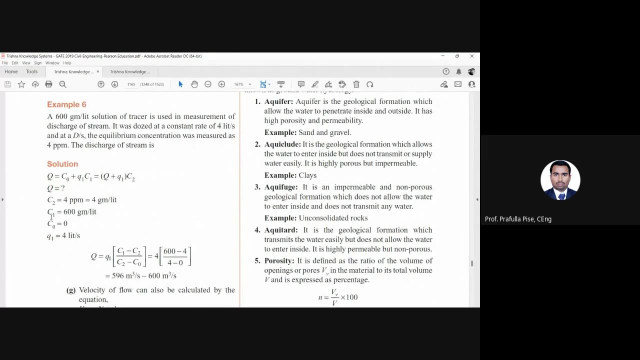 nothing but 0,. okay, so C0 is nothing but 0.. Okay, Okay, Okay. So C0 is nothing but the concentration of stream, so there is nothing in the stream, so it is a clean stream. that's why C0 is equal to 0. 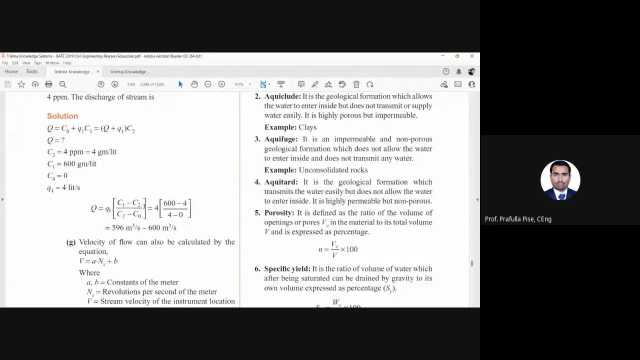 So if we use the equation, Q equals to small q1, C2 minus C1, C1 minus C2, whole C2 minus C0, you get your answer, which is 596 meter cube per second. nearly 600 meter cube per second. 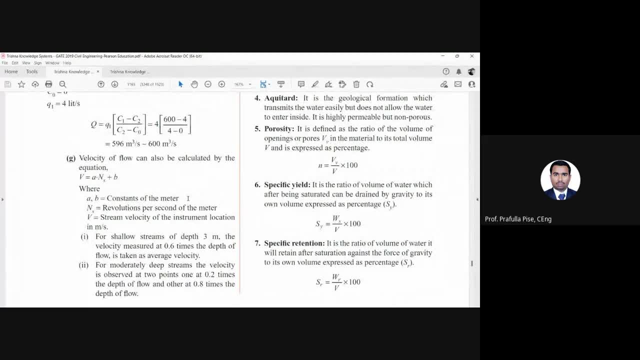 Now the next velocity flow can also be calculated by equation Q1.. Okay, by equation, b equals to a times ns plus b, where a and b are constant of meter. ns is the revolution per second for the meter and b is the stream velocity of the instrument. instrument location: 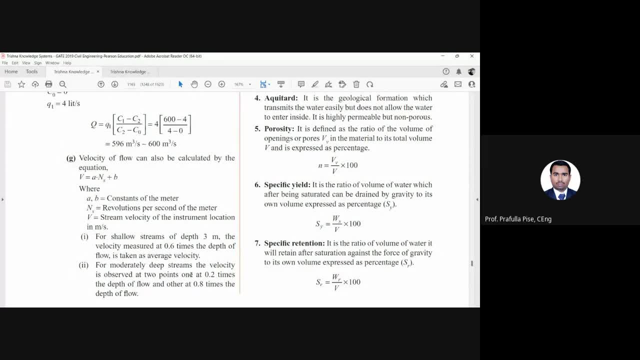 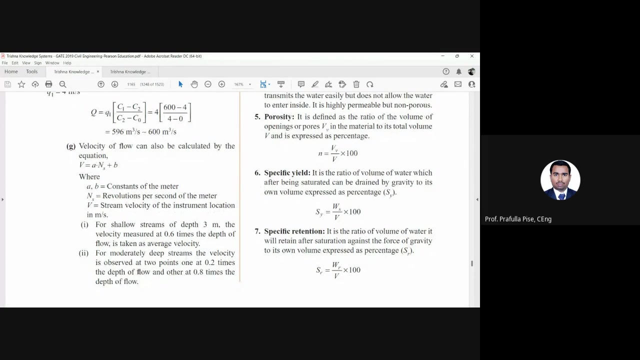 in meter per second. the shallow strips of depth: three meter. the velocity measure at six, 0.6 times the depth of flow. why, remember, i told you, because at 0.6 times of depth, that's where we have the maximum velocity, okay, for moderately steep streams. the velocity observed at two points, which is at 0.2 times and 0.8 times. 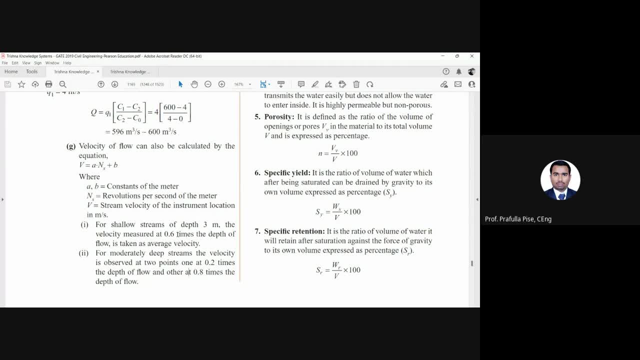 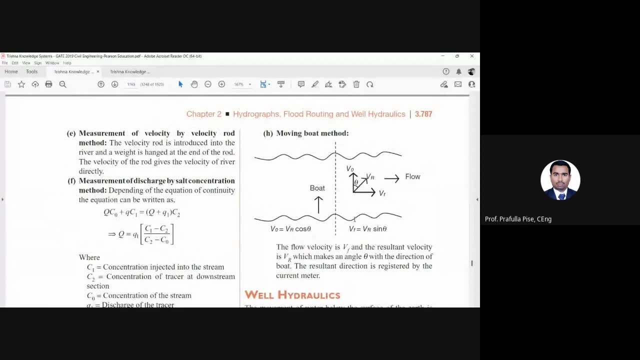 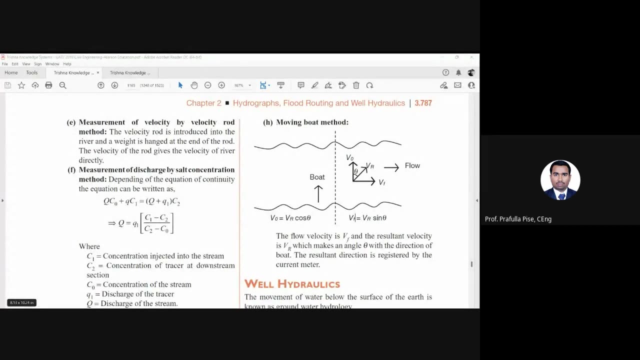 okay, basically, if you take the average, it is going to get up to 0.6. okay, so 0.2 and 0.8. okay, now moving boat method. so this is something you have to remember. we did, or we solve similar kind of problems, uh, in the engineering mechanics. okay, remember. 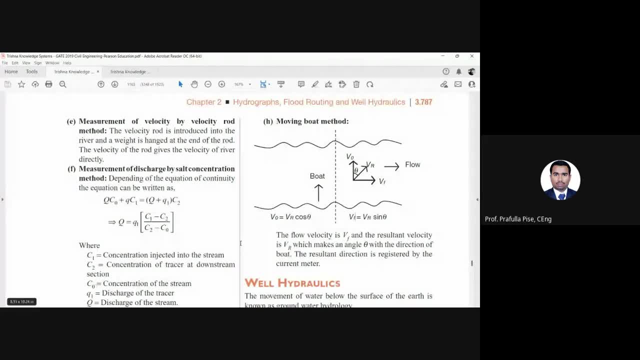 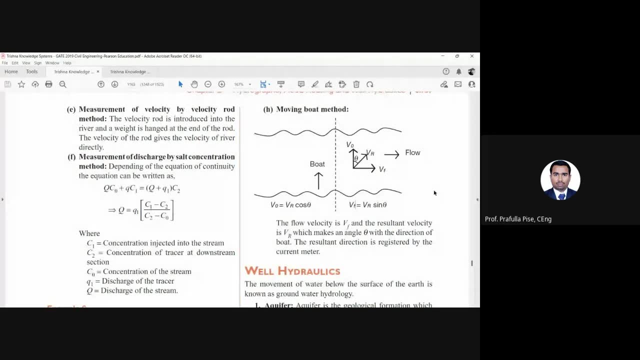 engineering mechanics, we have solved this kind of problems. the moving boat: okay, so the flow velocity, vf, and the result velocity is vr, which makes an angle, uh, theta, with the direction of both. okay, so, vf and vr, the resultant direction is registered by the current meter. okay, so we have both traveling. 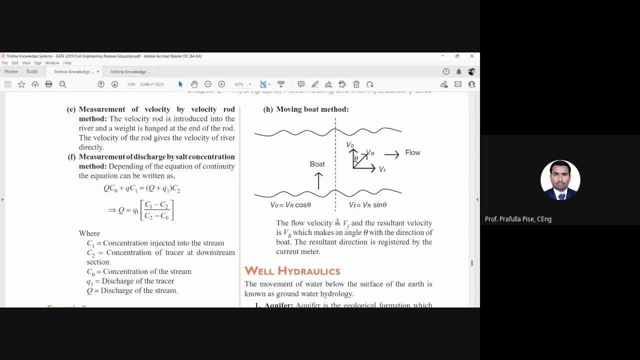 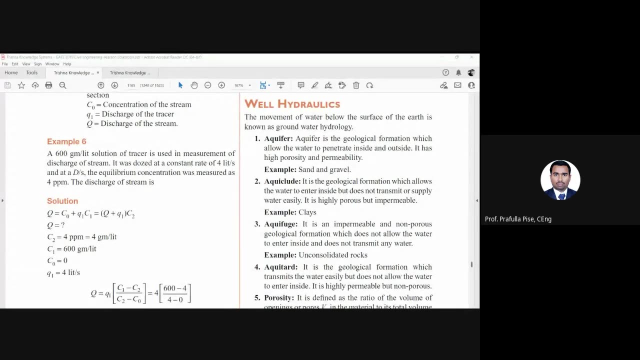 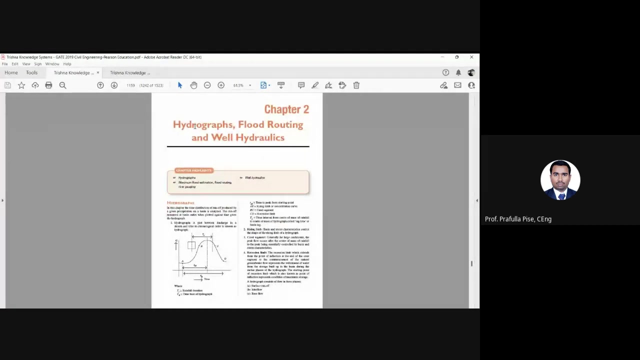 from here to there, okay. so usually it doesn't go straight away, it goes something along the edge. okay, now that's done with the hydrology, okay. so, if you remember, we started with hydrographs and then we done hydrographs and flow routing. now the last topic is, well, hydraulics. 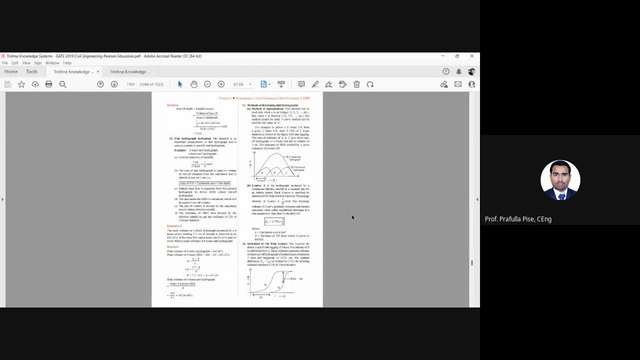 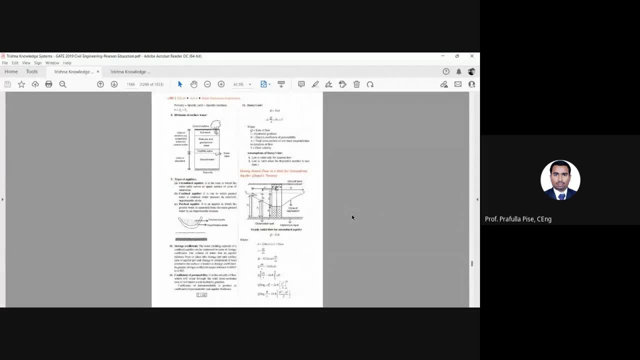 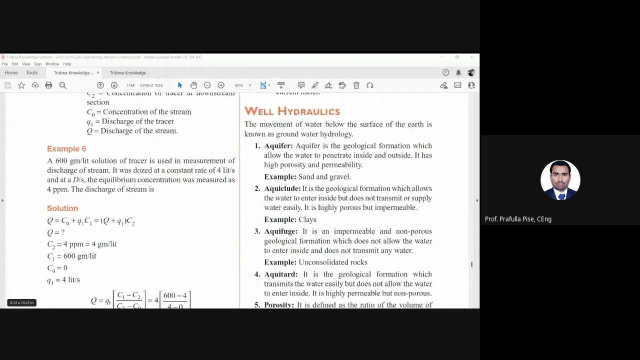 so after the well hydrates, we are going to finished with the um hydrology. okay, after that there is nothing about the hydrology. so do you want to take a break or do you want to continue and finish the well hydrology? mayuri harsha varadhan. 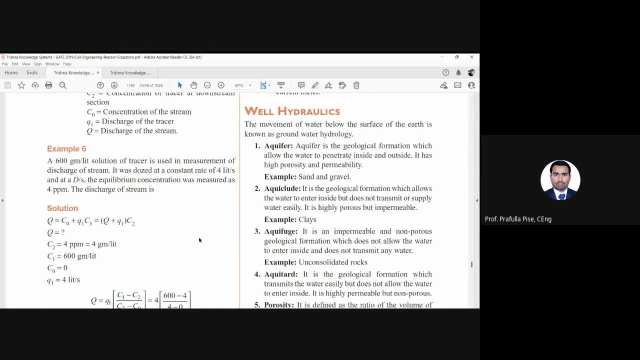 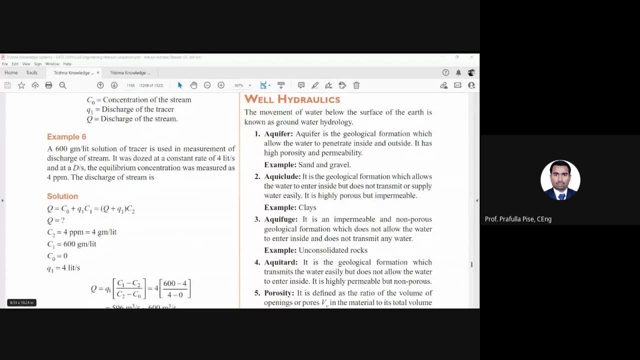 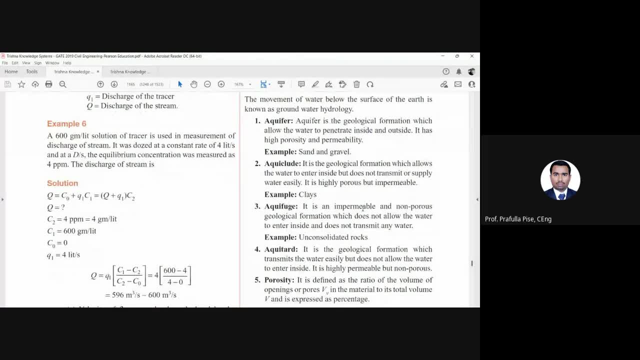 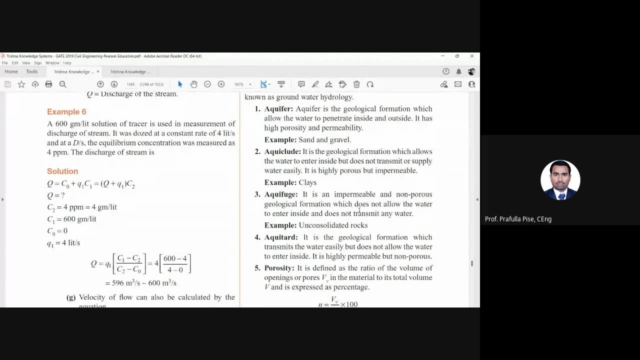 groundwater hydrology. it's obviously we know that aquifer, aquifer fur, is a geological formation which allow the water to penetrate inside and outside. it has high porosity and permutation and permeability, For example, sand and gravel Aquaclude. it is a geological formation which 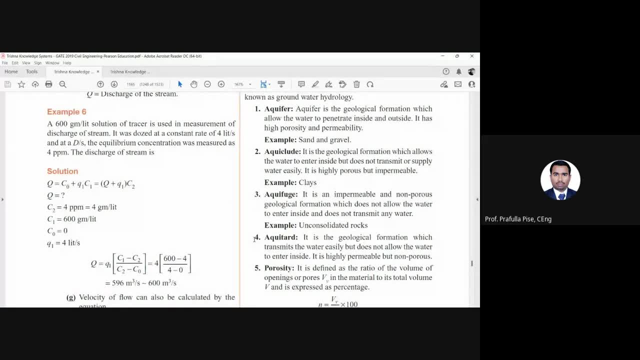 allows the water to enter inside, but does not transmit or supply water easily. It is highly porous but impermeable. So that is clay: High porosity, permeability, Highly porous but impermeable. Sand clay. That's how you remember things: Aquiferge it is. 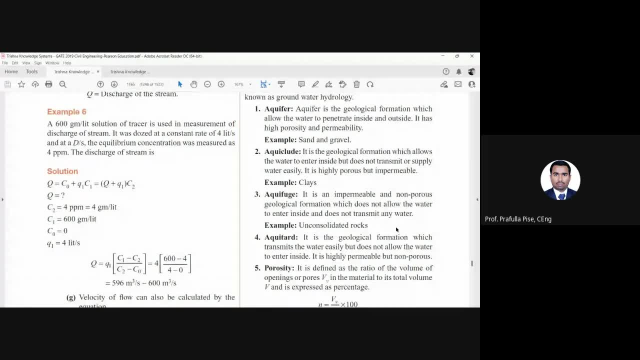 an impermeable and non-porous geological formation which does not allow the water to enter inside and does not transmit any water. So that is called unsolicited rocks. So sand, clay, Clay and rock Aquiferge, aquaclude, aquiferge, Now aquitard. it is the geological formation. 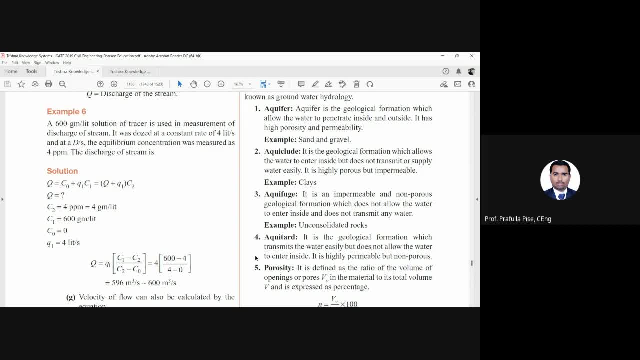 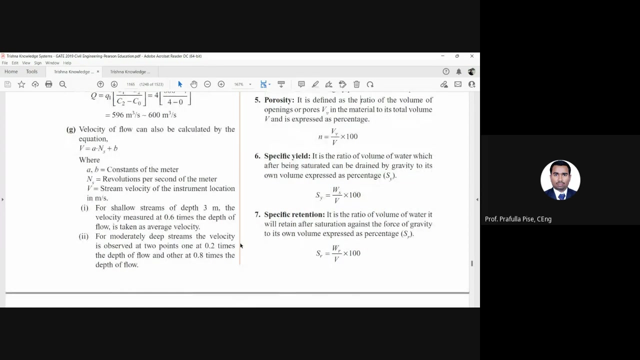 which transmits the water easily but does not allow the water to enter inside. It is highly permeable but non-porous. Here it was porous but impermeable. Here it was non-permeable, Non-porous and highly permeable Now. porosity: it is defined as the ratio of volume of openings. 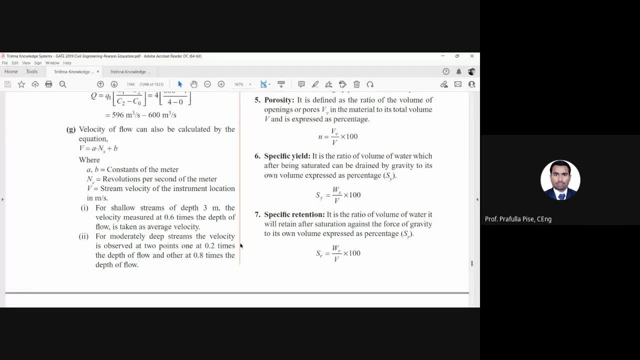 or pores in the material to its total volume, And it is expressed as percentage. So N equals to VV, volume of voids over V times 100.. You have to remember, you have to remember this formula from soil mechanics or geotechnical engineering: Porosity. 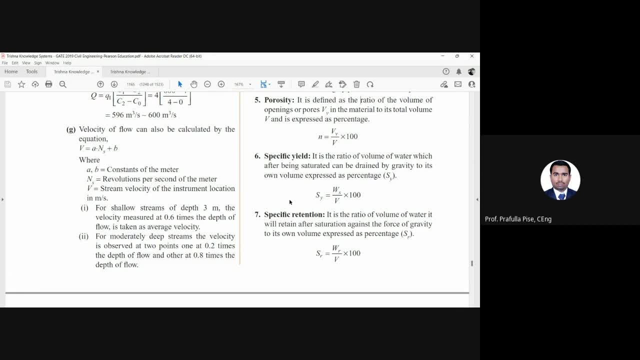 The specific yield. it is the ratio of volume of water which, after being saturated, can be drained by gravity to its own volume, expressed as percentage. Okay, So SY equals to WS, so weight of solids over volume times 100.. Okay, You have to remember. 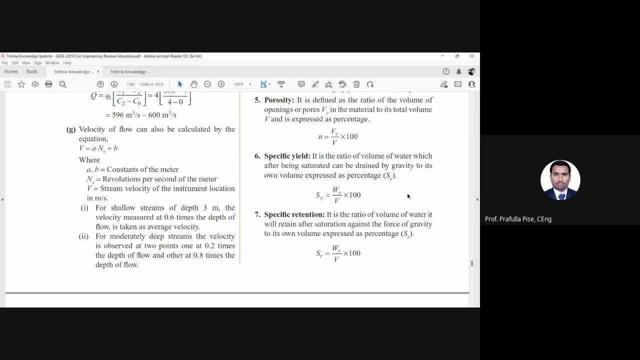 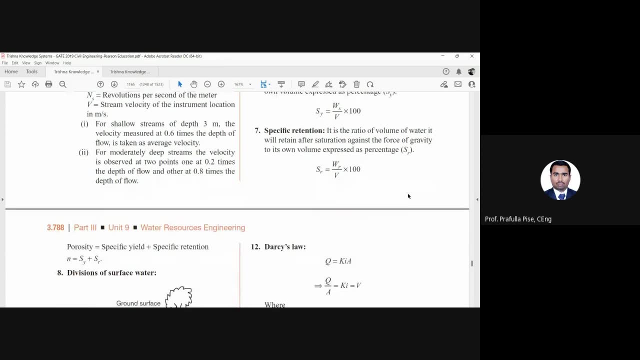 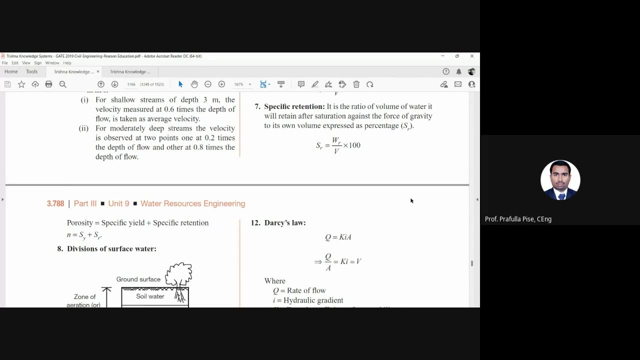 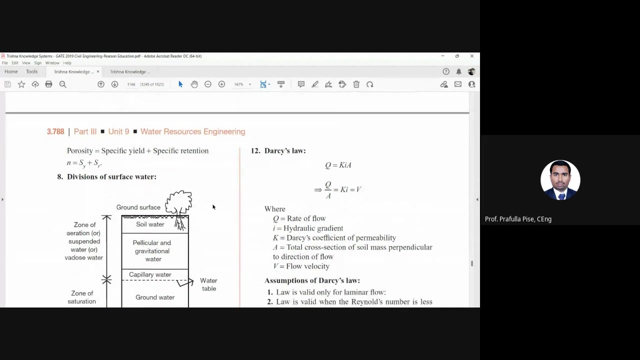 Okay, uh it from your uh soil mechanics or geological engineering, specific retention, that the ratio of volume of water it will retain after saturation against the force of gravity. so its own volume expert uh expressed as percentage. so sr equals to wr over v times 100, so positive equal to specific yield plus specific retention, so n equal to sy plus sr. 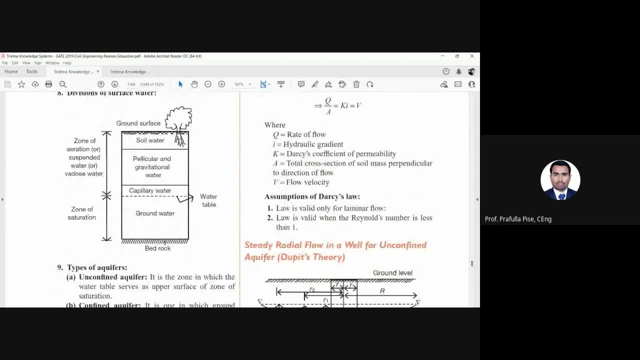 now division of surface water. so we have the bedrock, then we have ground water and the top of the groundwater is what requires a ground groundwater table or water table. then we have capillary water. okay, so below the groundwater table, that's what requires zone of saturation. 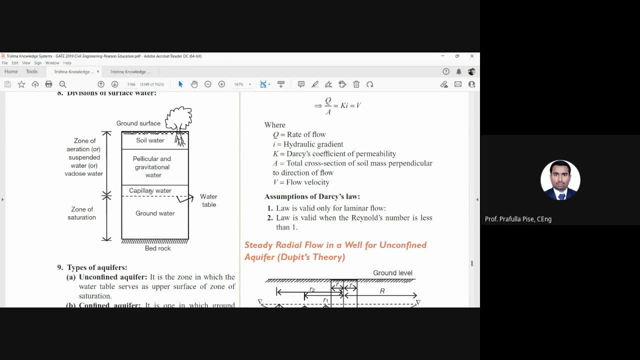 or saturation zone and about that. above the groundwater table, what we have that is the zone of aeration, or suspended water or waters water. okay, so we have capillary water, then we have pellicular and gravitational water and then we have soil water. above that, obviously, surface water. 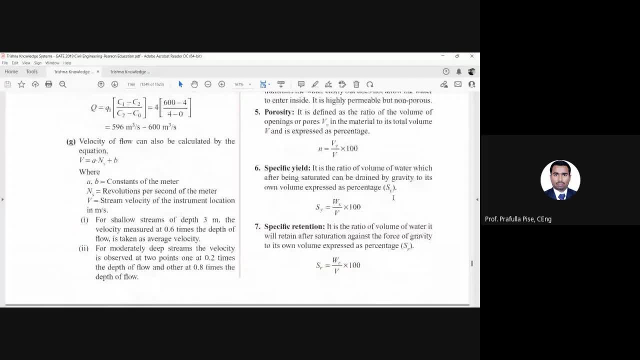 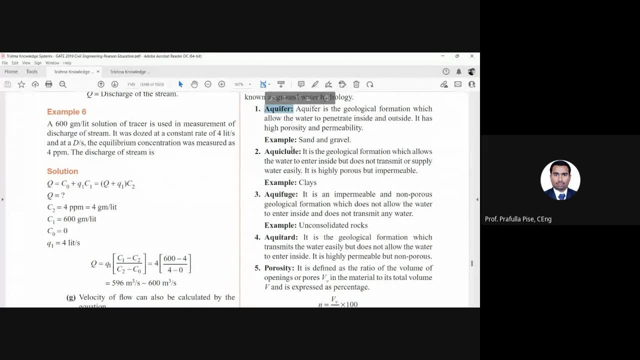 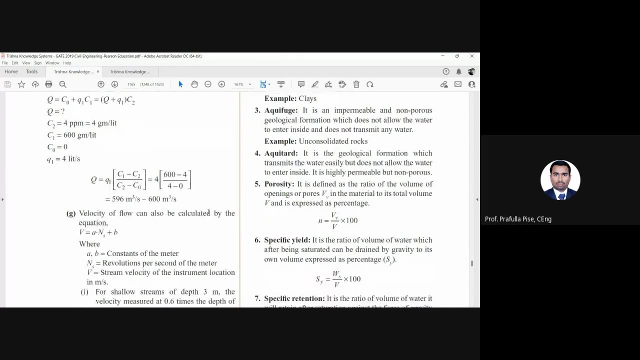 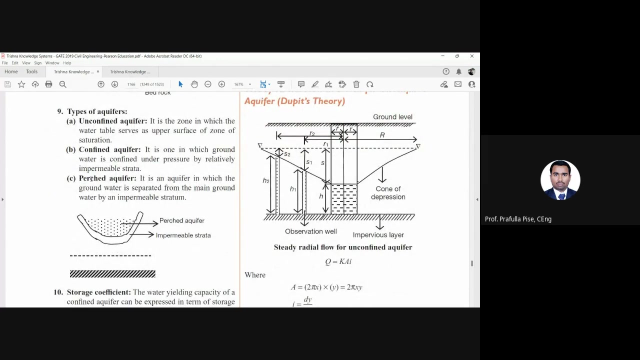 now we are most important, uh, most uh interested in aquifer, okay, rather than the active aquifers or aquitard, okay. so we are always concerned or interested in aquifer. there are different types of aquifer: unconfined aquifer, confined aquifer and purged aquifer. 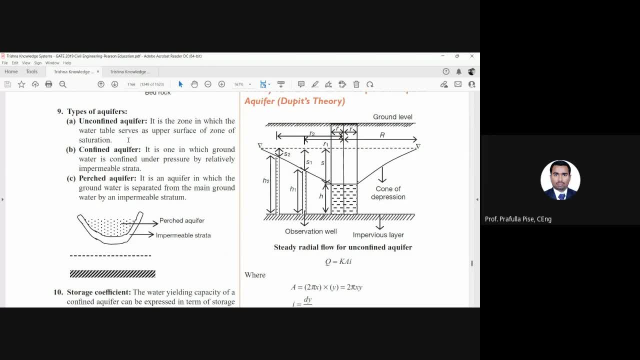 so what is this? unconfined? so it is the zone in which the water table serve as upper surface zone of saturation. confined, it is the one in which ground water is confined under pressure by relatively impermeable strata. now, first aquifer, it is an aquifer in which the groundwater is separated. 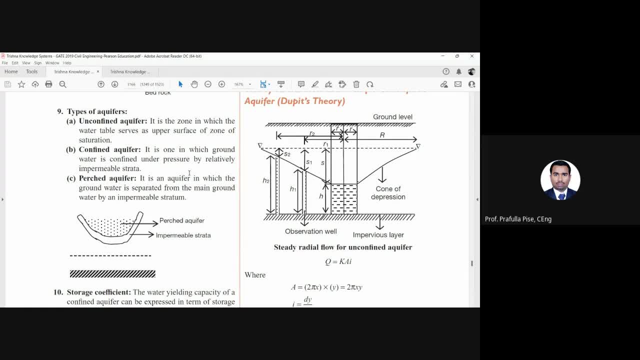 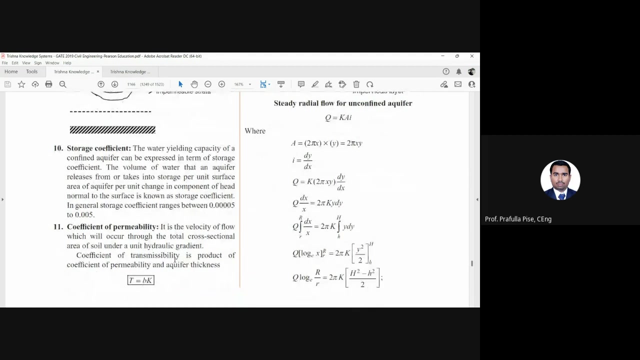 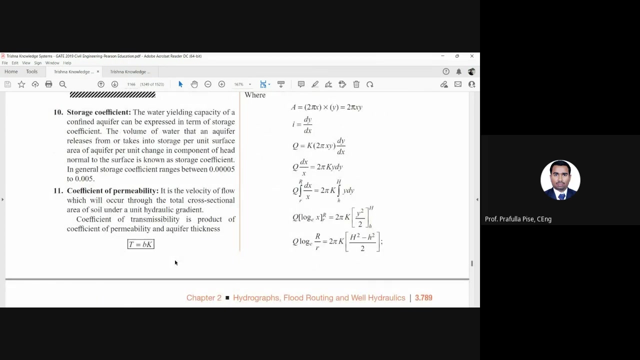 from the main ground water by impermeable strata. okay, so impermeable strata first aquifer, okay, so it usually makes, like you know, a lake. okay, first aquifer, now storage coefficient: the water yielding capacity of a confined aquifer can be expressed in terms of 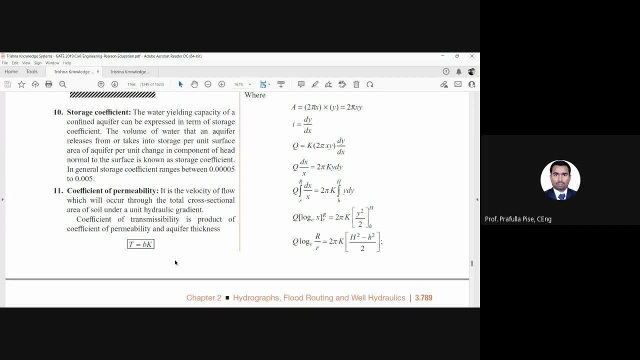 storage coefficient: the volume of water that an aquifer releases from or takes into storage per unit. surface area of aquifer per unit. change in component of head, normal to the surface, is known as storage coefficient. in general, storage coefficient ranges between 0.0005 to 0.005. okay, so in this kind of problem, for this kind of 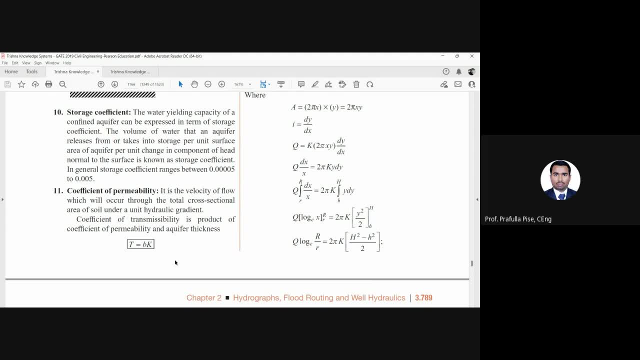 question. you just have to remember or you have to understand the range of storage. coefficient- okay, the rest of the things not much okay. coefficient of permeability: it is the waste of flow which will occur through the total cross-sectional area of soil under a unit hydraulic gradient. coefficient of transportation, coefficient across the area. a particular one is a return coefficient of flow. The deflection coefficient is t and t verdad. cold flow flow means the지만 of pre- fades per unit area under period. Grassland: The base size is 0.6. powertrain level of soil: the: 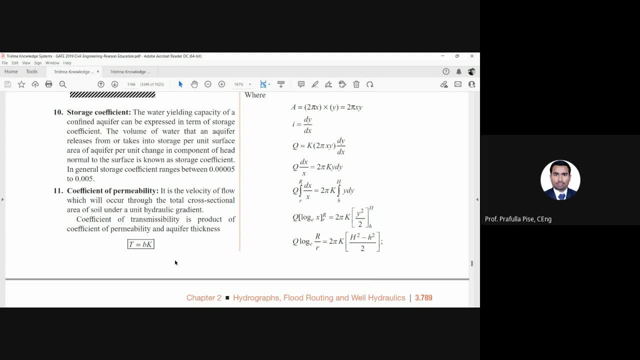 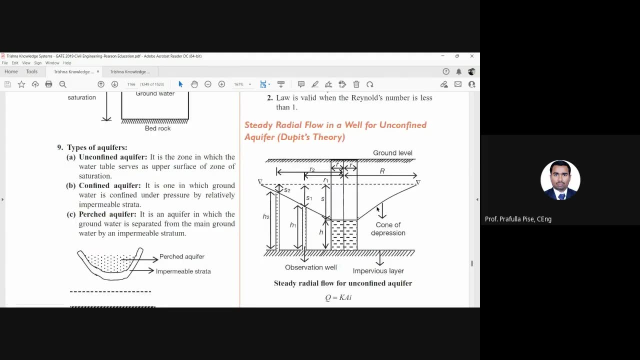 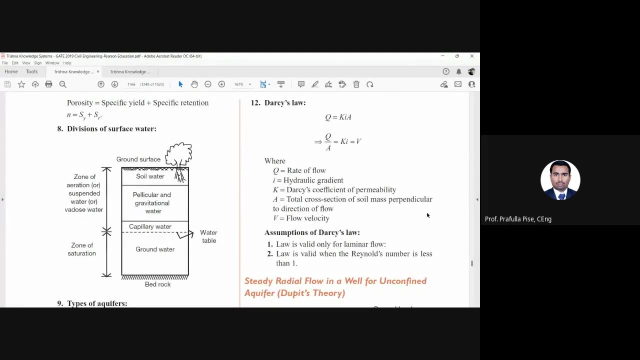 of transmissibility is product of coefficient of permeability and aquifer thickness. so t equal to b times k. okay, and the most important, most popular formula which we are going to use in groundwater hydrology, or well, hydraulics, is darcy's law: q equal to k, i a, where q is the rate of flow, i is the hydraulic. 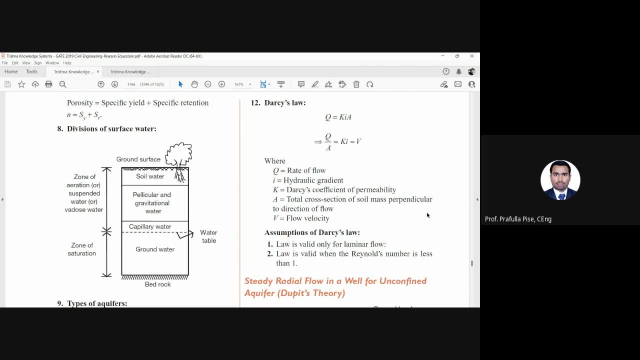 gradient. k is the darcy's coefficient of permeability, a is the area, uh, total cross section area. okay, it's cross section area of soil mass perpendicular to direct shown of flow and we can say the flow velocity, the assumptions of darcy's law, again, very 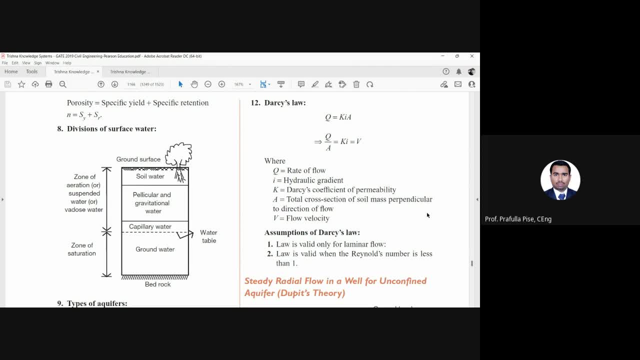 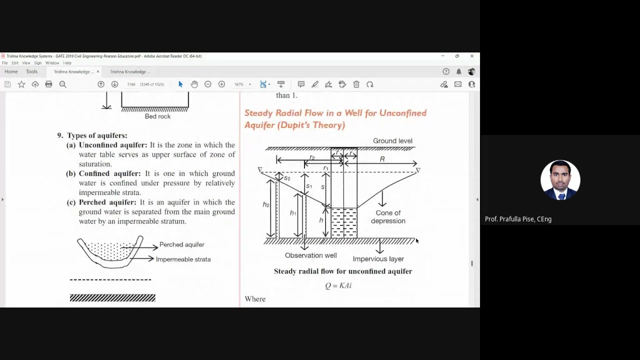 important law is valid only for laminar flow. if the flow is turbulent, we cannot use darcy's law. and law is valid when reynolds number is less than one. when reynolds number is more than one, we cannot use darcy's law. that's very important thing, because those are again can be asked in the exam. 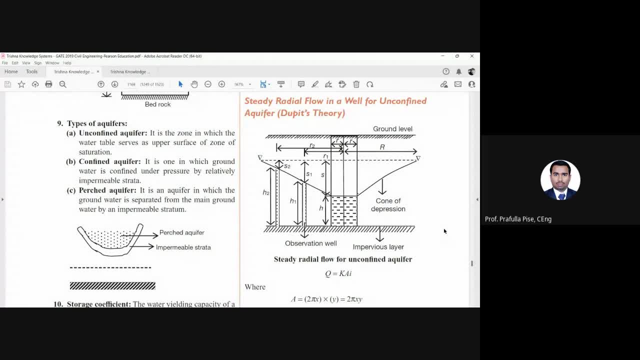 a steady radial flow, in a way for unconfined aquifer. so we are going to use dupitz theory. okay, now, any one of you remember this kind of diagram? if not, and i will tell you. okay, so this is what we have. well, okay, and this is the dotted line is the ground water table. okay, so water flows, okay. 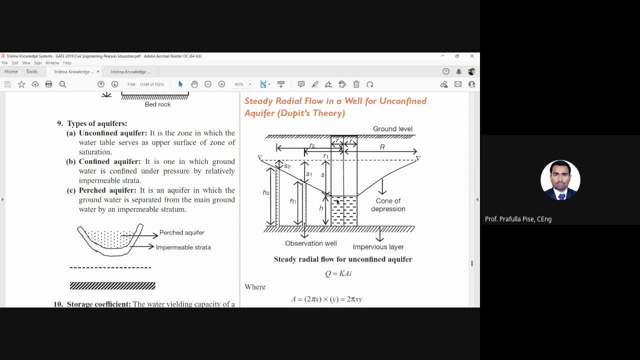 in between this, that's what quasi cone of depression, and this is what we have: water inside the well, so that's well okay. so if you find out the center of that, well okay. so r this side, r this side so, radius of the well, okay. total d diameter of well from the center: this r capital r okay. and then we have 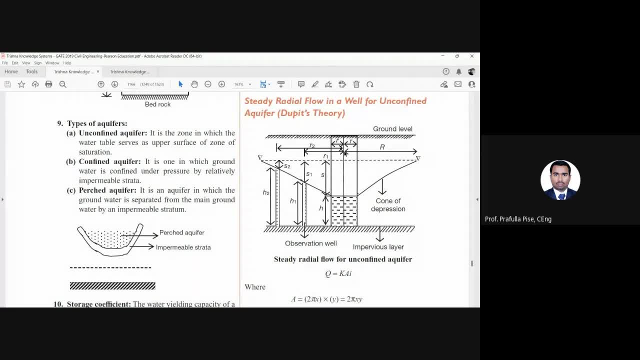 this also capital r. okay, up to this point. so, small r and capital r, these are the two r's you have to remember, okay? and then h is the height of water, okay, from the impervious layer, and this is the s is the height or depth of water from the groundwater table. 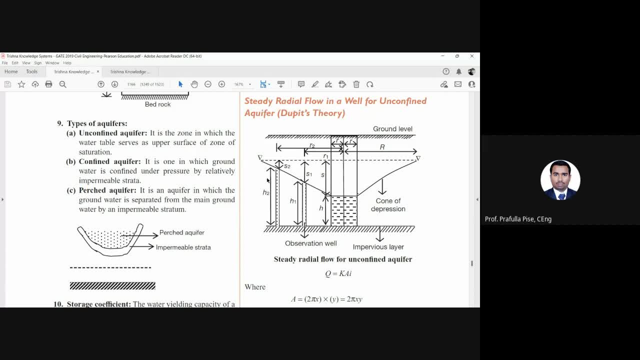 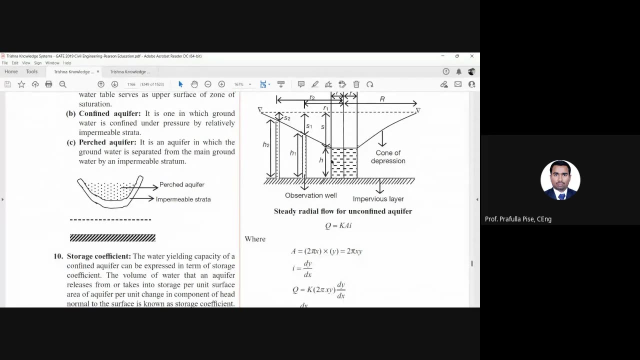 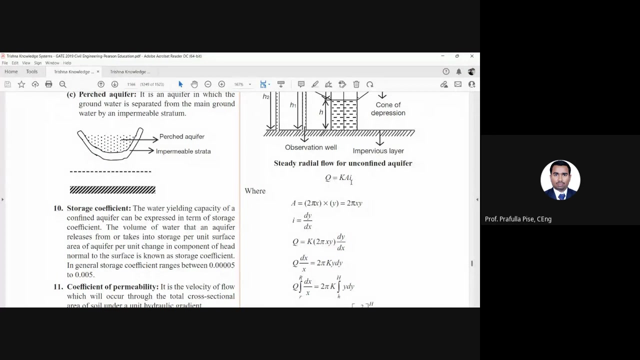 same thing. we have s1 and s2 and h1 and h2, because we are going to use a lot of trigonometry, okay here. okay, so these are the observation, well one, observation well two, and this is the actual, well steady, uh, radial flow for unconfirmed aquifer. again, q equals to k, i, a, a is the 2, pi, x, so area. 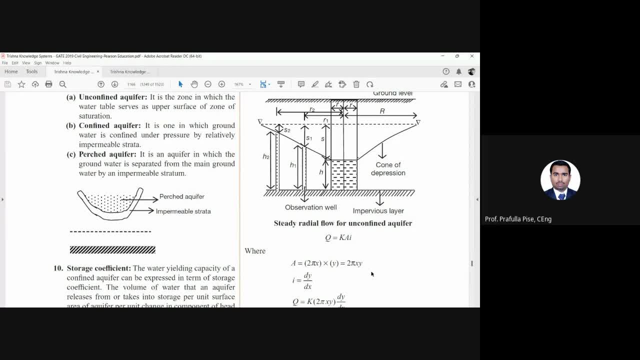 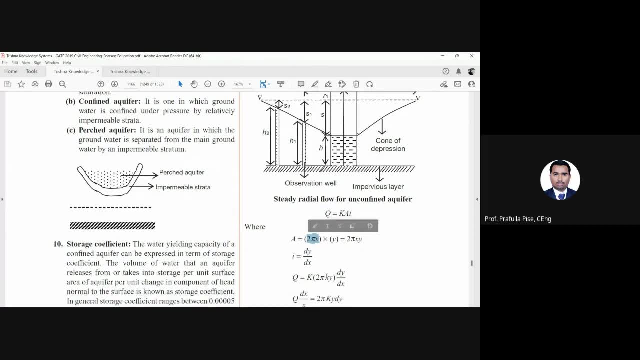 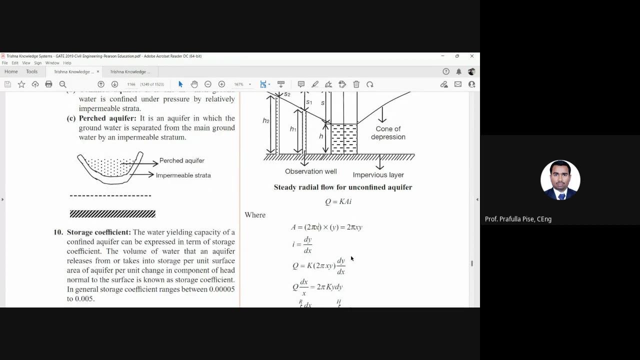 2 pi x times y, so equals to 2 pi x- y. okay, 2 pi x means, if you remember from your geometry, 2 pi r is the perimeter. it is the perimeter of your circle, okay, so that's why we have 2 pi x and y is a small depth, so that will give us the. 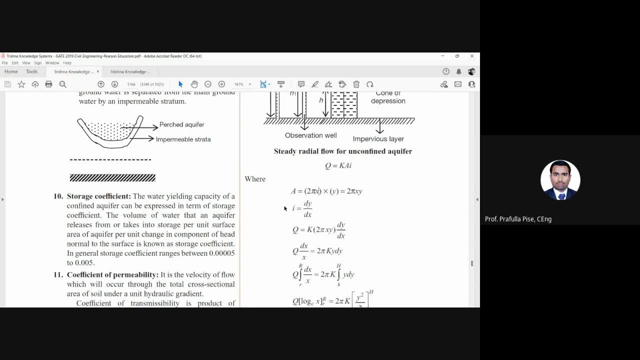 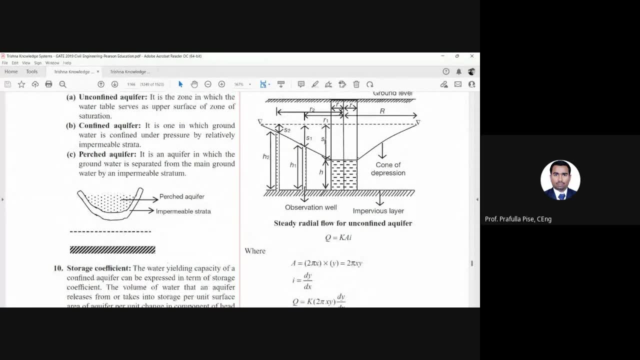 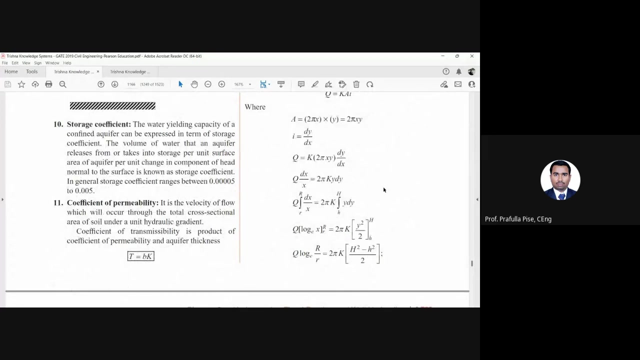 total area, total area, so i is nothing equal to d, y over dx. so in this case we are going to consider this vertical distance as y and this horizontal distance as x. vertical y, horizontal x. okay, q equals to um k times 2, y x, 2, pi xy. 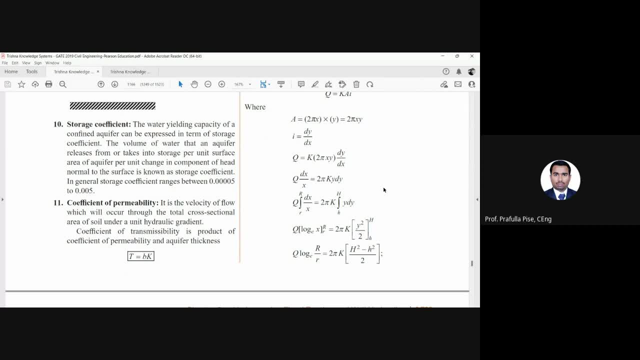 times d, y over dx, so q dx over dw lo города areaying area x. 그러면 you can think about the vertical distance in this吨ow area and horizontal distance as x, vertical, y, horizontalľ of times dx you can think of, it will minimize the x, vertical, y or dx in form of the horizontal. 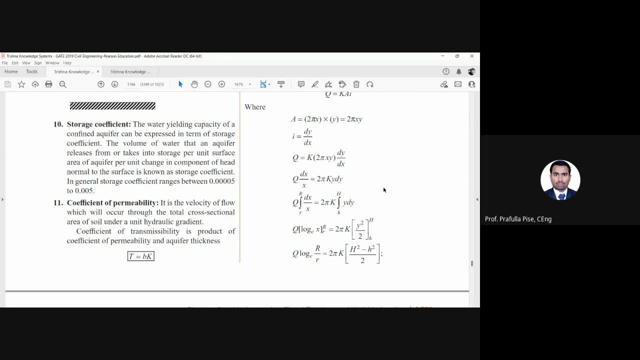 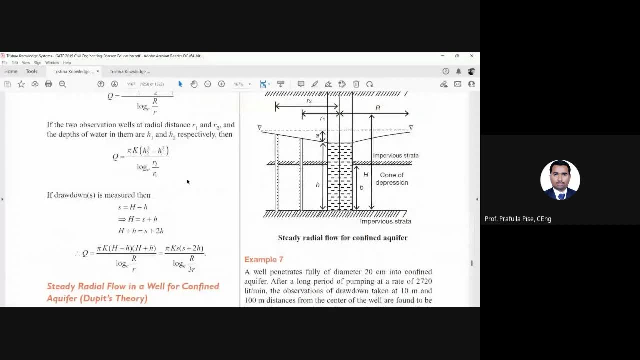 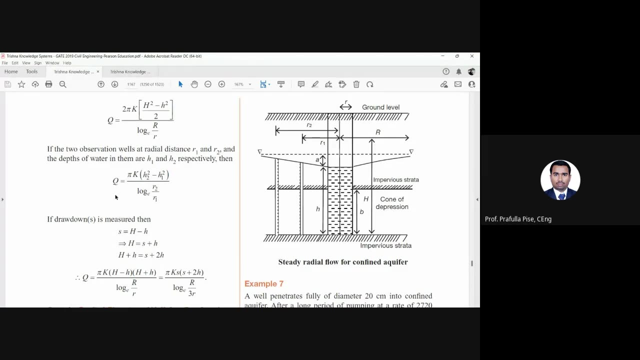 dx over x equals to 2 pi ky dy. okay, i don't think you need to remember the derivation of this equation. okay, at the end, this is the equation you are going to use, okay, which is: q equals to 2 pi k times h2 square minus h1 square, or log e. log is mean natural log r2 minus r1. okay, 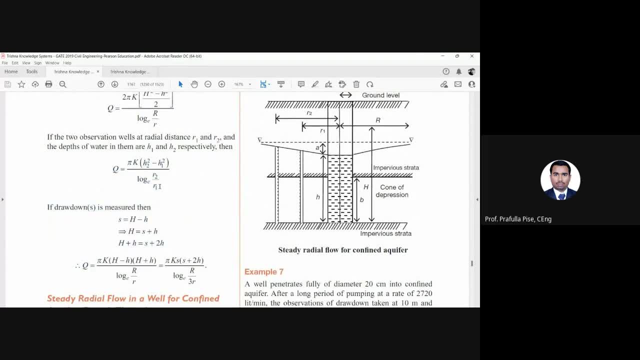 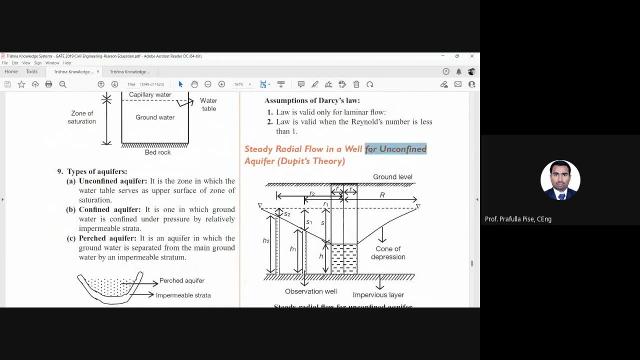 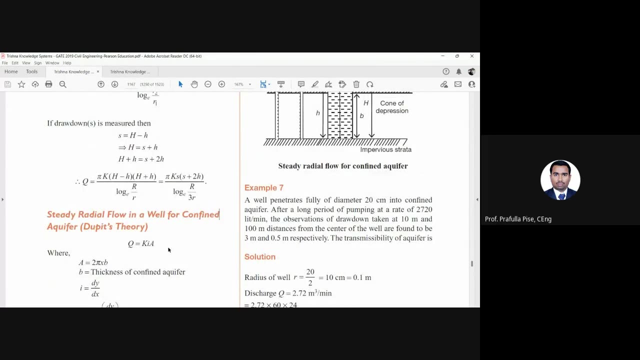 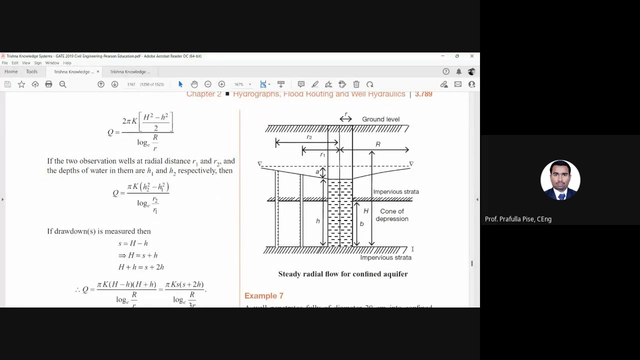 okay. so this is the equation you are going to remember for steady radial flow in a well, for unconfined aquifer. and if we find the steady radial flow for confined aquifer, so in confined aquifer we just have to add b. okay, why? because we have impervious layer. okay, this is aquifer. and then we again have impervious data. okay, 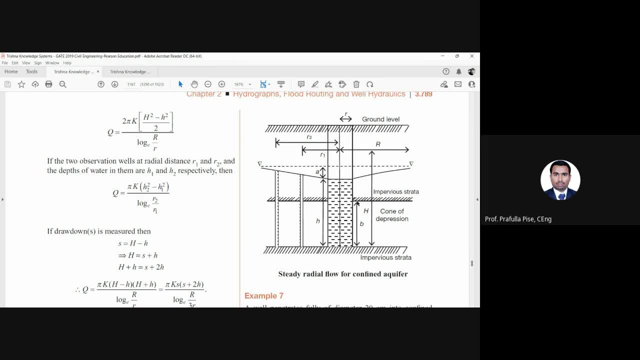 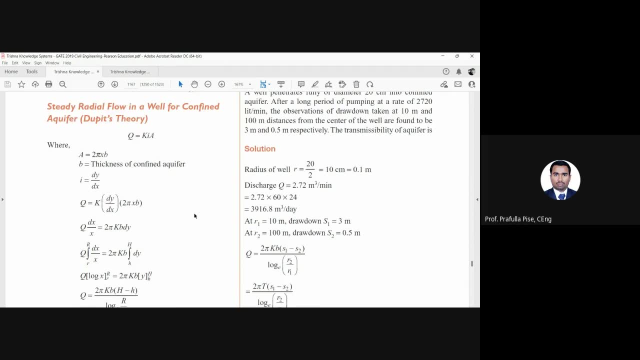 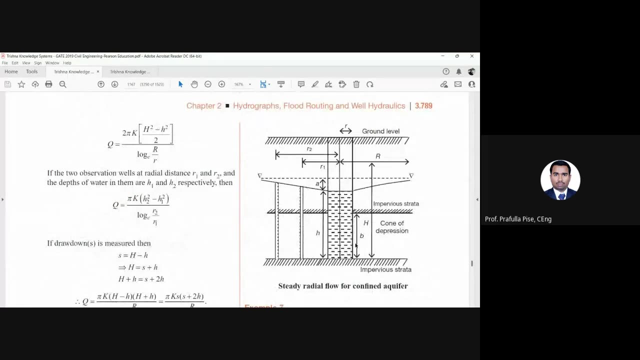 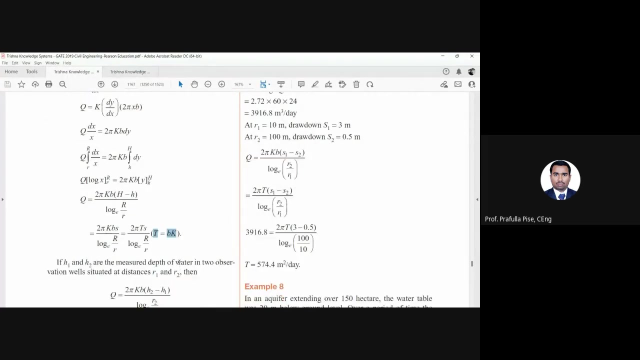 so we just have to add b. okay, so that is added in the diagram, but in formula we are going to subtract that b or account we have. we are going to be accounted for at b using the formula. where the formula t equals to b k. okay, you can use t equals. 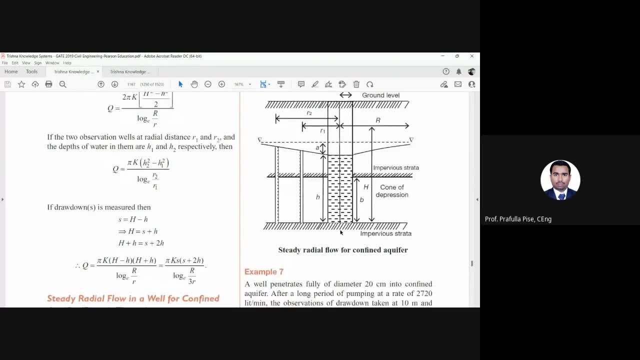 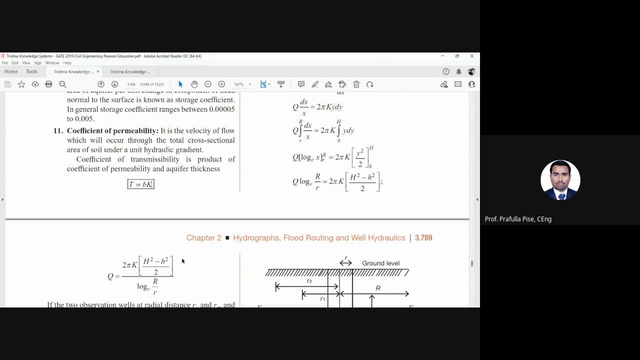 to b. k. b is the depth, or the depth of that Tran shapes. okay, so this b player, we're going to add depth or thickness of the aquifer times. k, yeah, okay. so k is the coefficient of permeability. okay, so coefficient of transferability equals to coefficient of permeability, k times the. 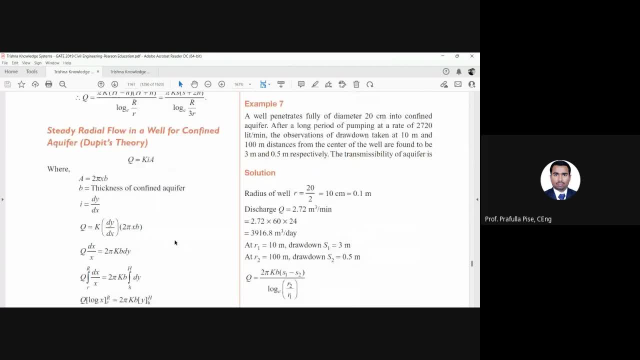 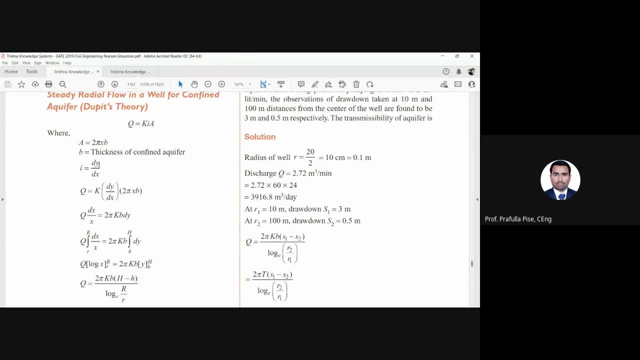 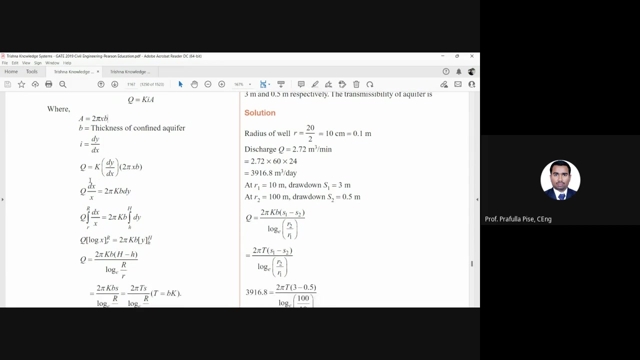 aquifer. thickness b. that is what we are going to use. again, the basic formula is same: q equals to kia. okay, now here, when we find an area. so again, 2 pi x is the same, but instead of y we are going to have b. okay, that's the thickness of confined aquifer. okay, same again, same derivation, but at: 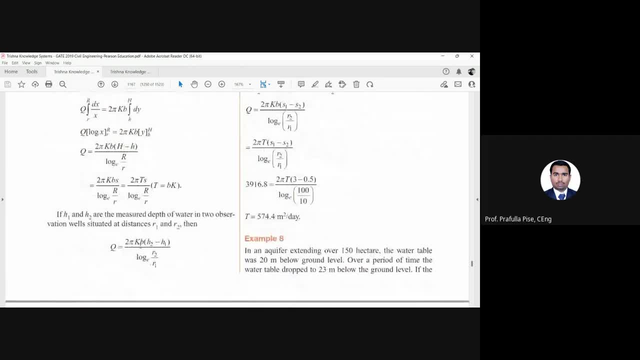 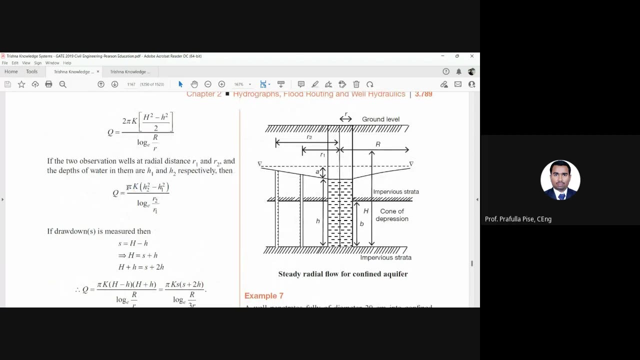 the end we'll get equation q equals to 2 pi kb. h2 minus h1, log e r2 over r1. so you just pay attention, we have b here, we don't have b here. okay, so pi k h2 square minus h1 square over log e r2 minus r2 over r1. 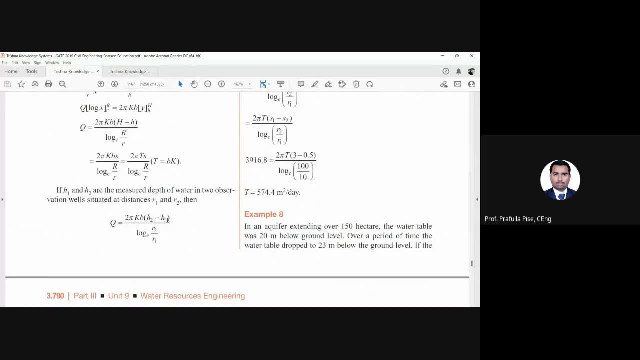 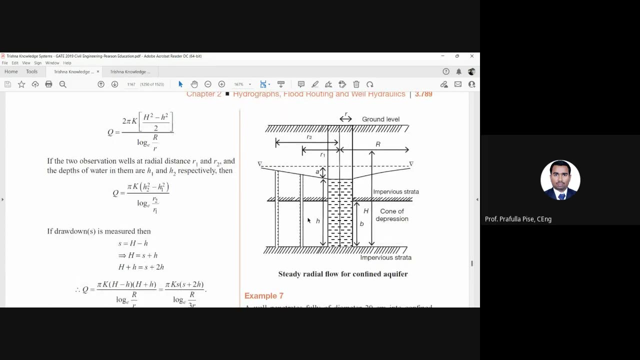 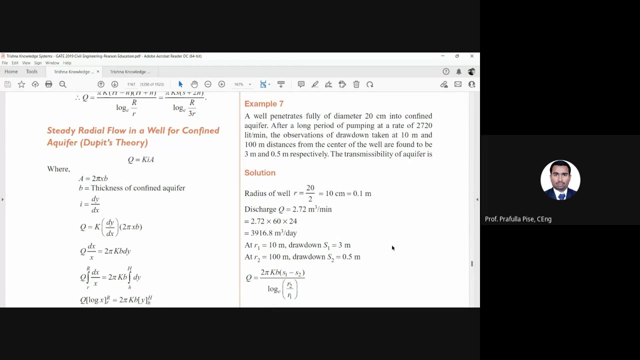 so same thing. pi k, h2 minus h1, log e, r2 over r1 and 2 b is extra. okay, 2 times b is extra here. so similar formula. but we have the thickness of aquifer, so let's try to solve an example. a well, penetrates fully of diameter 20. 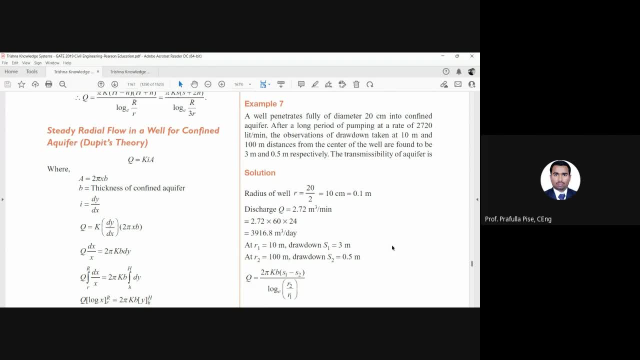 centimeter into confined aquifer. confined, okay, so we know this complaint, so we are going to use the formula with b. after a long period of pumping at a rate of 20- 2720 liter per minute, the observation of draw down at 10 meter and 100 meter distances from the center of the well are found to be 3 meter. 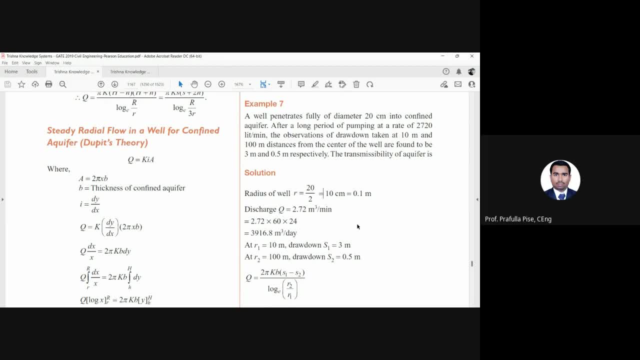 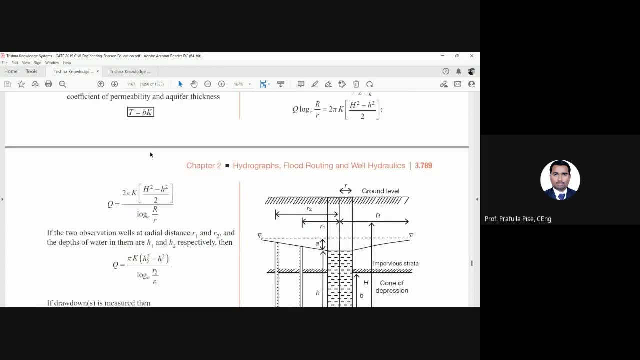 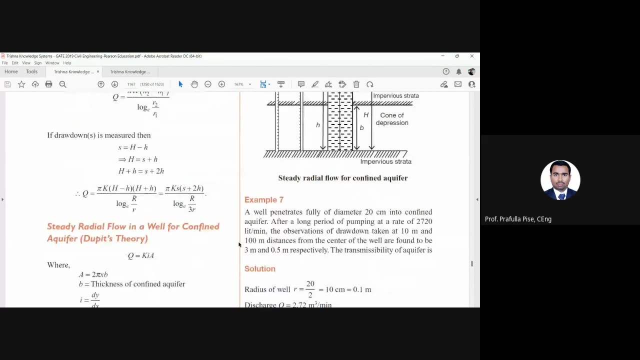 and 0.5 meter respectively. The transmissibility of aquifer is. so we are going to find out the transmissibility of aquifer, which is T. that is what we are trying to find out. T, okay, the B and K that we are going to already know from the formula. okay, So radius of well, they. 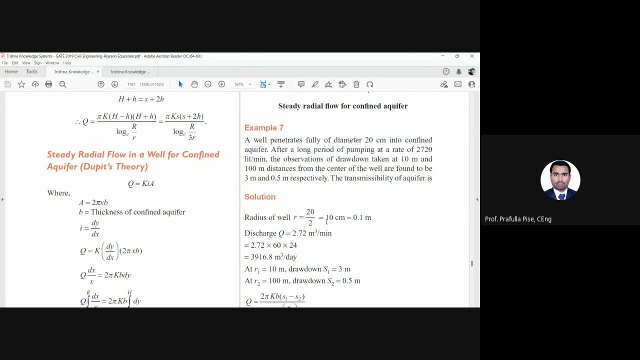 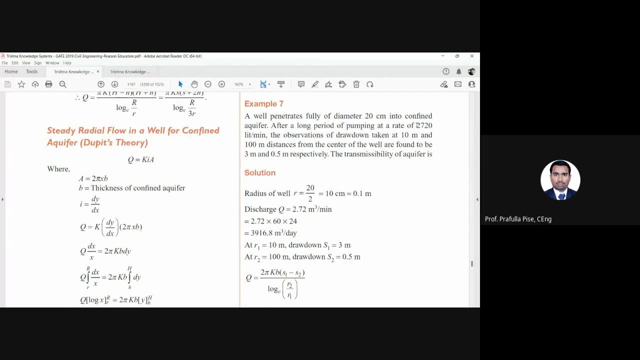 say diameter of 20 centimeter. so that's why radius of well will be 10 centimeters. so the meter 0.1 discharge, so they have 2720, okay, liter per minute. so if you convert that liter per minute to meter cube per minute, 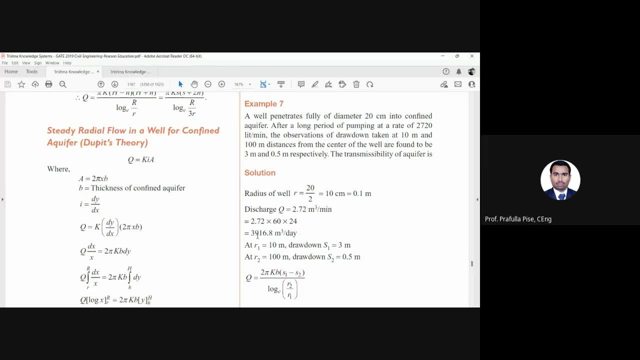 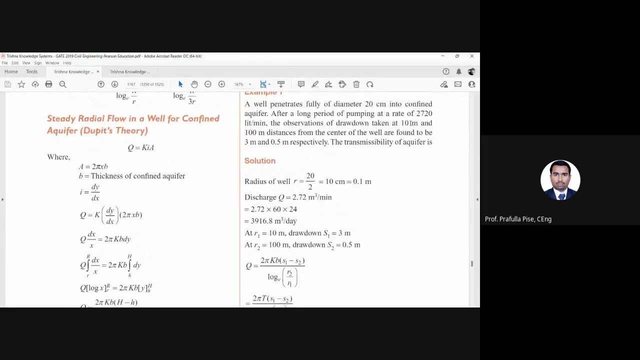 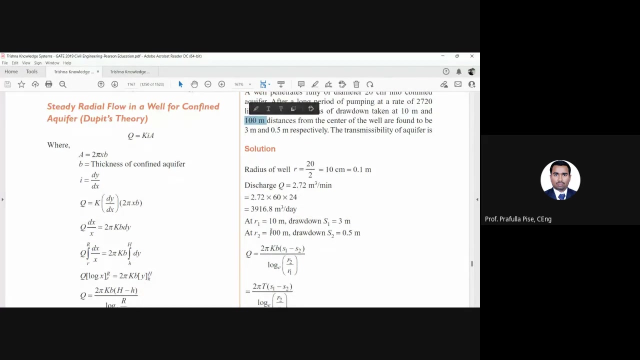 So 2.. 72 meter cube per minute. so basically 3916.8 meter cube per day, so 60 minutes, 24 hours. Now R1, we know 10 meter because they say first or two observation draw down taken, which is that one is 10 meter and one is 100 meter. so R1 is 10 meter, R2 is 100 meter. For S1 they have say: 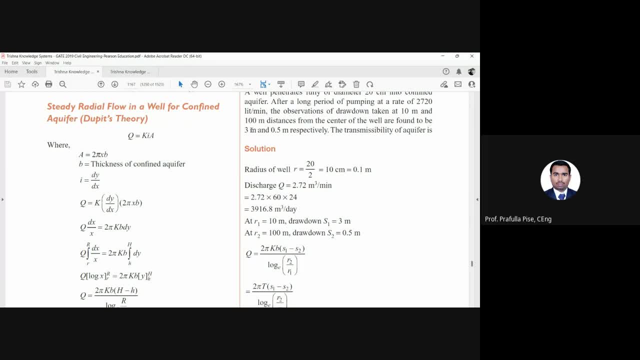 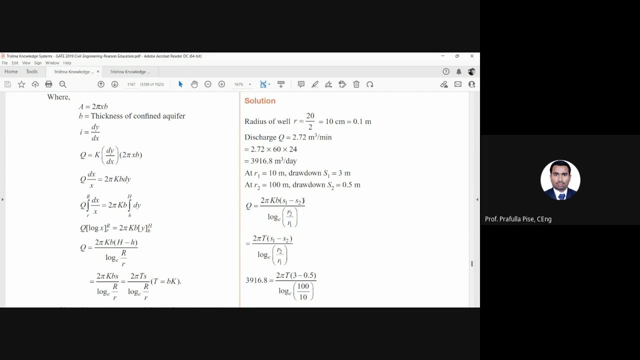 value is the well are found to be 3 meter and 0.5 meter, so S1 is 3 meter, S2 is 0.5 meter. Using the formula q equals to 2 Pi KB, S1 minus S2 or h1 minus S2 over log of R2, R2 over R1. 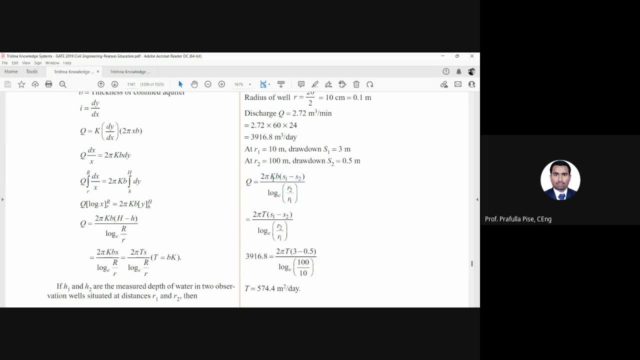 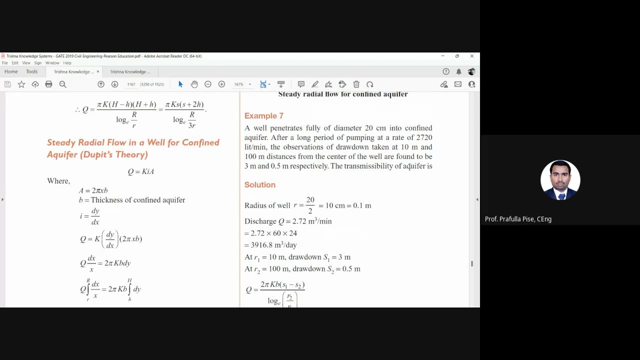 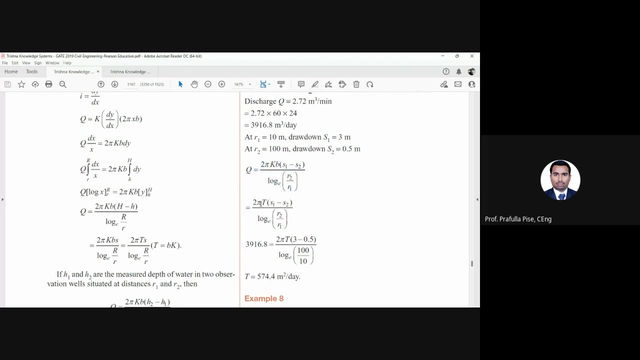 So 2 Pi, Now KB. okay, we can write kb as t. okay, because we are interested in finding out t uh, then k. okay, because that's what they ask: transparency of impact before we are trying to figure out the t. that's why we replace kb. we replace kb with t uh. s1 minus s2. love of r2 over r1. 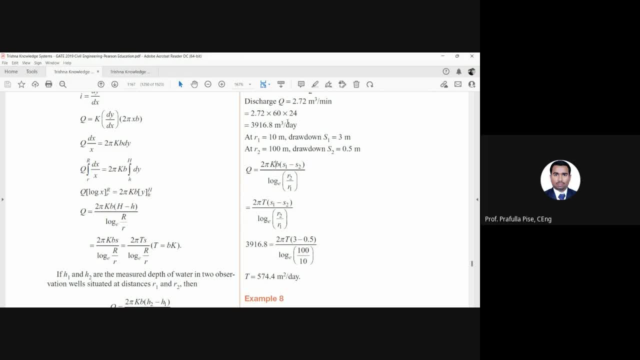 q. we already figured out q. 3960.8, 2 pi t, 3 minus 0.5, 3 minus 0.5 log of 100 over 10.. so we already know pi, we know 2, we can figure out the t. so that's the, that's the. 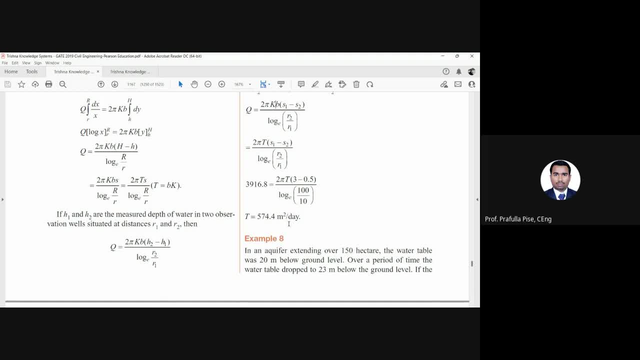 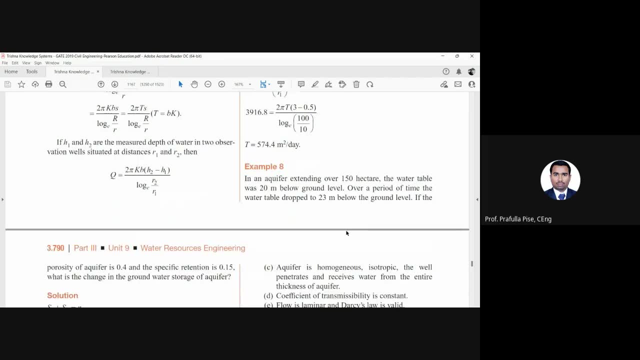 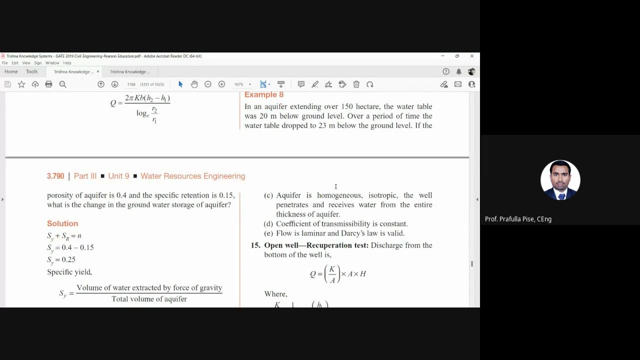 solution for t, which is 574.4 meter square per day. now let's see the next problem. in an aquifer extending over 150 hectare, the water table has 20 meter below one ground level. over a period of time, the water table dropped to 23 meter below the ground water. 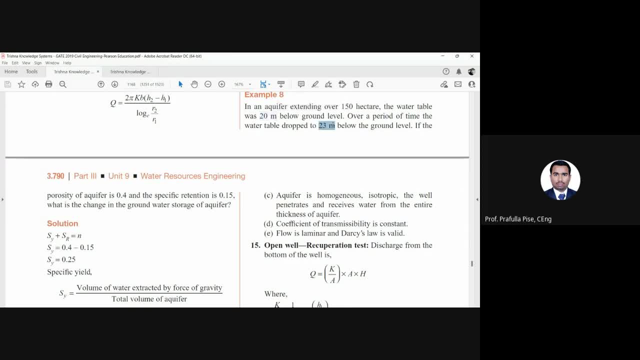 ground level. so see, before it was 20 meter, now it is 23, so 3 meter. okay, if the positive aquifer is 0.4 and the specific rotation is 0.15, what is the change? in groundwater storage of a paper? so we know, porosity: n equals to sy plus sr. okay, yield and retention, so sy equals to 0.4. 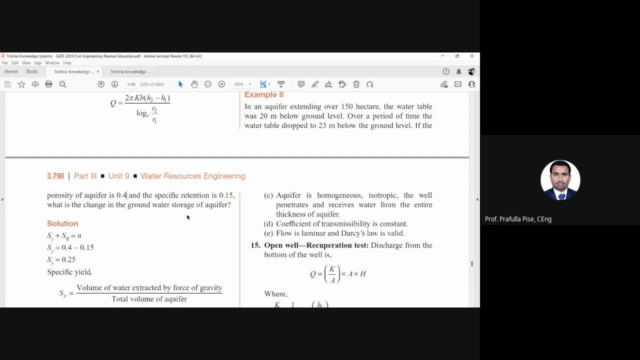 with 0.4, 0.4, okay, minus 0.15, and uh, because if we rearrange this equation, n is 0.4 and s r retention is 0.15, so we got sy equals 0.25. the specific yield equals the volume of water extracted by force of gravity. 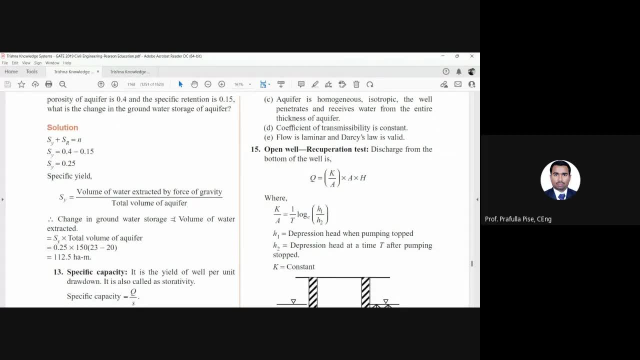 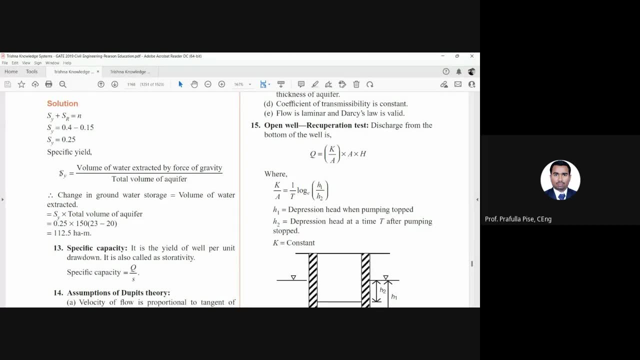 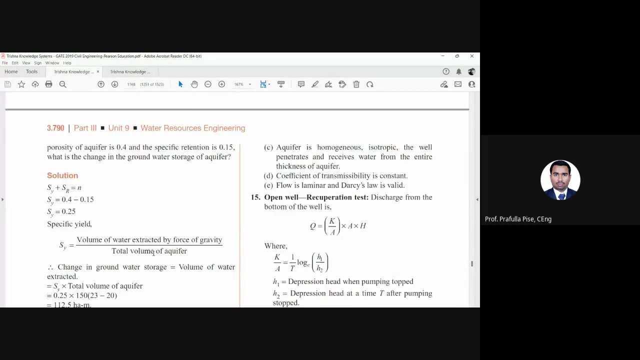 divided by total volume of aquifer, the change in ground water storage equal to volume of water extracted, so sy times total volume of aquifer. so that's why we are in figure out 0.25 total volume of aquifer is nothing but what we have, 150 hectares times the difference. so which is? 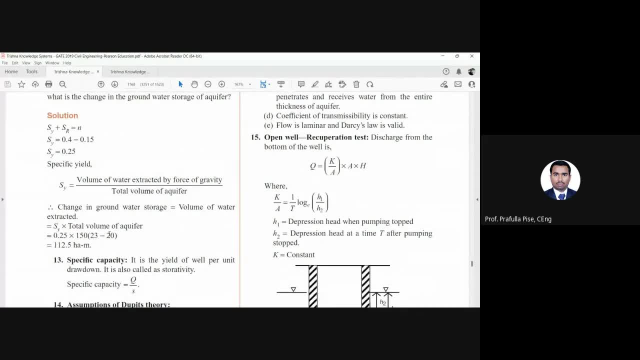 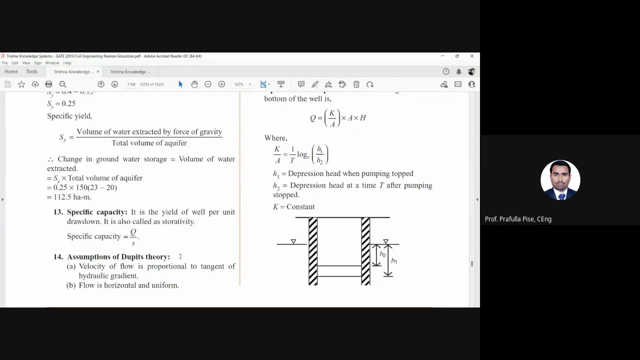 23 minus 2 area, times depth, okay, and times sy, that will give us a groundwater storage which is 112.5 hectare meter specific capacity. it is the yield of well per unit drawn- pardon. it is also called as storativity. space with cavity equals to uh, q or s. now there are assumptions of dupitz theory. 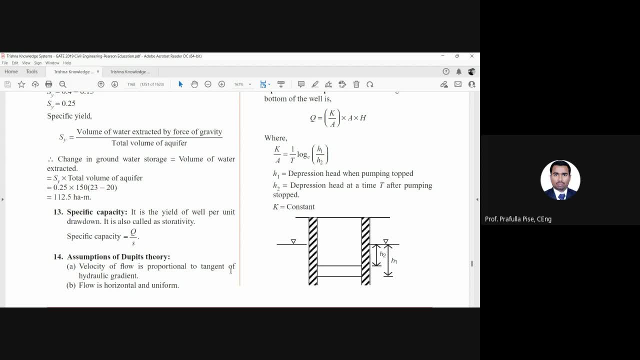 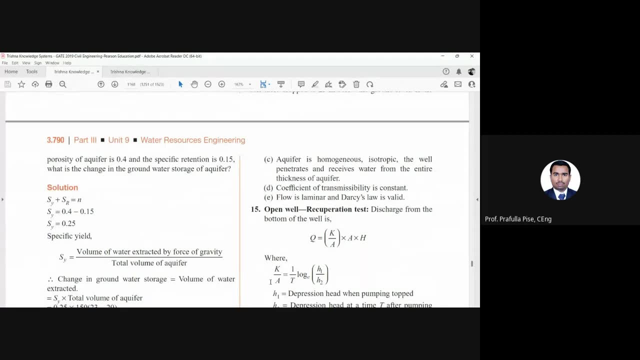 the wellster flow is proportional to the tangent of hydraulic gradient. flow is horizontal and uniform, which is more likely. aquifer is homogeneous, isotropic, and the well penetrates and receives water from the entire thickness of aquifer. coefficient of transmissibility is constant. flow is laminar and follows the darcy's law. 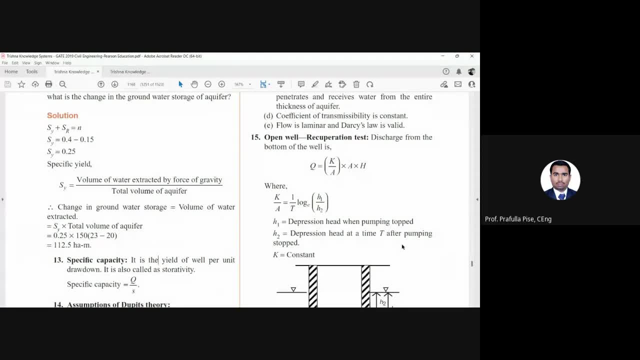 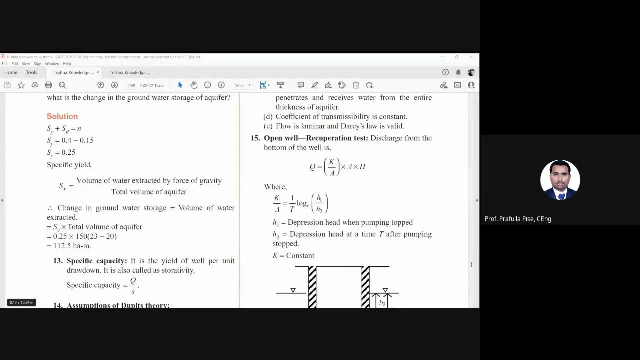 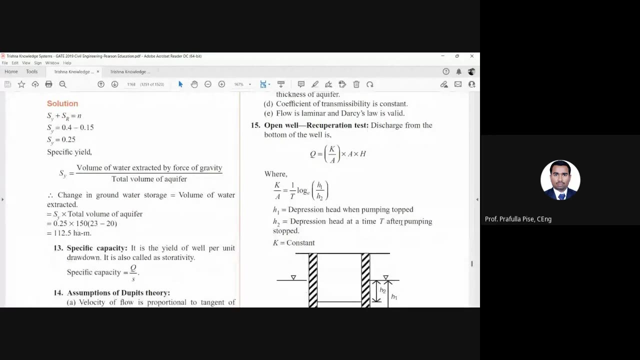 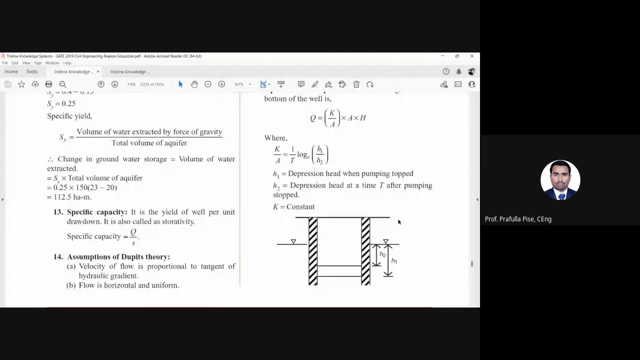 now open. well recuperation test. open. well recuperation test. q equals to k over a times a times h, where k over a is nothing but equal to 1 over t. log of h1 over h2. so h1 is depression head when pumping stopped and h2 is depression head at the time t after pumping stopped. k is a constant. 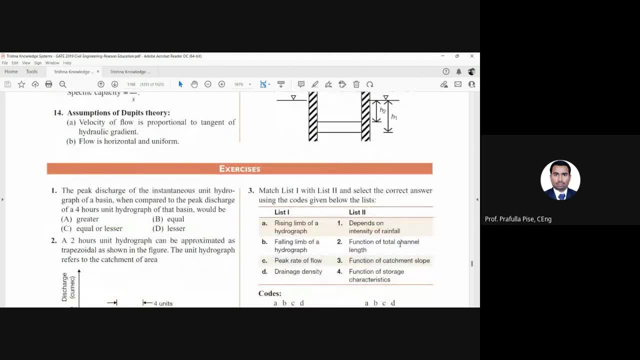 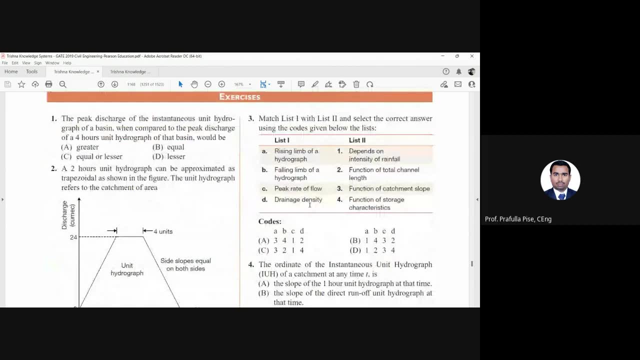 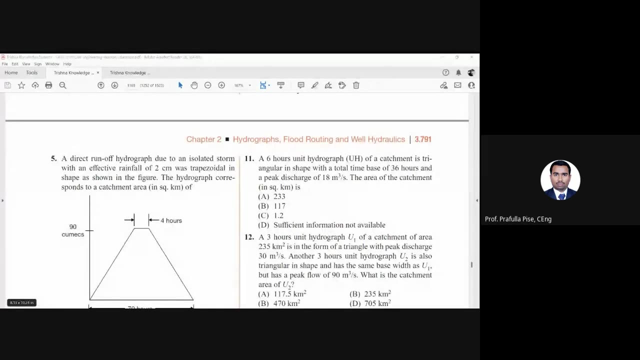 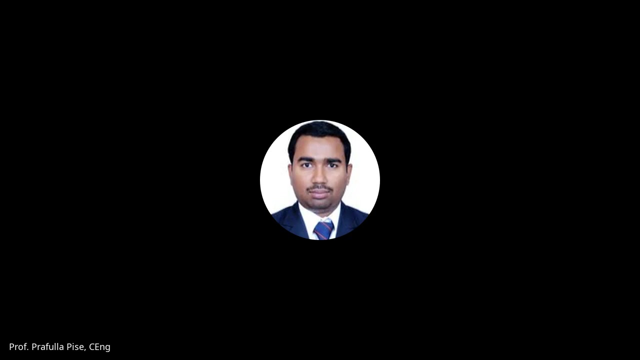 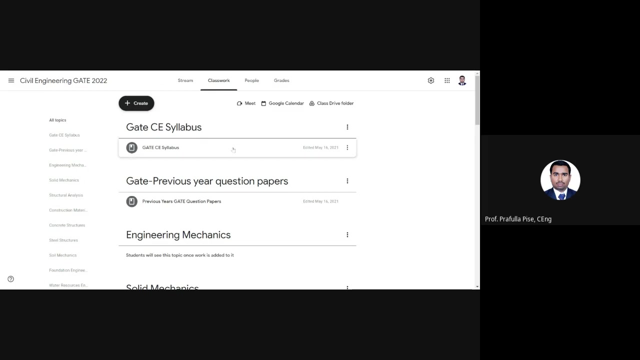 okay, so that's done with the well, hydraulics and these are some problems. okay, now i don't know how many of you joined the google classroom of get 2022. can you see PRESIDENTIAL after dot? excuse me, get 22 2002. 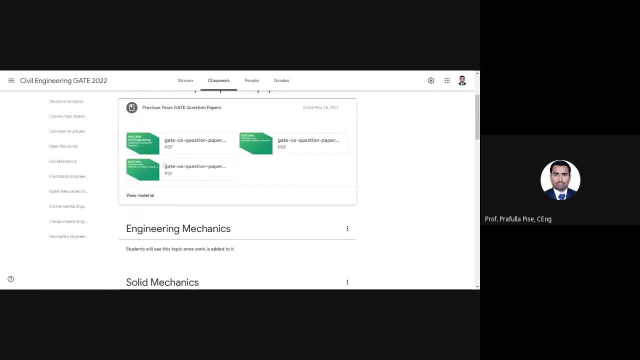 so under the classroom you will see there are previous years question paper. okay, so 2018, 2019 question papers. okay then. if you go down t lot of questions, 12stick so requests, then if you write the question paper, then you can take right down all the questions- nothing, okay. if you go till the unanalyze: okay. if you go down ahietetetetetet is where they are all contents- okay then. if so, if you product laughed at home plat bugün, ignited questions aboutpla, then what we will use? cakie a. 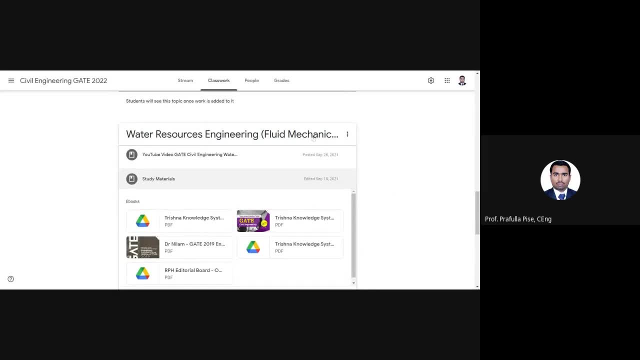 study material. what was engineering fluid mechanics? okay, this one, so you can go study matter. you will find there are books. okay, uh, okay. okay, so this one. okay. so do you see? this is um civil engineering. previous years solved question papers. okay, question paper. this is uh, what is? this is the topic was practice test. 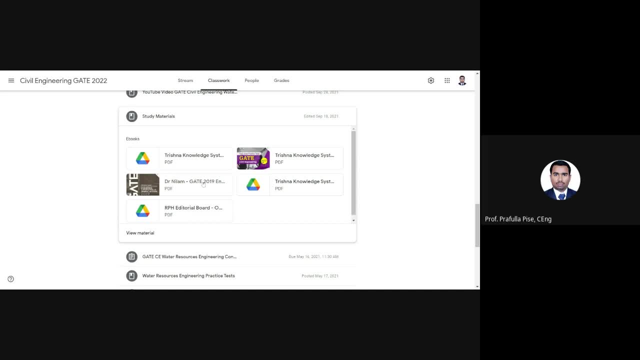 this is the get book. uh, this is the mathematics and general attitude previous year's solved paper and these are the objective question for the civil engineering. okay, it is also uploaded here in the google classroom, okay, any further question? doubt guy question. no, sir, i'm going to share the youtube link for today's session on your google classroom. okay, so you can.